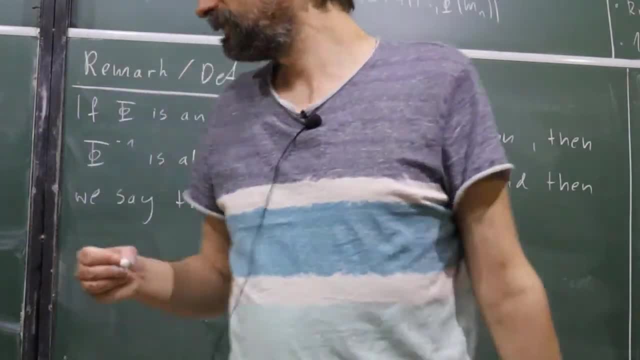 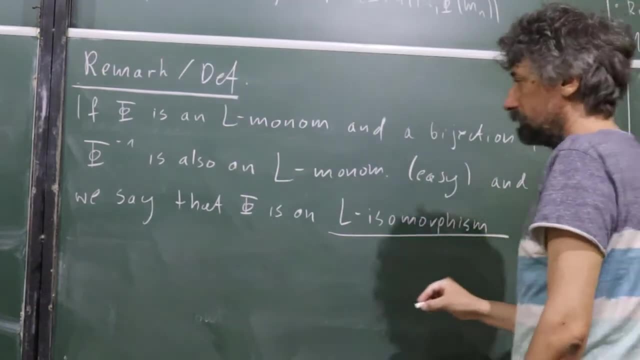 isomorphism of groups or rings. then we kind of say: what is this L denoted? What did you give to the definition of monomorphism? Yes, I was trying to say, to be honest, I don't know. I don't know the definition To. 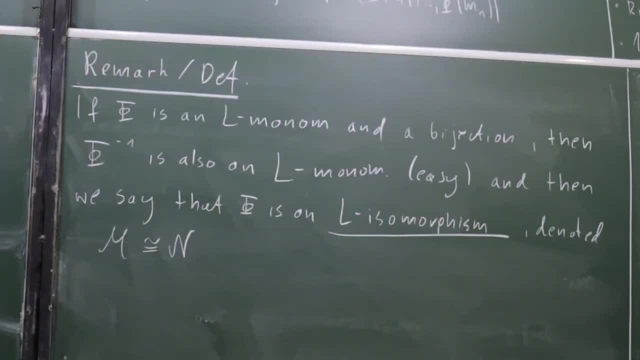 be honest, I don't know the definition. What is the definition of monomorphism? Yes, I was trying to say, to be honest, I don't know the definition of monomorphism. a good reason, but for relations it's pretty strange. 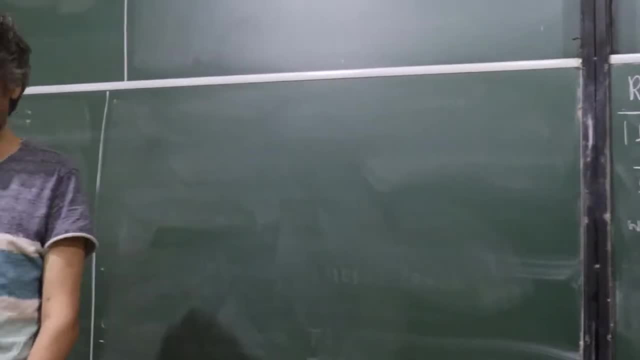 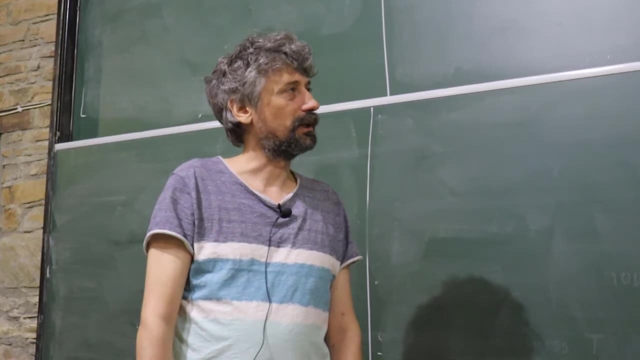 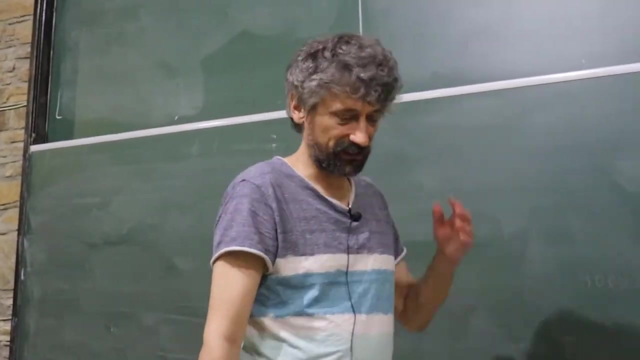 function is not one to one. that I think doesn't make much sense to say it's a homomorphism if we consider relations. but yes, somehow people don't define in this general context homomorphism. but I cannot say now what really breaks if you do. 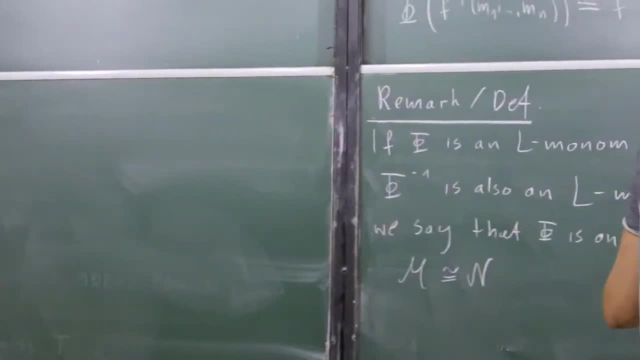 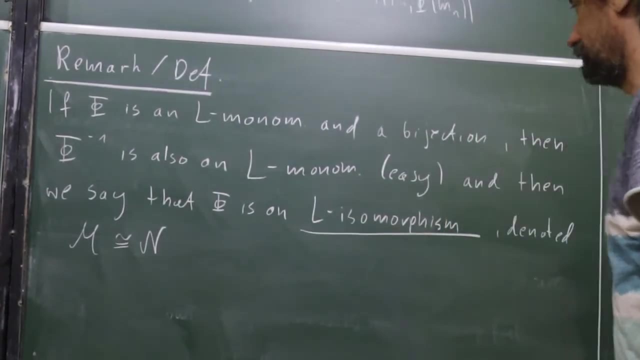 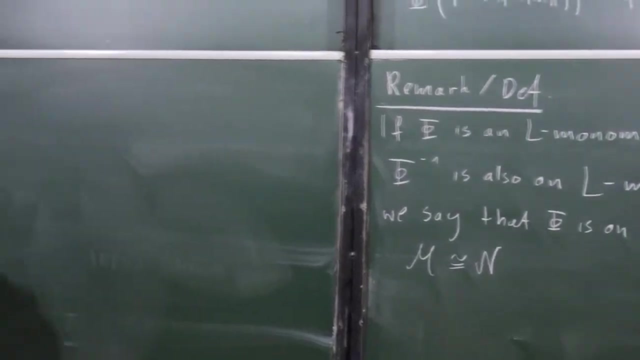 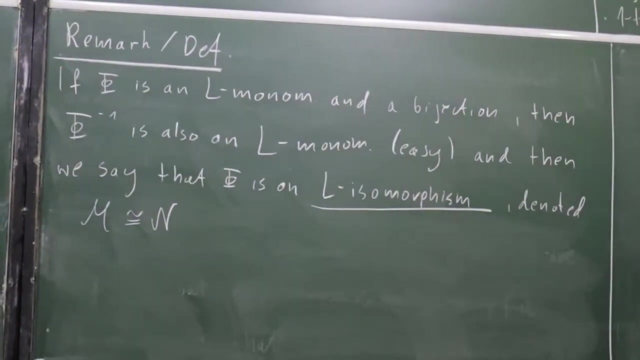 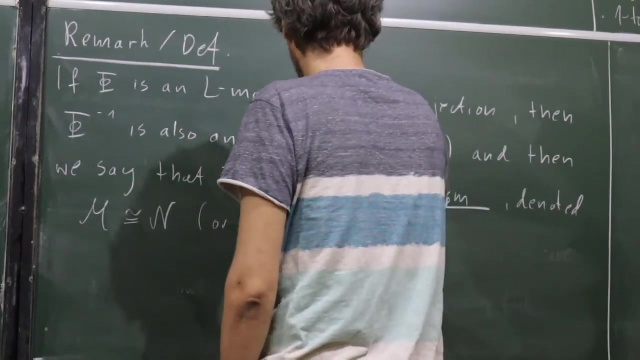 also. also, they are not very much useful in this generality because the most important notion will be of substructure and then some elementary extensions and it all is one to one there. so we will come to that or denote it like this: huh, so some lemma which will again not show. 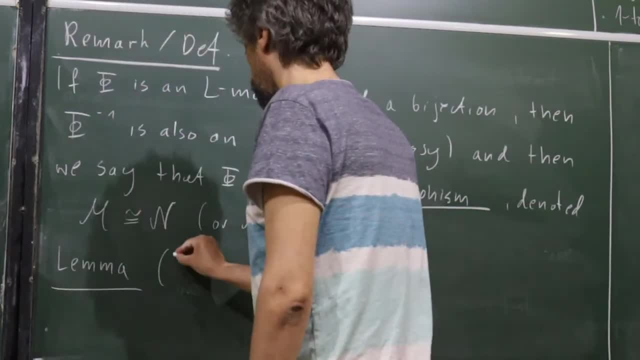 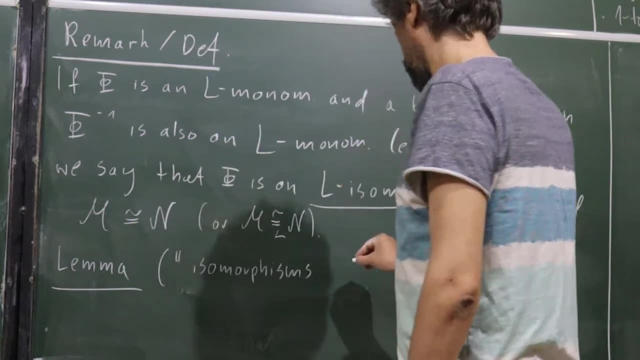 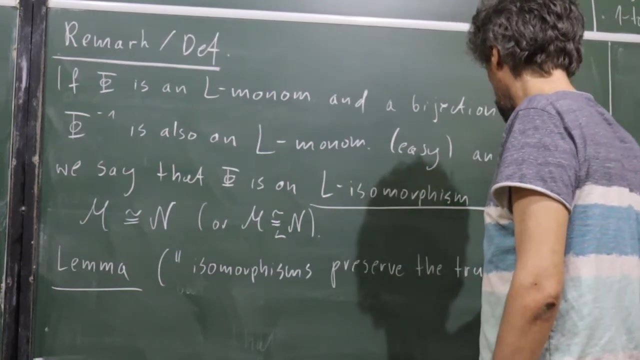 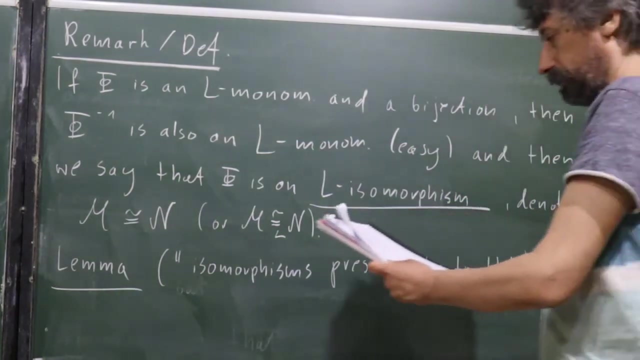 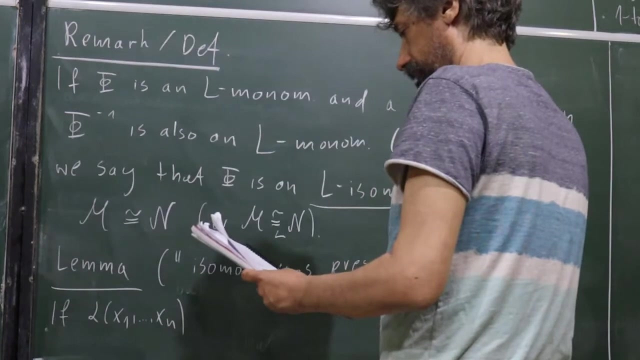 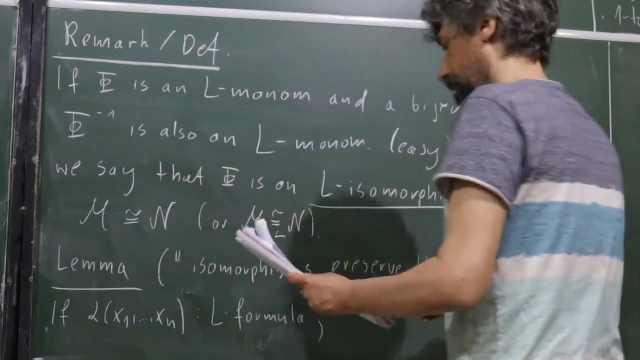 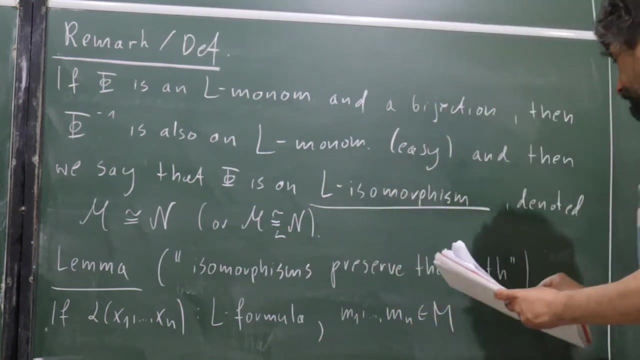 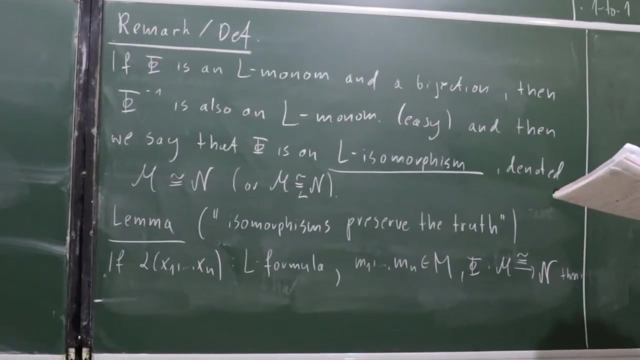 but often use. so short saying will be that isomorphisms preserve the truth. so formal statement is: if we have a formula with some three variables and elements in the first structure and let's see, is this isomorphism in this sense, then well then, it kind of preserves. 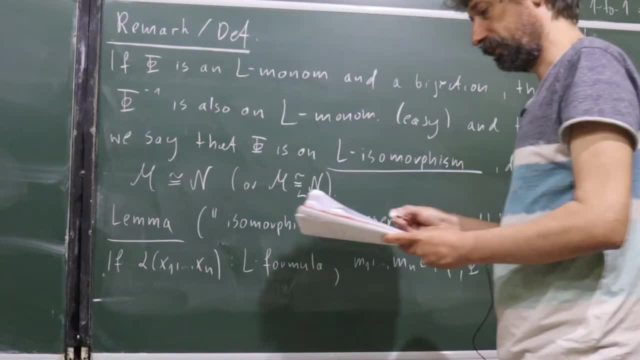 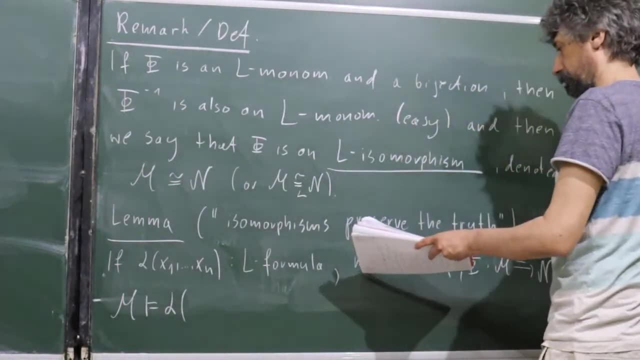 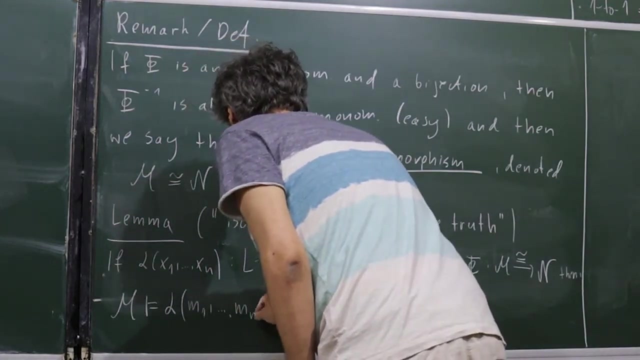 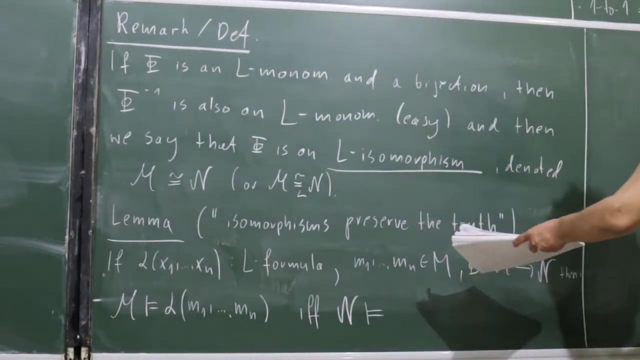 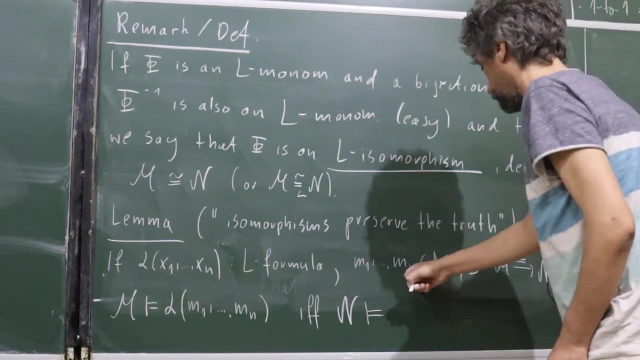 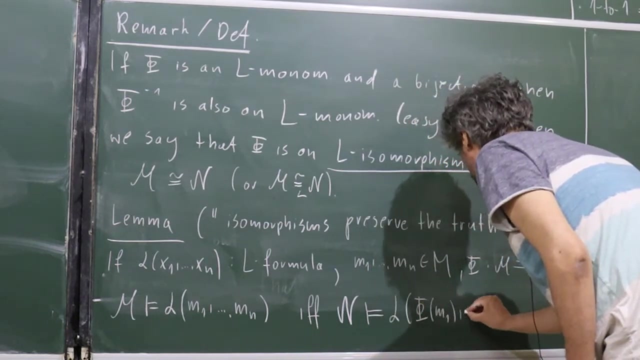 the satisfaction of this formula. so M, so alpha, after we plug M1, Mn for these three variables holds in M if, and only if, the same happens in N after the positive image at x is 1. so Alpha's, berm, Mudden's, we put Psi to this, to this, to these parameters. 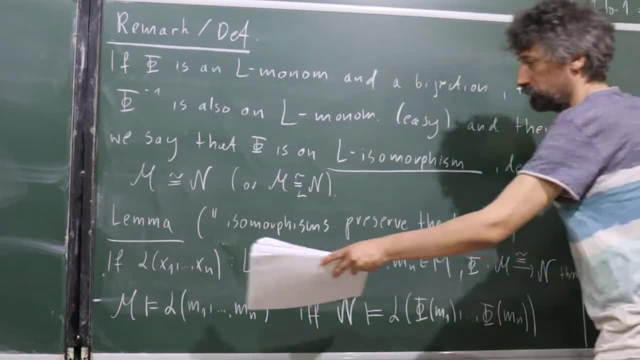 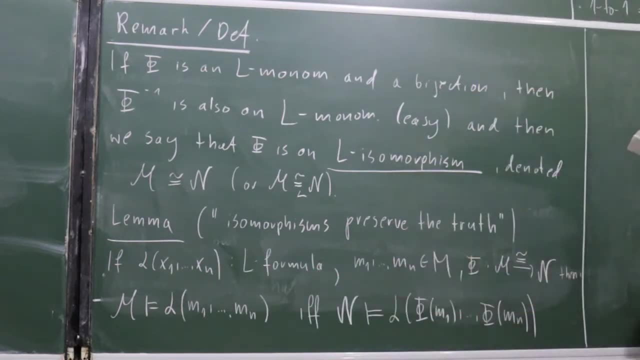 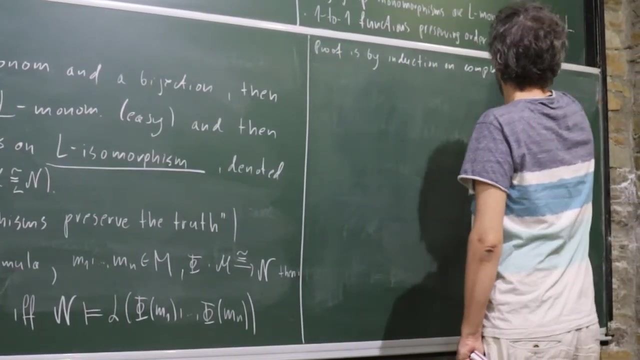 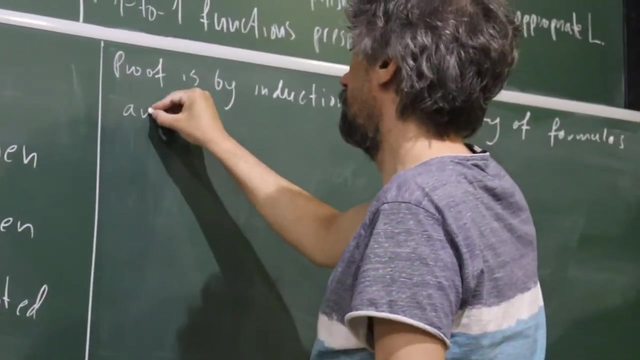 in particular, if this formula was a sentence, then it's true in M, if, and only if, it is true in N, because there is nothing to plug. so again, as many times before, so proof is by induction on complexity of formulas and we skip it. and and, and. 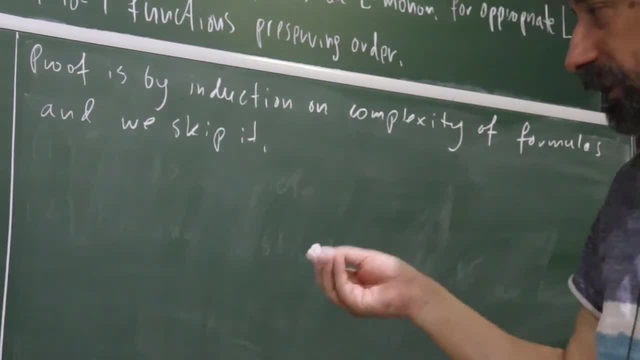 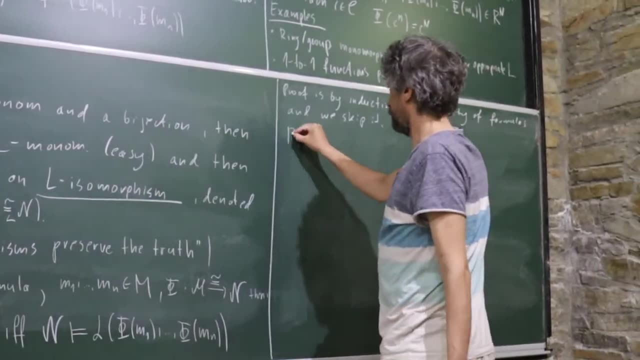 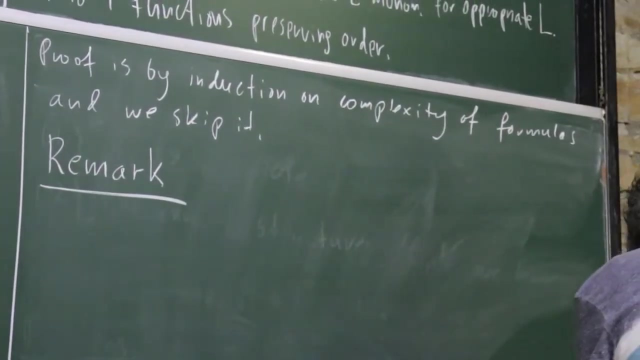 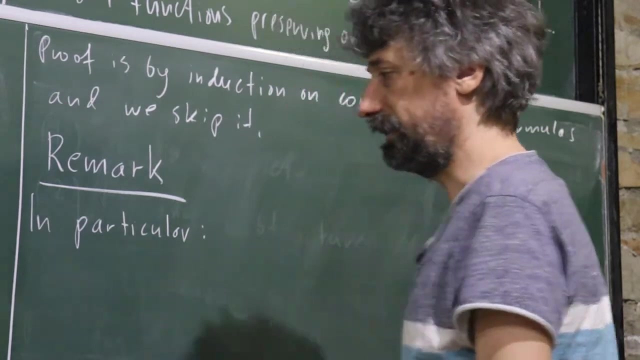 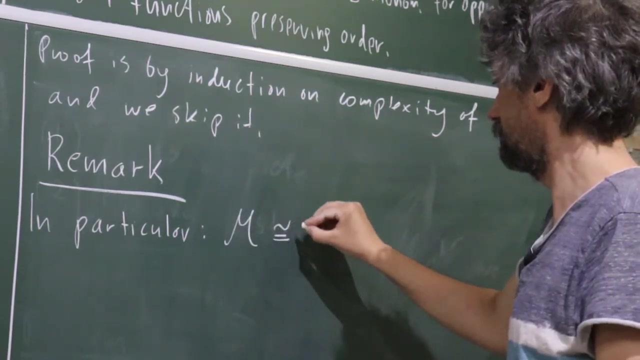 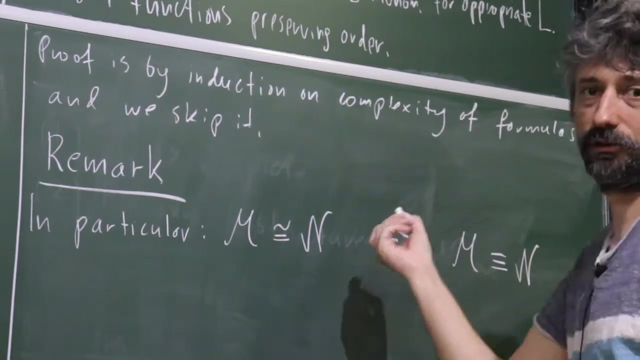 and and yes, we skip everything which actually requires the formal definition of formula, but remark which we kind of used already in problem session. so, in particular, what I exactly said: isomorphisms. isomorphism implies elementary equivalence. so, yeah, the truth, but this is much stronger. 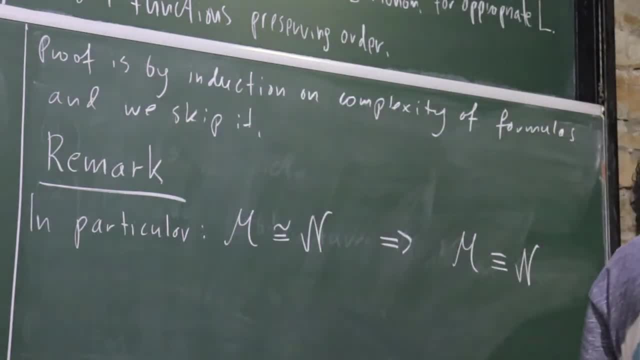 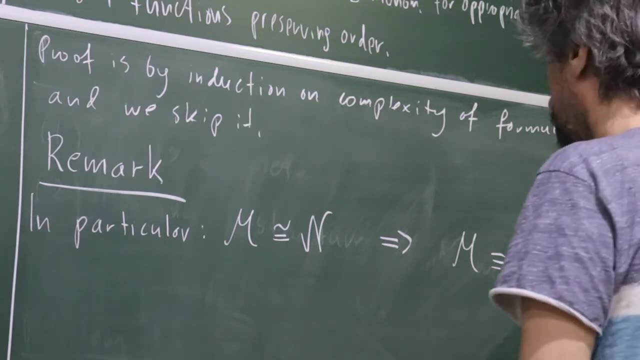 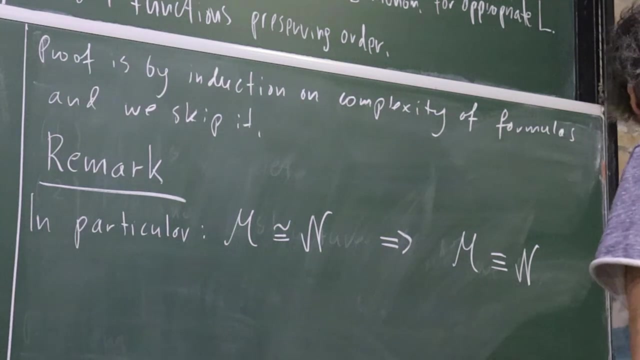 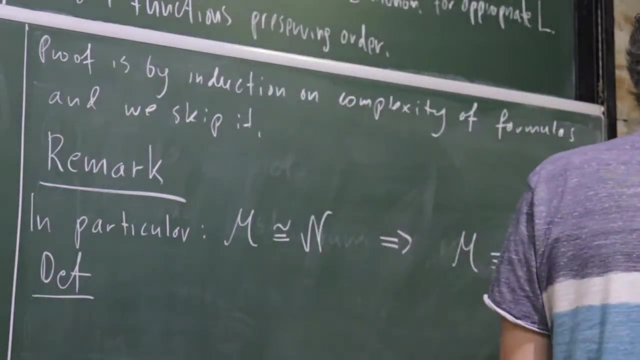 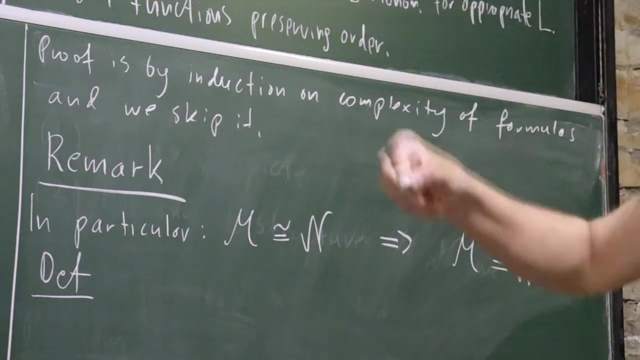 Okay, yes, it's not the same, but still, soon we will see example, so it's not the same. so, Finally, the notion which I was really aiming at may be quicker, but I also need that. so I really need that notion of isomorphism and of substructure, but this one contains both. 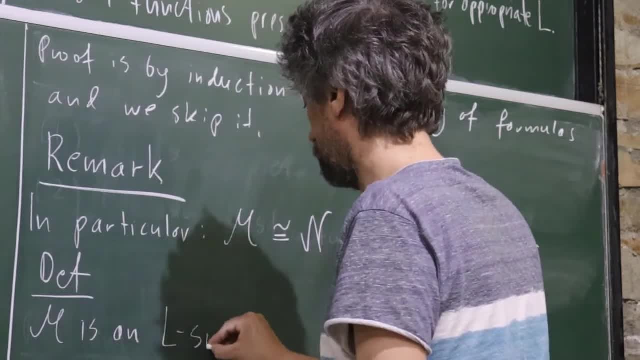 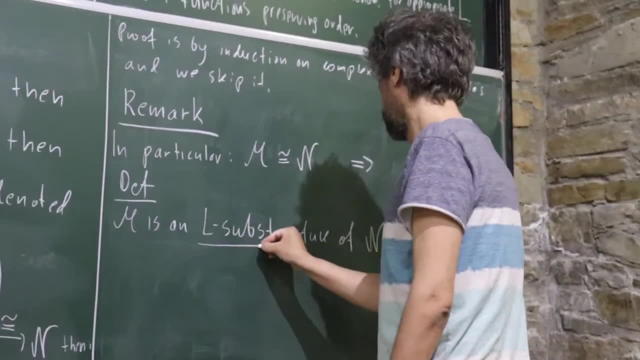 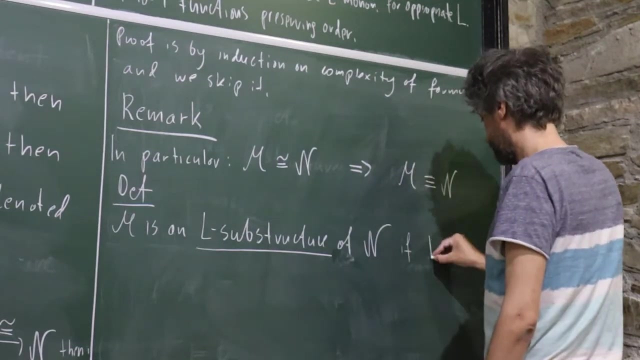 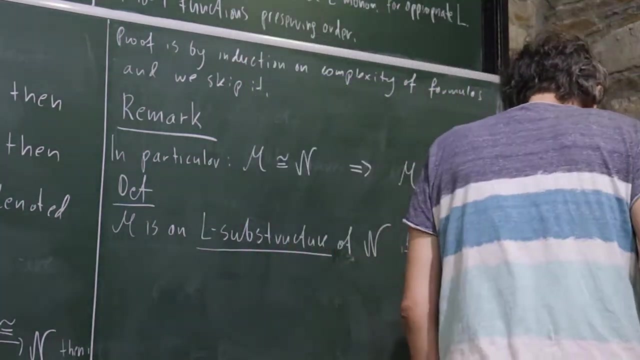 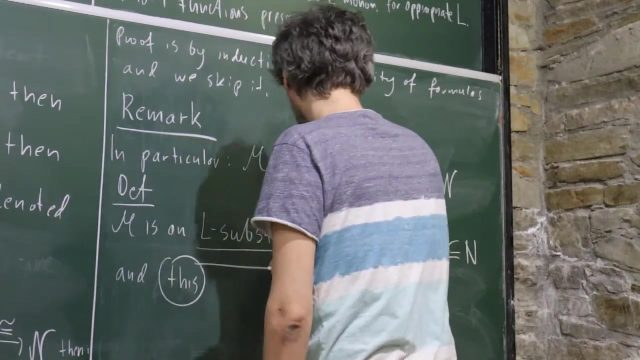 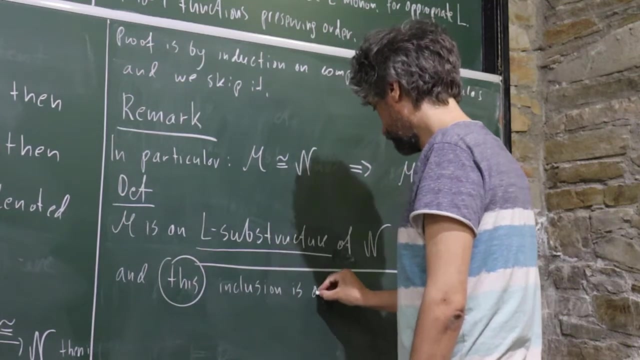 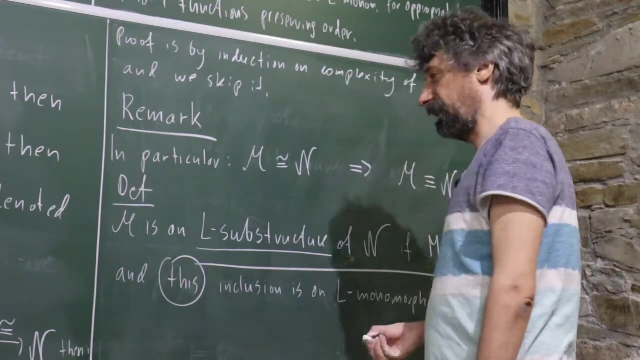 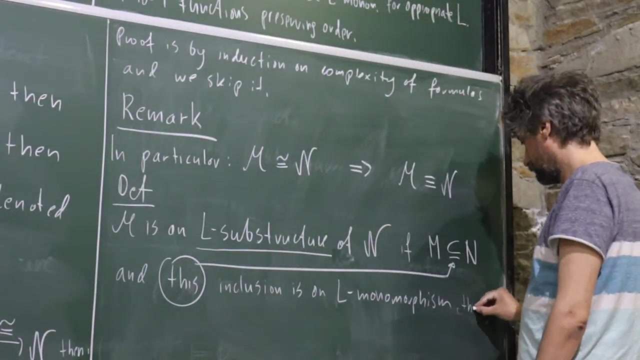 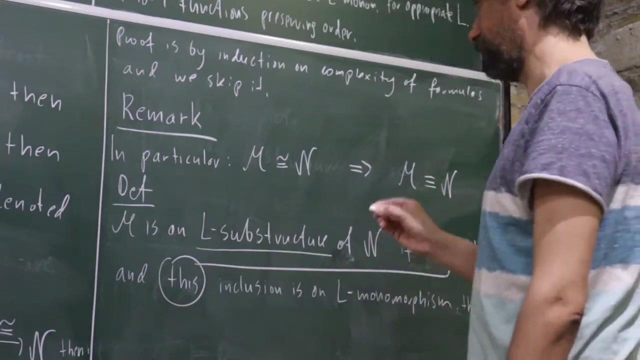 M is an L substructure of N, so of course, if universe is a subset of bigger universe and this inclusion is a monomorphism, so that's pretty formal. so let us write what this means. that is actually. it's a definition which in algebra i don't like. let me mention it later. that is: 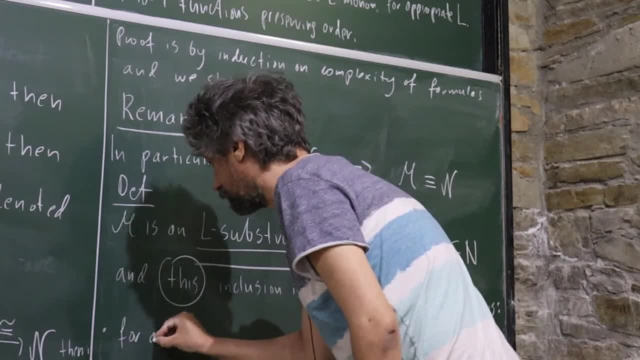 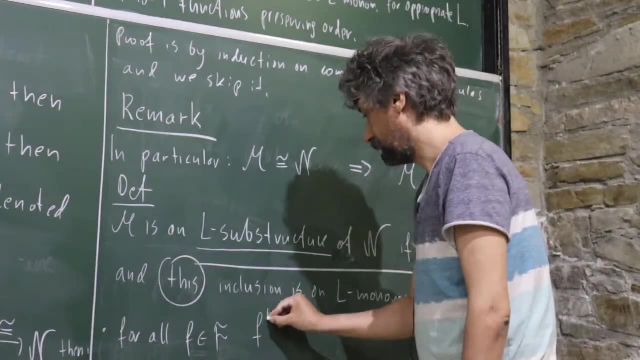 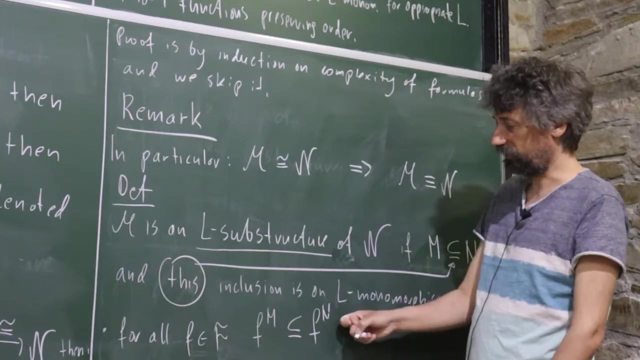 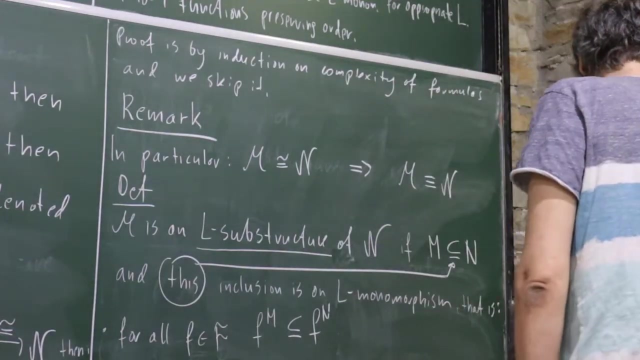 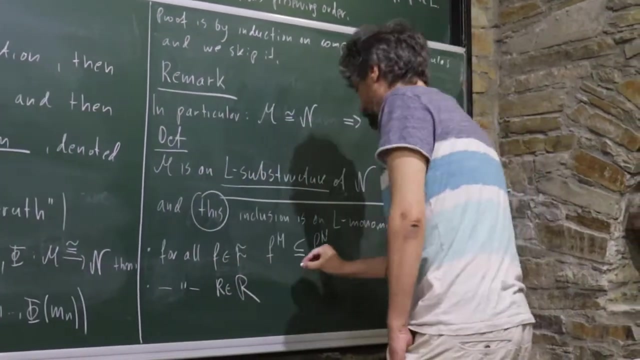 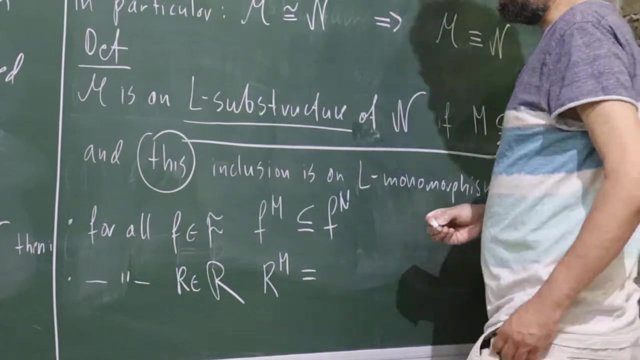 for all f in f instead of n connections and extends. okay, just notation means that of n restricted to power of m is fm, but formally it means that graph is contained in the graph for all r in r. that's the difference. kind of this is not a subset, not only a subset, but it's exactly. 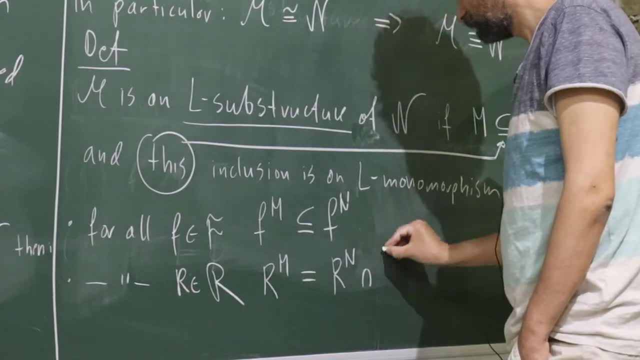 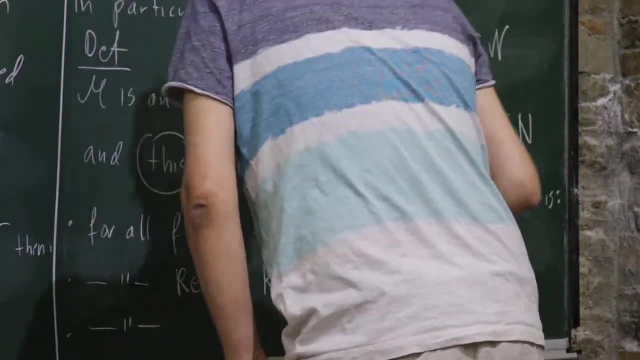 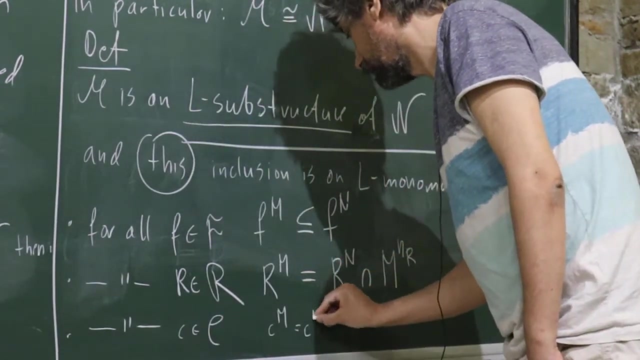 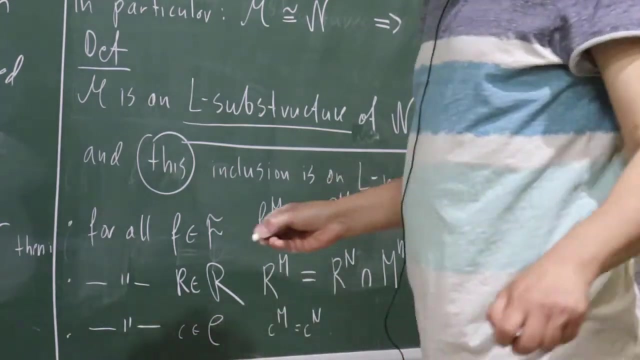 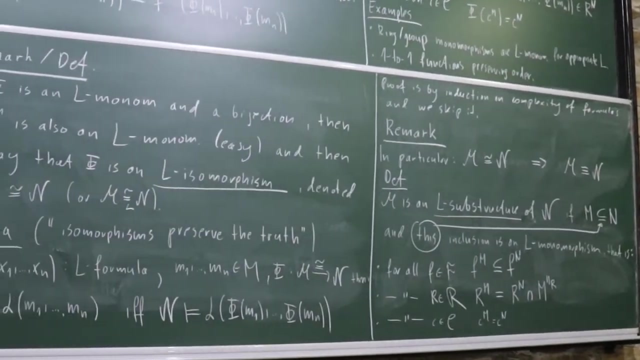 the intersection and, of course, for constants, it's just the same interpretation. so so this is the moment to answer the question of the guy who didn't come today. why did we call to our language the language of rings? to make sure that substructures are subrings, okay, so examples: 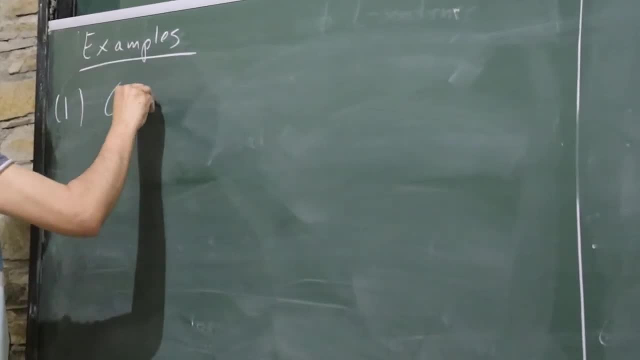 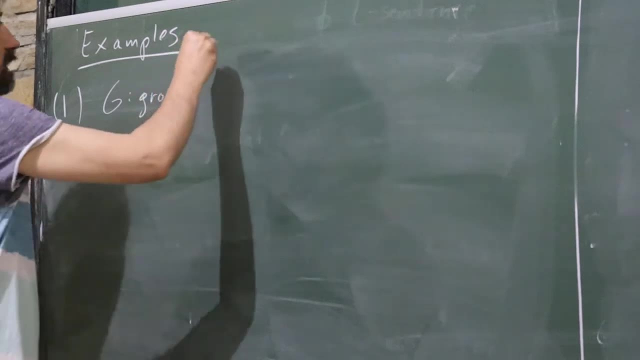 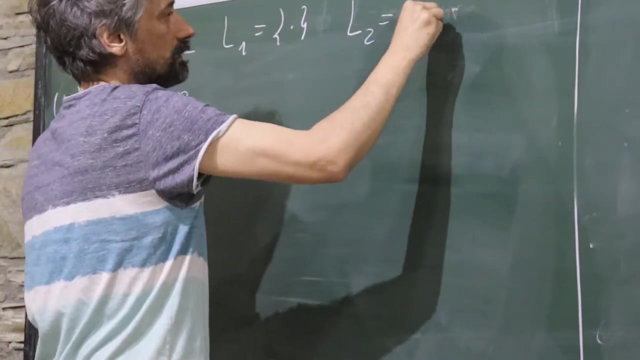 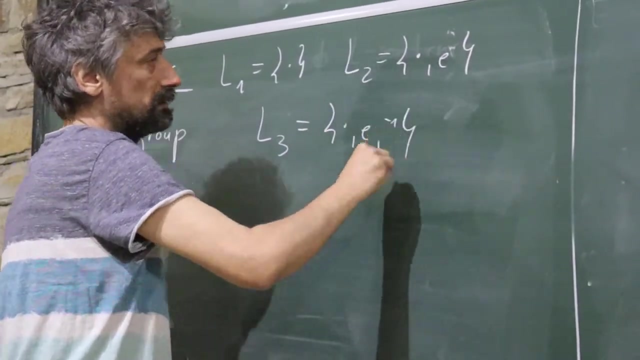 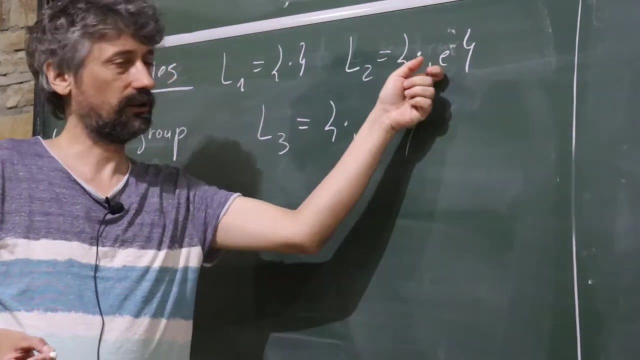 so if g is a group, okay, then we can regard it in at least three languages: g a group and l1 be this, okay. so this is just binary function for multiplication. this is also language with constant for neutral element and this also has unar function for inverse. 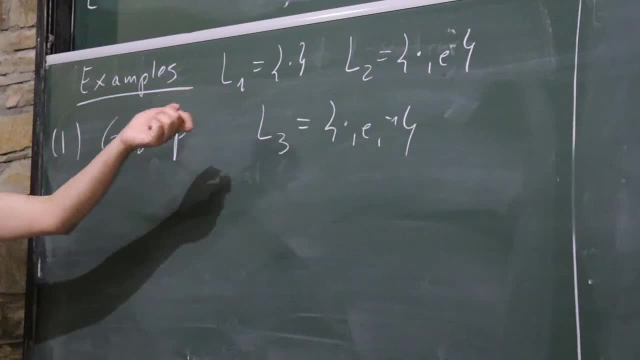 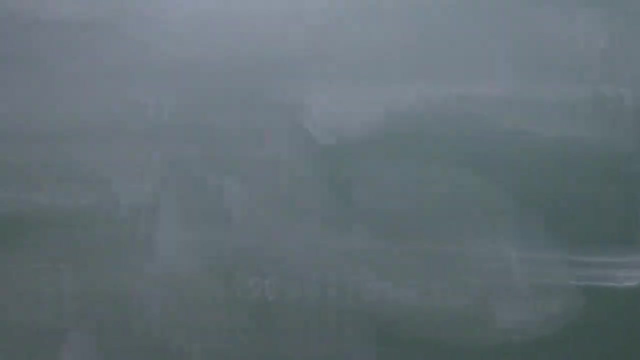 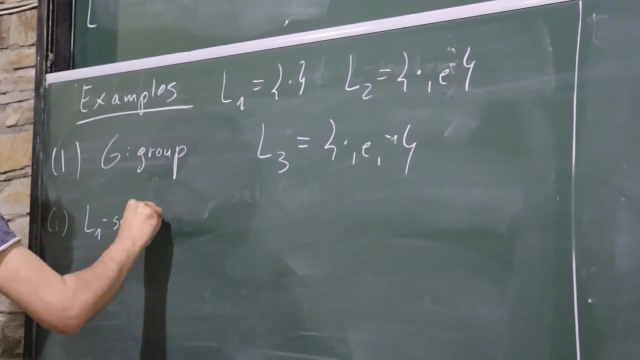 so all is kind of the same. g is a group in all of these languages, and if it is a group you can always define uniquely this and this. so not much difference. but the notion of substructure changes. so if you care about substructures, so here and l1- substructures. 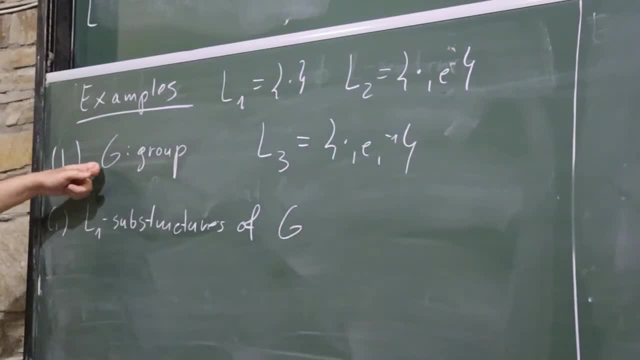 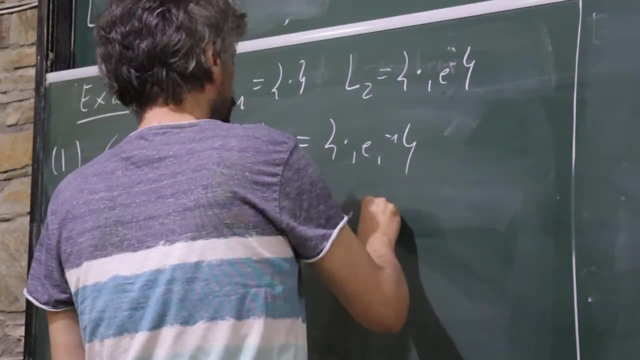 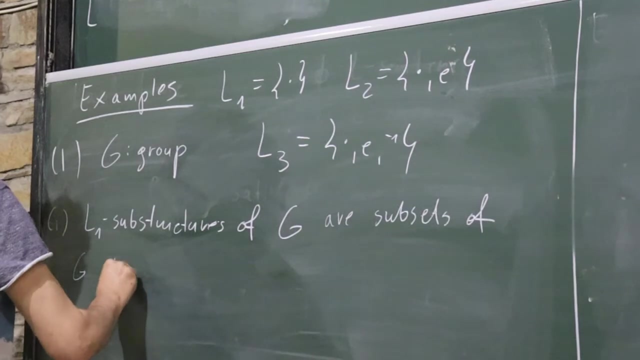 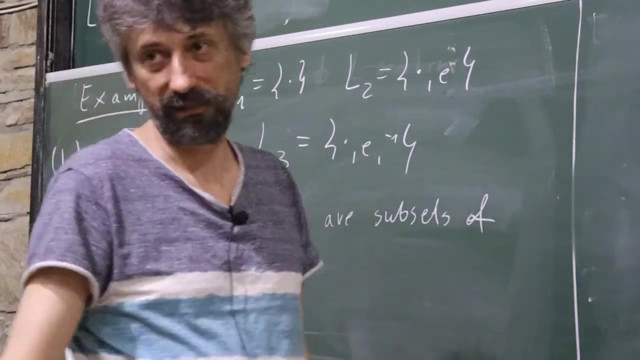 of g okay, and i don't care. now i denote by the same letter g and its universe. are subsets of g closed under okay, so they don't have to be subgroups, like natural numbers in z plus, or even numbers greater than a million in z plus are also closed under plus. better example: 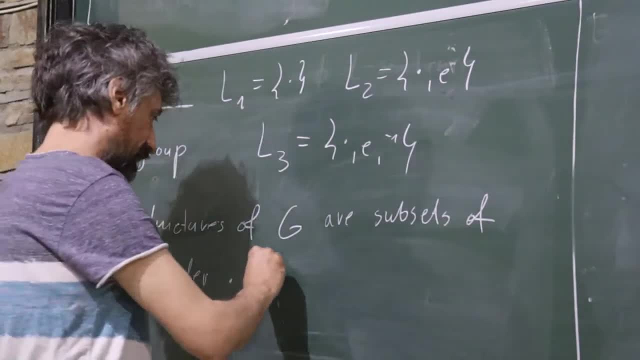 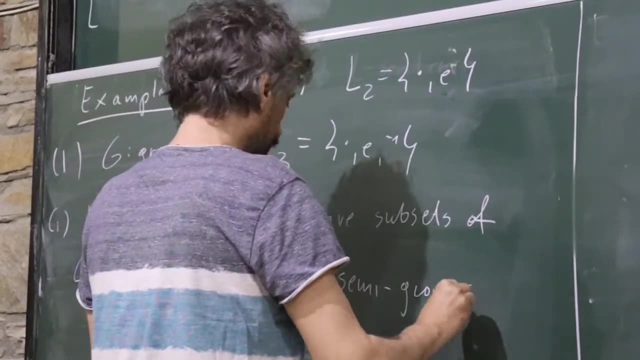 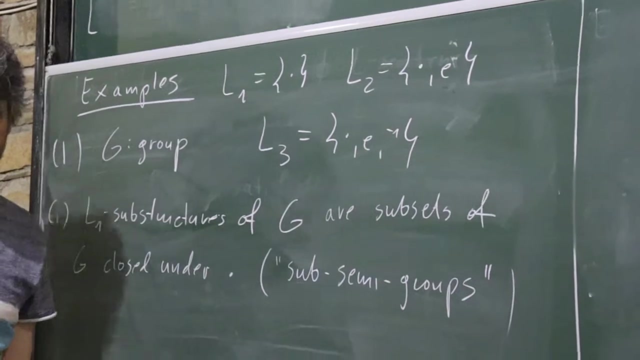 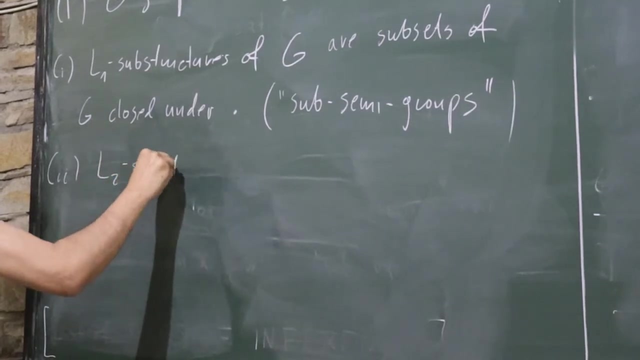 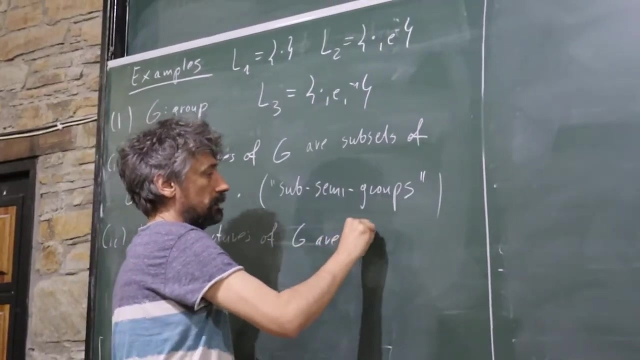 okay, so the word would be perhaps sub semigroups, so this good name would be language of semi-groups. i guess. l2 substructures of g, l2 substructures of g, of g, l2 substructures of g, l2 substructures of g- g are subsets of g. 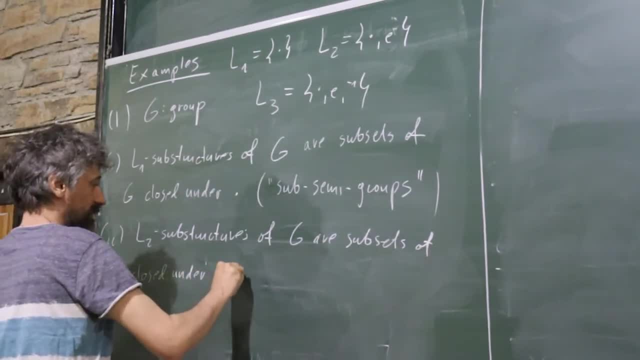 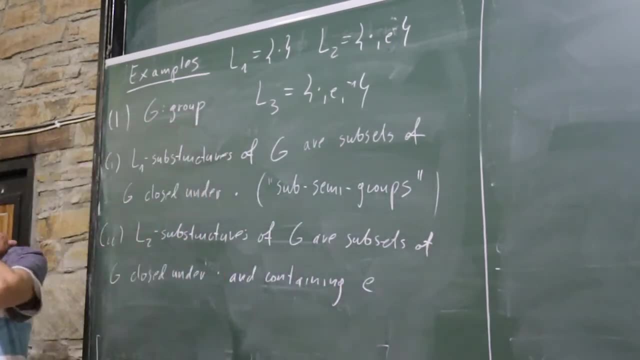 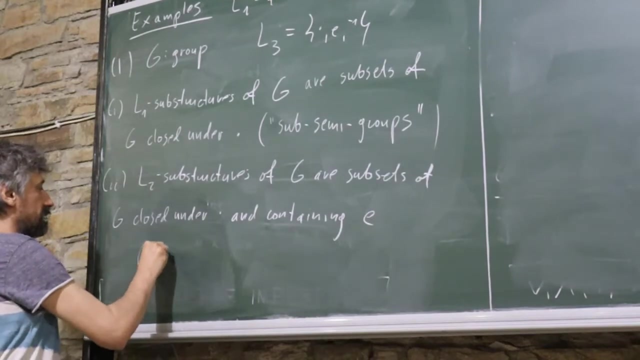 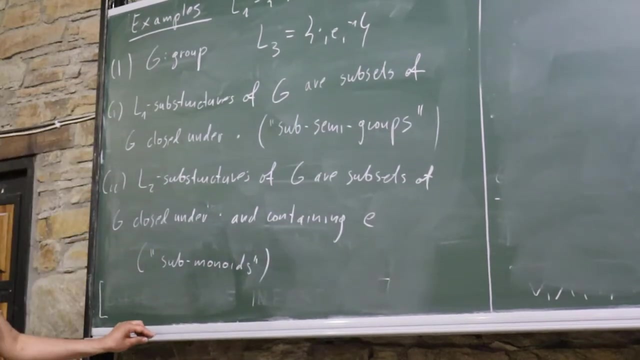 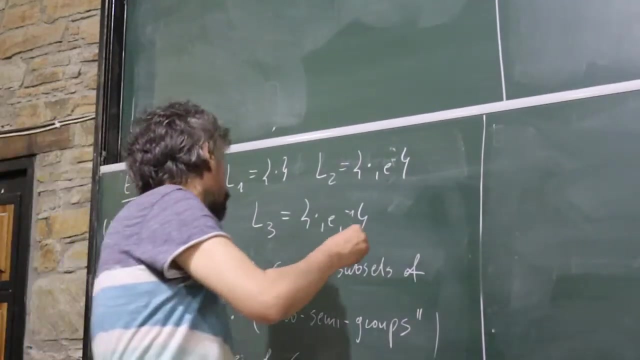 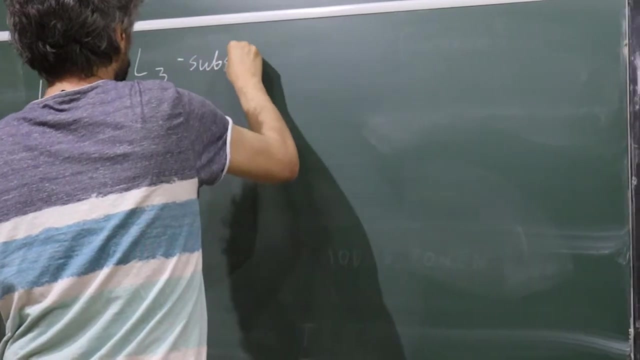 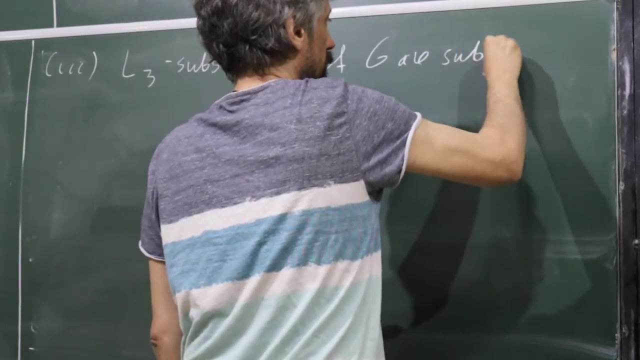 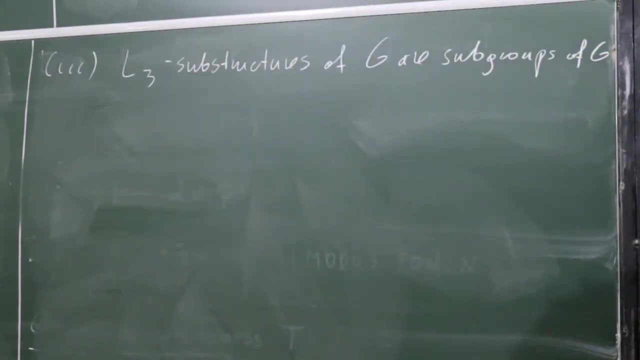 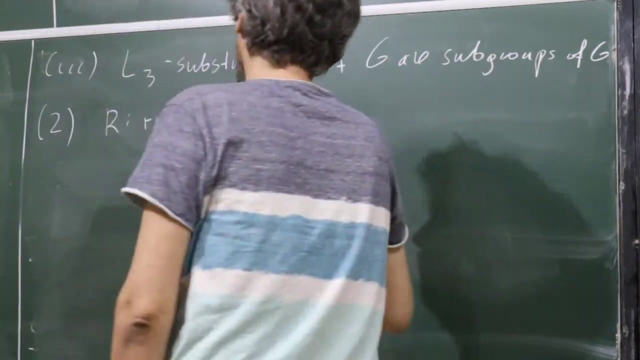 closed under and containing neutral elements. still, they don't have to be subgroups now, like n in z, so one of the names could be sub monoids or subsemi-groups with identity, and just in this third language, substructures are really subgroups- questions. so let's just do the same for a ring. 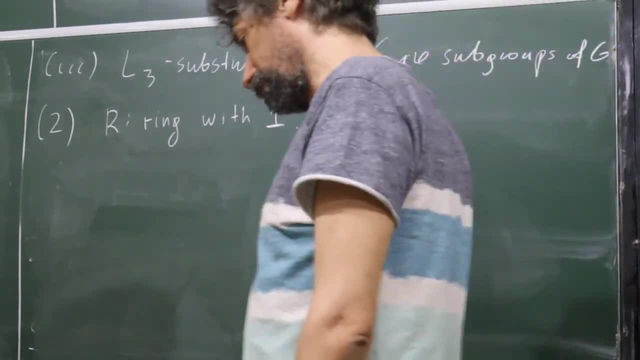 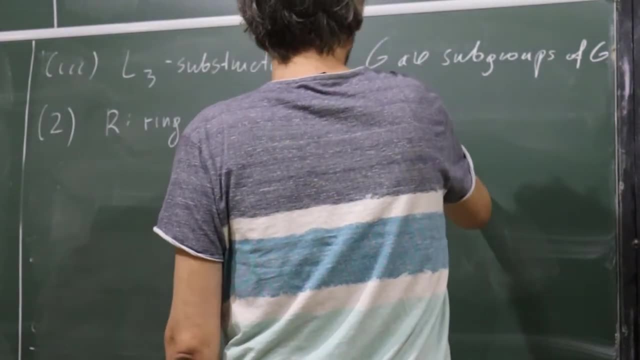 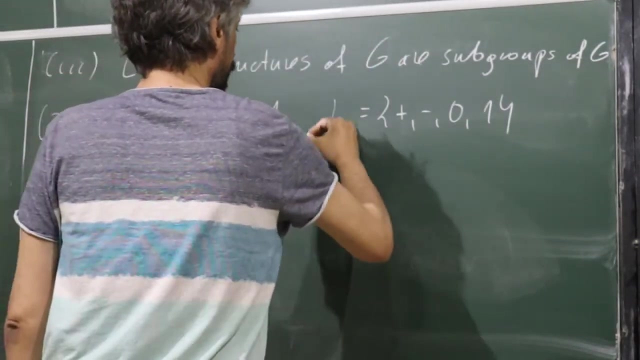 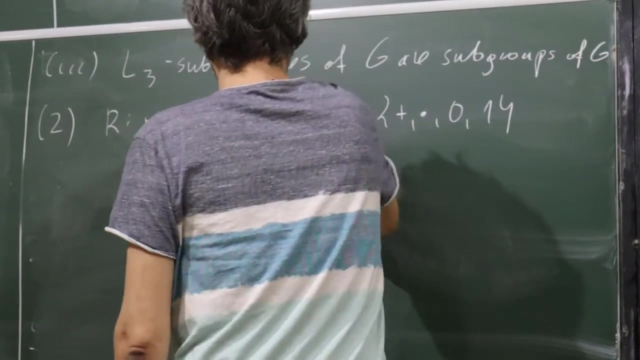 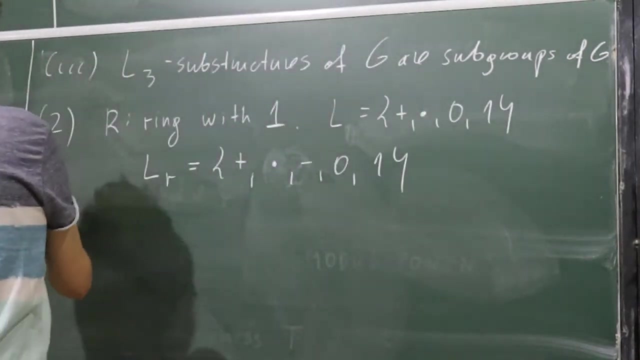 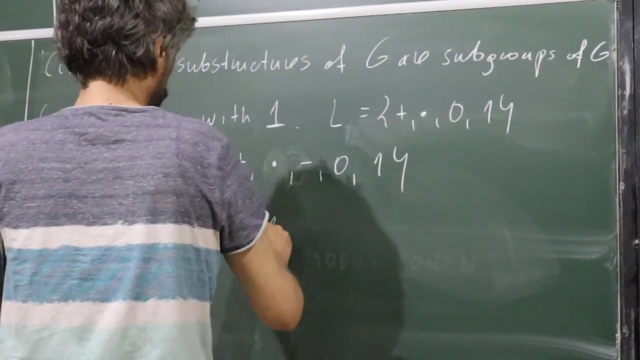 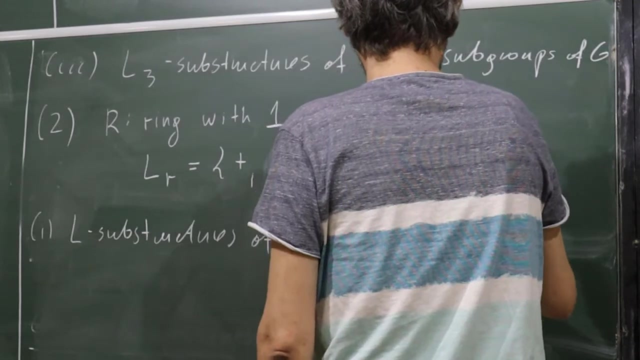 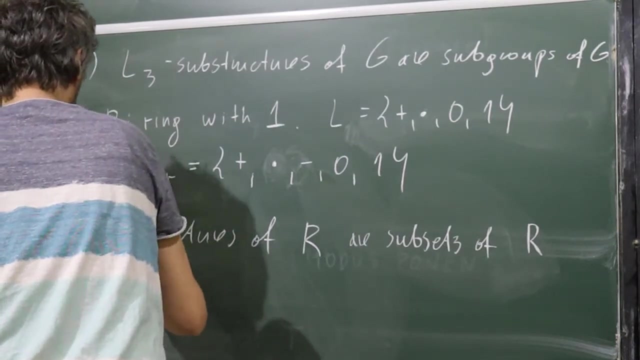 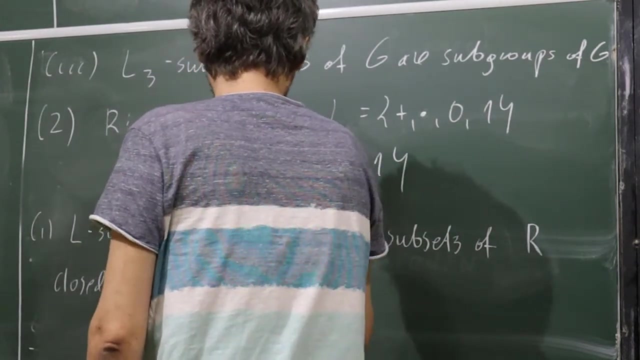 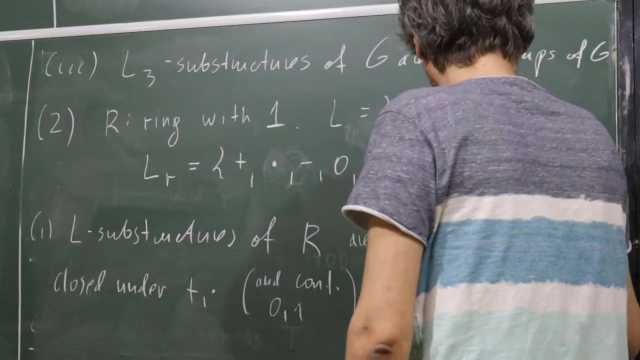 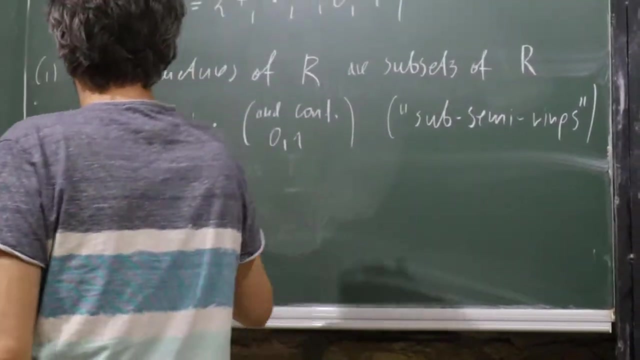 to get to our case. so if r, r is orange like this and Lr our, so maybe L now plus times- and L substructures of r are subsets of r, okay, and containing zero one, so something like subsemi rings. and finally, Lr substructures are exactly subrings. 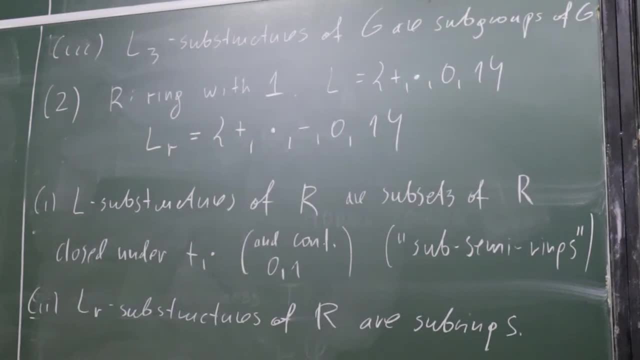 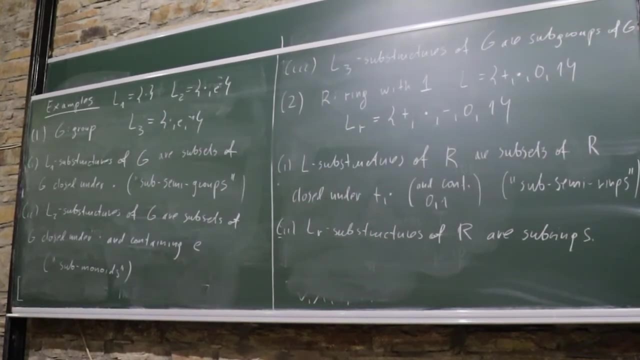 okay, so this was a bit long example, but also justification of names. why do we give particular names to particular languages? but also often we forget people could say this is language of groups, this language of groups, this language of groups. but most careful people would say this is language of groups. 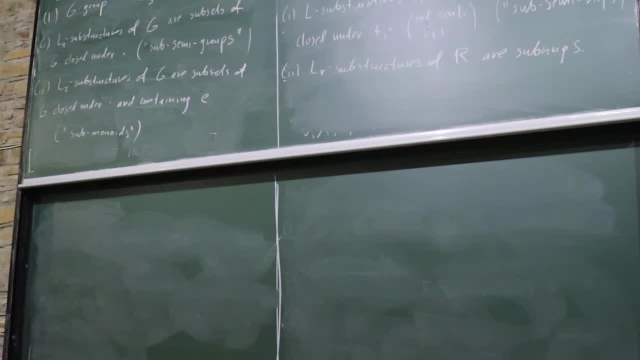 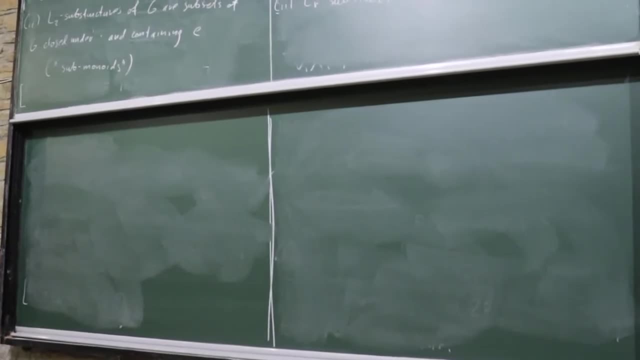 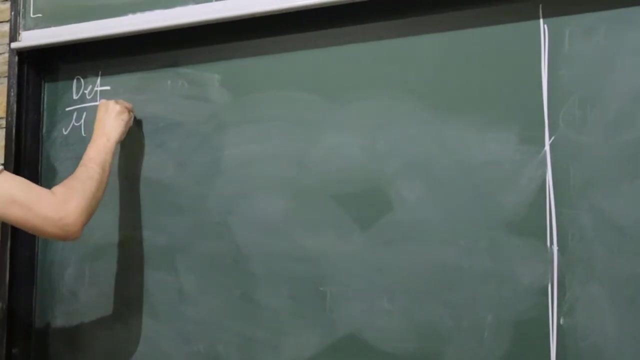 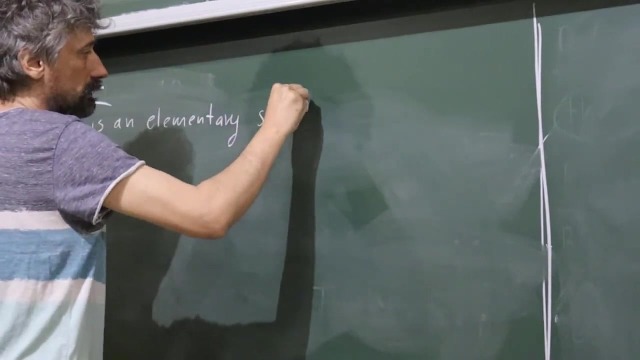 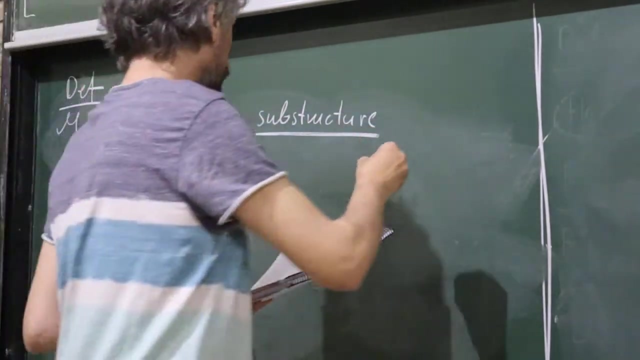 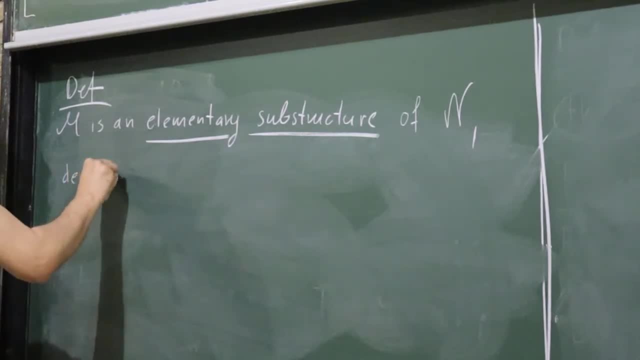 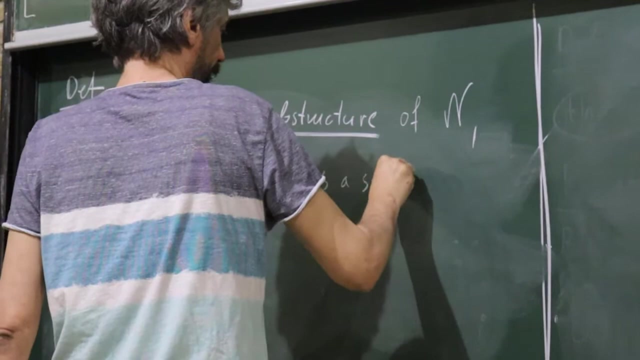 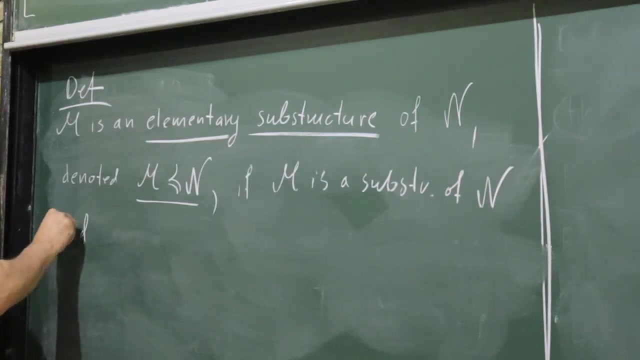 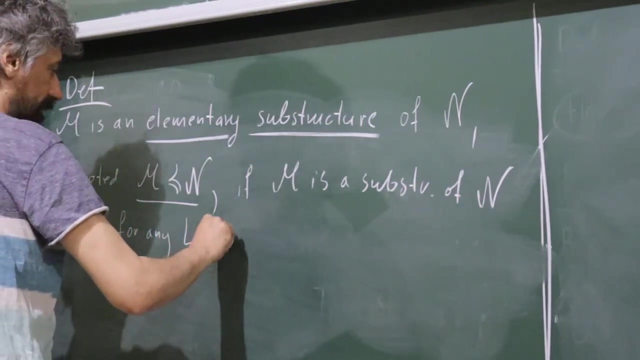 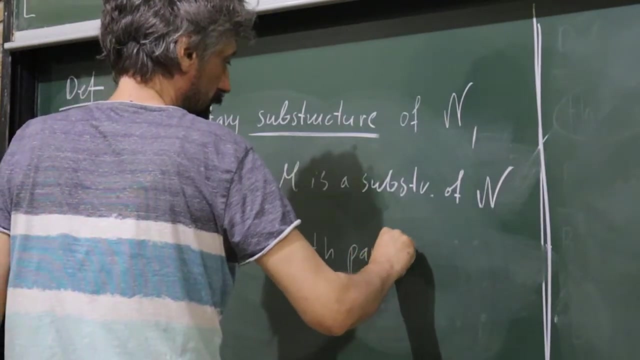 this is denoted. this is denoted, so. so like this, if it is a substructure, like this: if it is a substructure, but also it preserves the truth of sentences with parameters from m. so that's really strong condition. and for any l sentence, parameters from m. 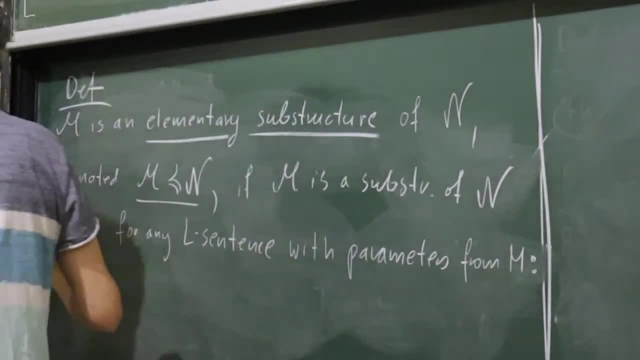 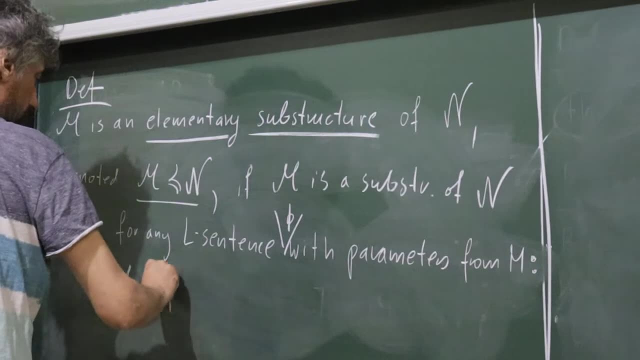 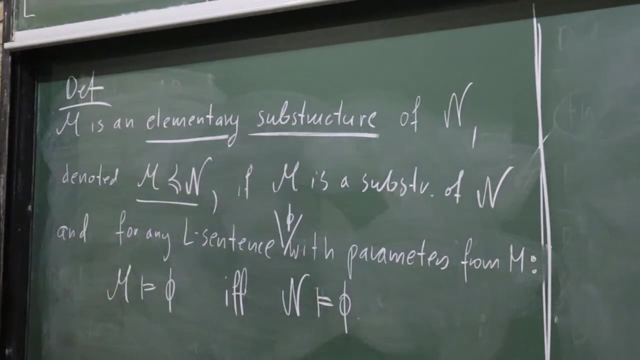 we have that it holds for any else, sentence v. okay, so first i will give some remarks about it and then some other examples. at this moment it's not easy to give any example of it, well, except trivial, except if m is equal to n. yes, because to give example we kind of have to know. 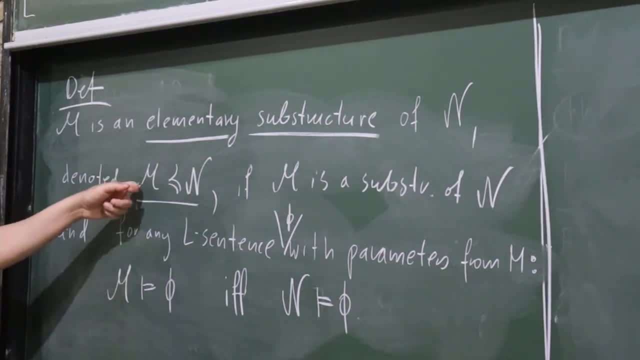 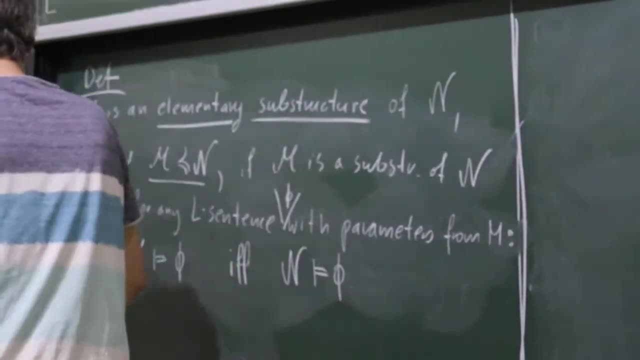 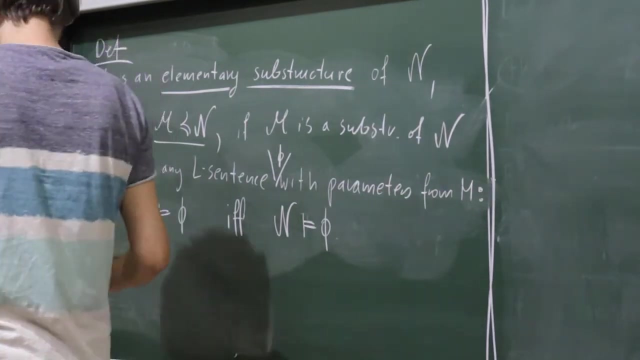 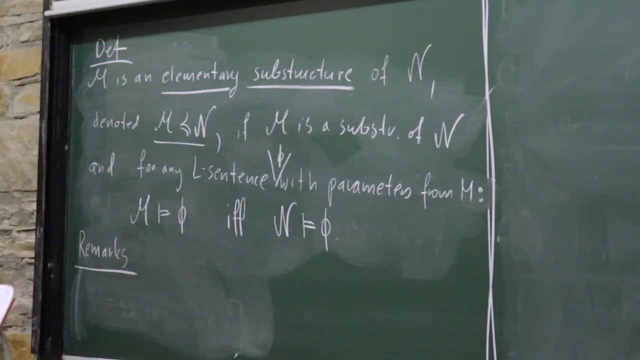 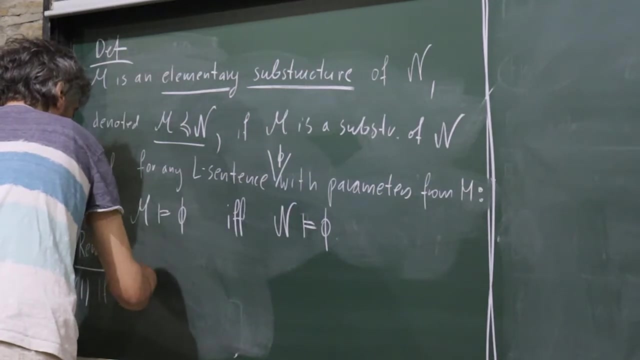 the full theory of it, even with all the names for elements of m. we will get some examples later, but it's never easy. so what are the remarks? so first, this is okay. all these remarks are aiming to say this is something stronger than elementary equivalence. so if m is a, 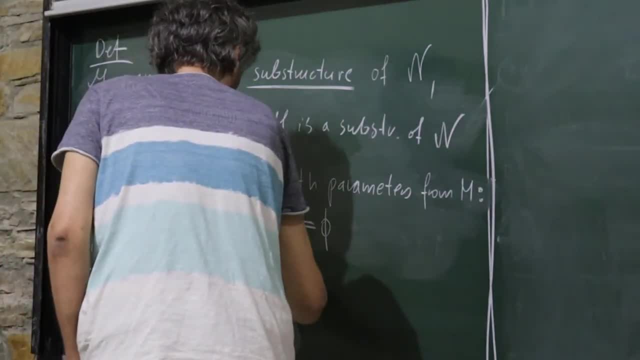 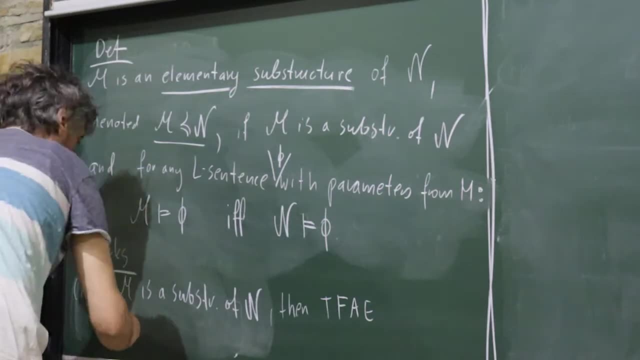 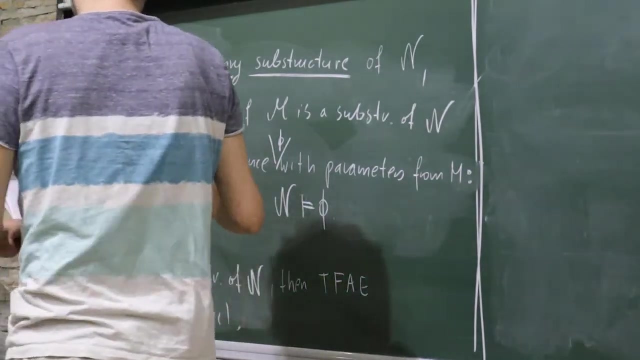 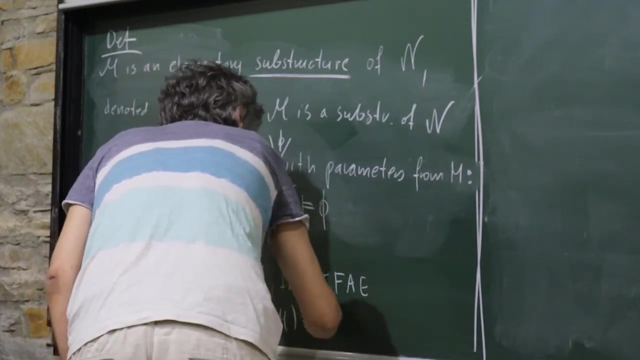 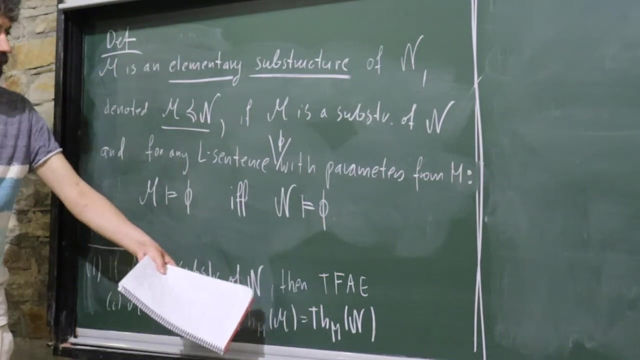 substructure of n, then it is elementary if, and only if, theories are the same- okay, if you remember this notation- but with the language containing parameters from M, exactly like here. yes, not just sentences, not just sentences in the original language, but we are allowed to put parameters from this smaller structure, M, which are, of course, naturally interpreted. 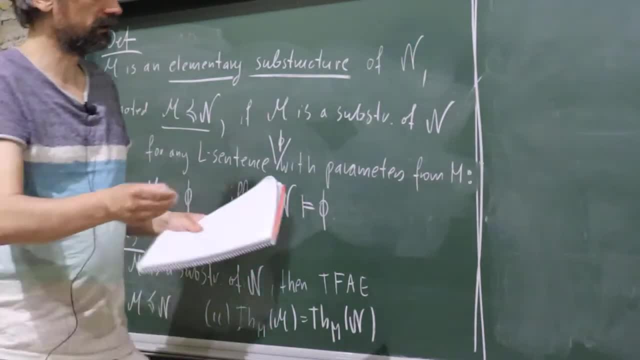 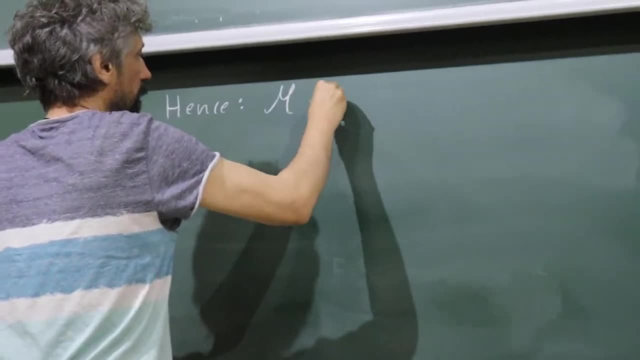 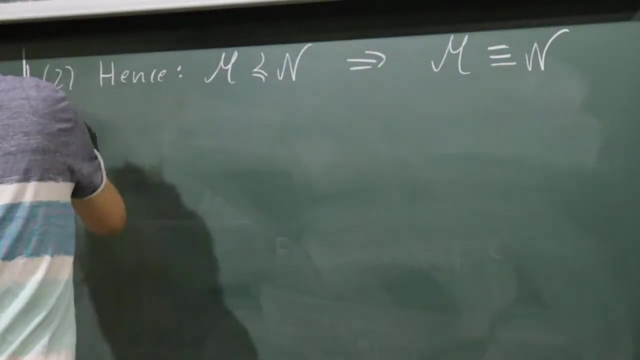 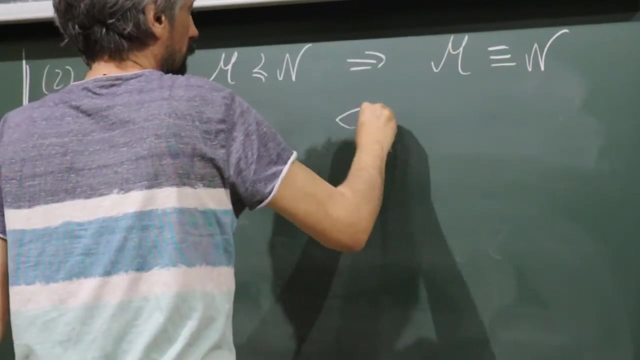 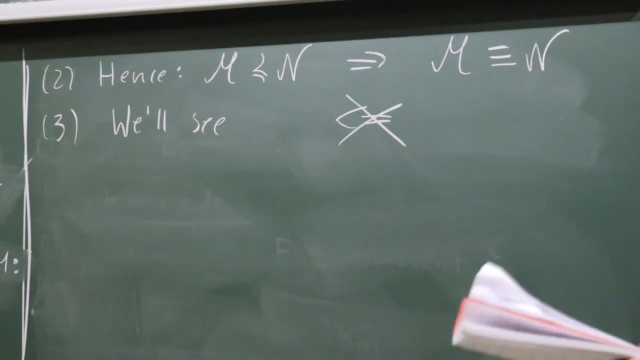 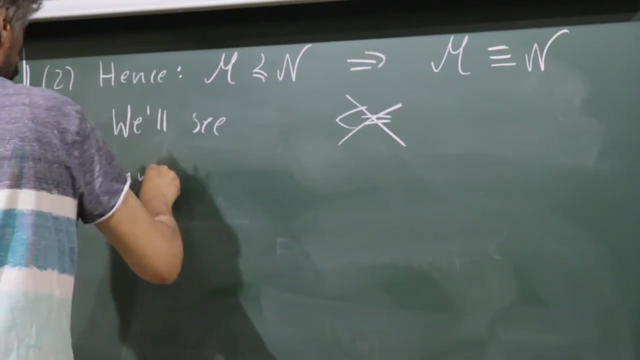 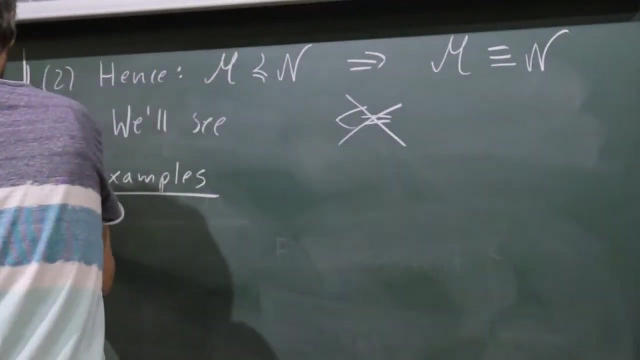 here. so it is something more. so it implies, but we will see that it's not the same, okay, so let's see some non-examples first. so almost anything you just take will be not, because any substructure taken at random will not be an example. for example, R is not in C. 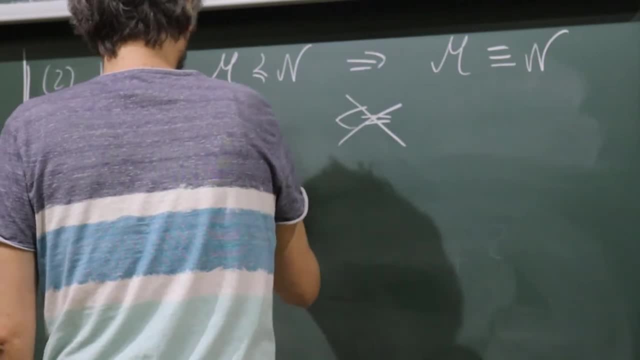 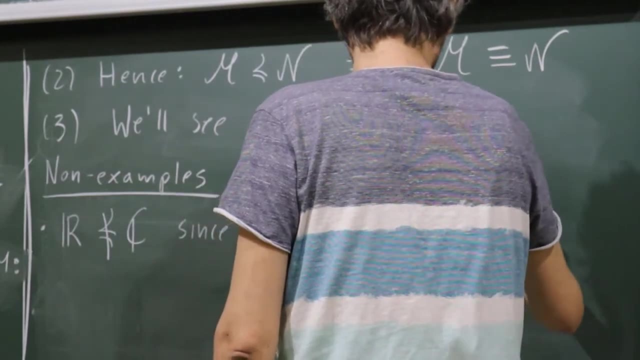 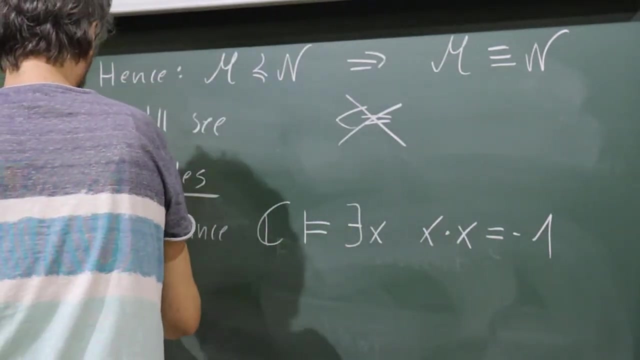 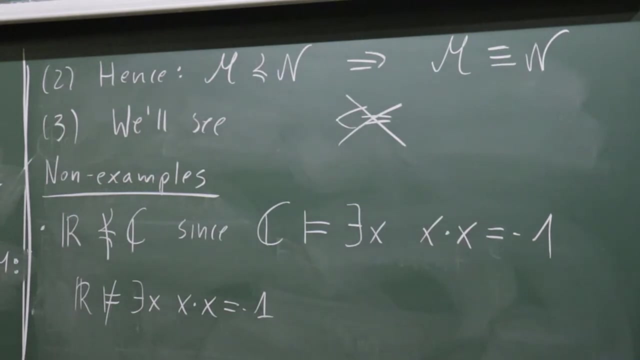 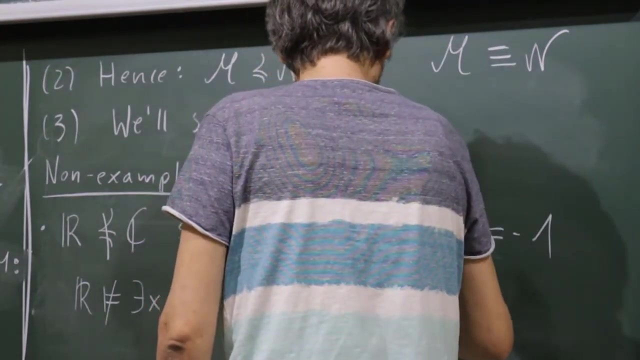 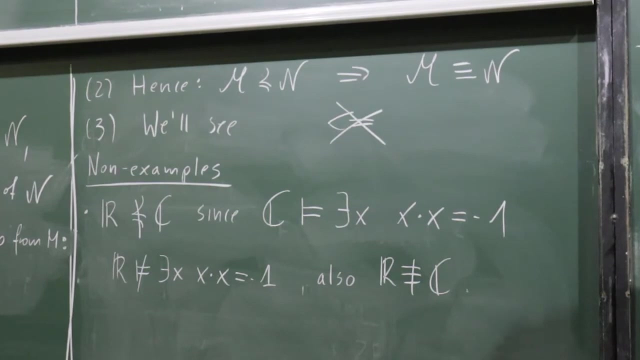 because, yes, here we have square root of minus one here, not okay, and this seems to be using parameter, but it's not using one is the constant from the language. so even okay, so, so, so, so, so, go on. also, this holds, which is here stronger? it's in the context of the theory, this concept of elementary substructure. 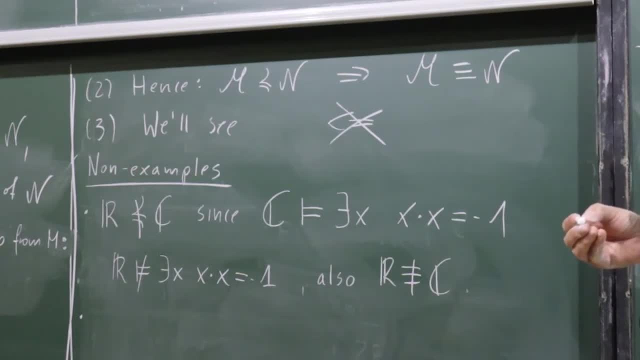 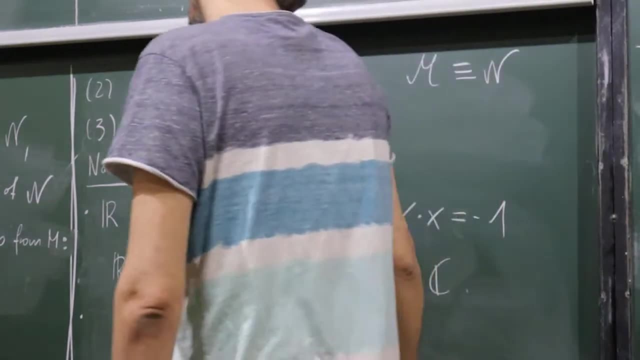 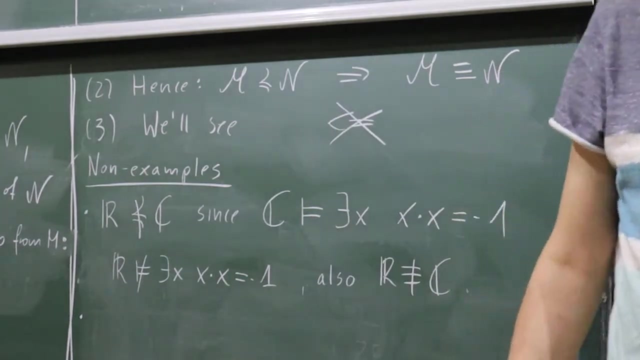 in which, ah, yes, okay, I mean it's about structures, only there is no underlying theory. yes, yes, yes, but usually in practice it is. we are taking subgroups, subfields. I mean, if we take a substructure of a group which is not even a group, then of course it's not elementary, but it's a kind. 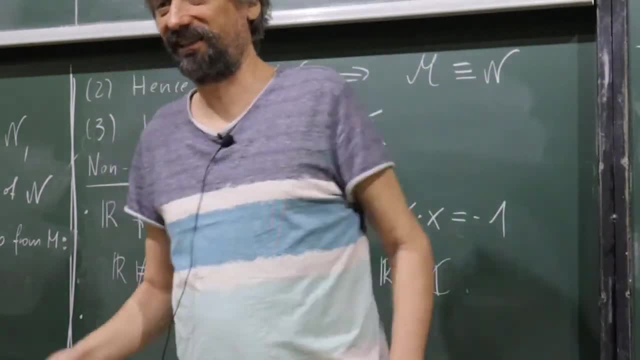 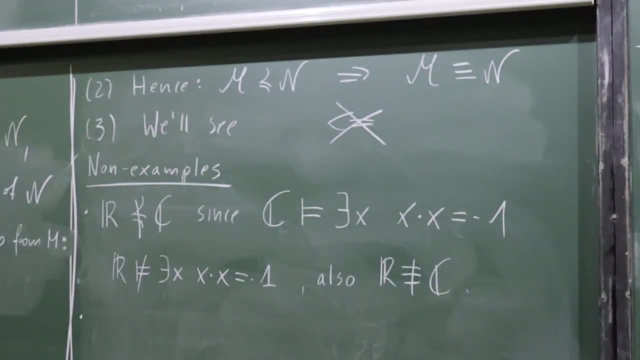 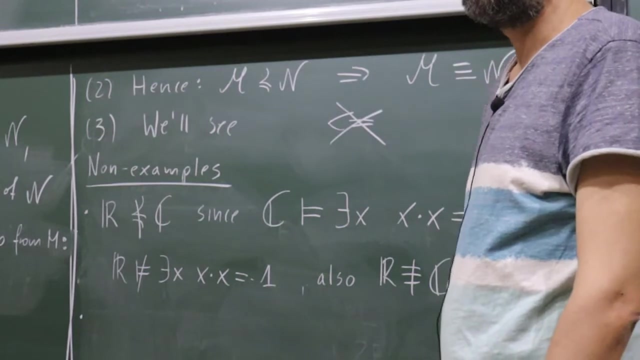 of morally? okay, formally not, but morally there is some bigger theory around always. but yes, it's formal, it's only about structures. does it use parameters for c? no, it doesn't use parameters from anywhere here, not nowhere. minus one is not a parameter. what if you write: 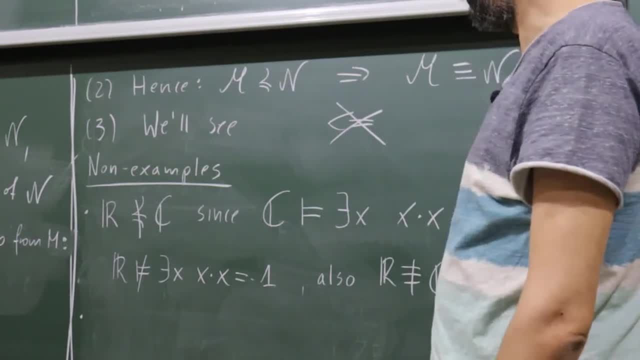 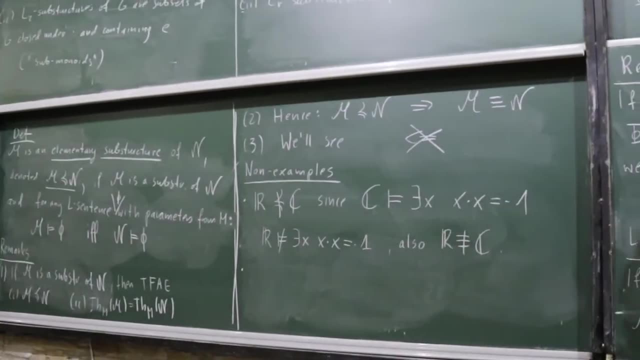 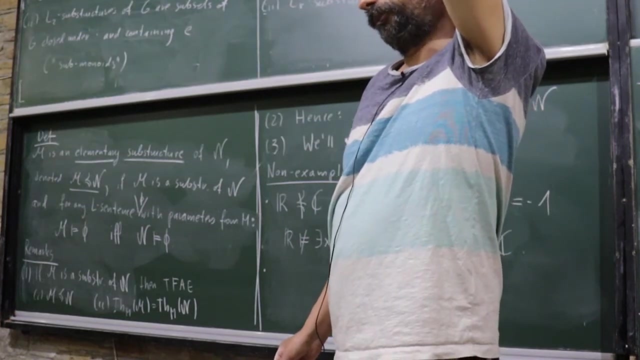 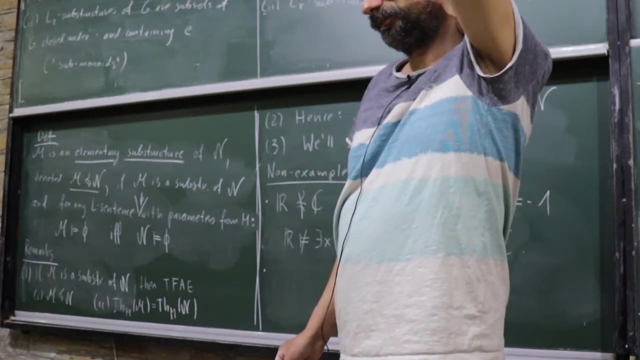 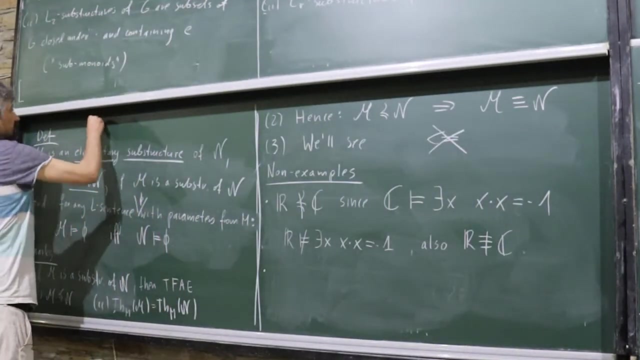 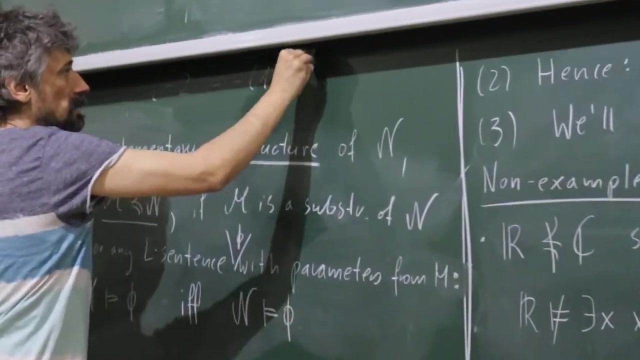 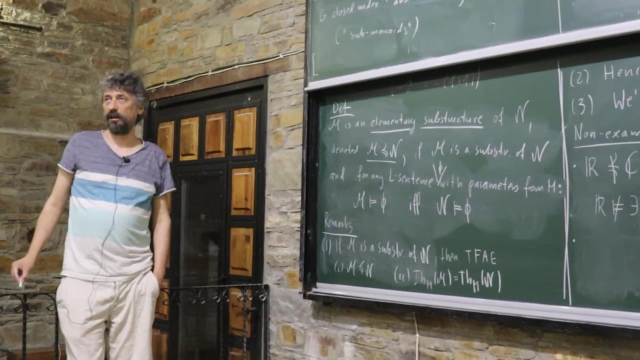 minus two. it is still not okay. it is both minus one plus minus one is minus two. so you can define minus 2 without any parametrics, with only constants, constant symbols. so minus 2, yeah, minus 2 is defined as, let's say, minus square root of 2. 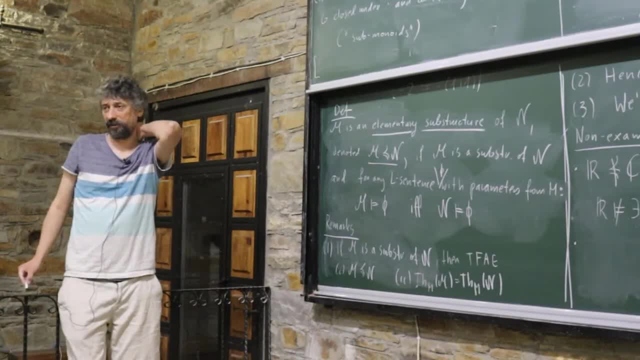 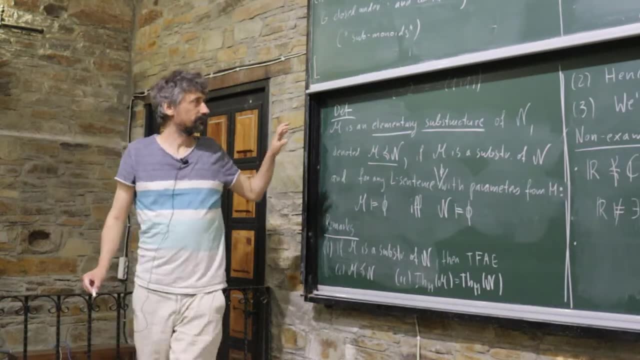 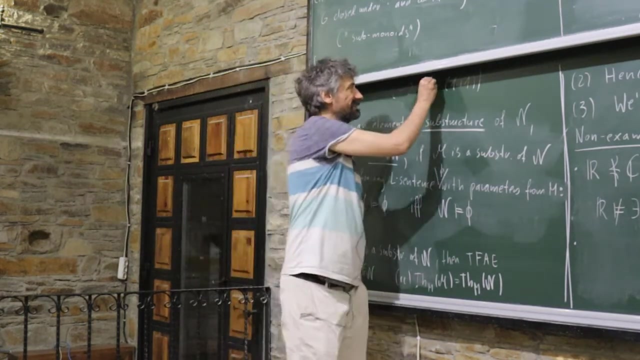 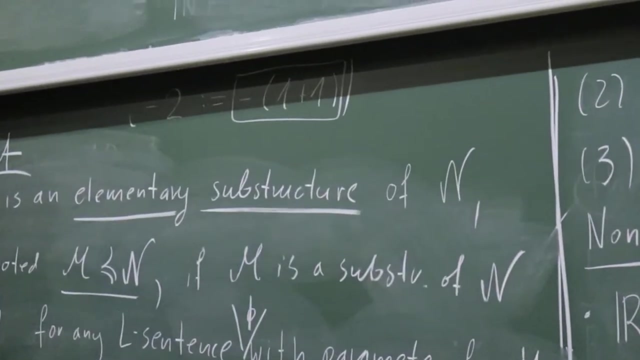 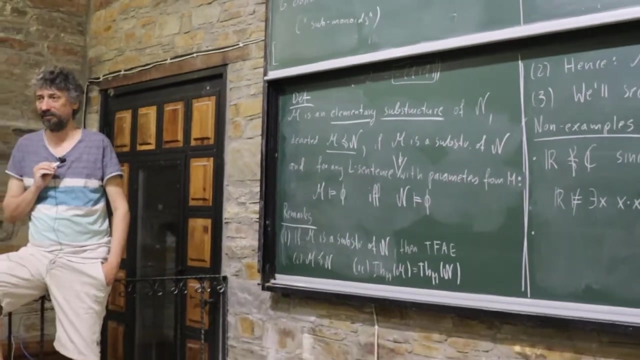 is something which depends on the difference between definable and the break closure. this is like a term. you can define it. something like that, something like that, something like this is a part of language and it has interpretation in every LR structure, unique interpretation. so constants are also like this. 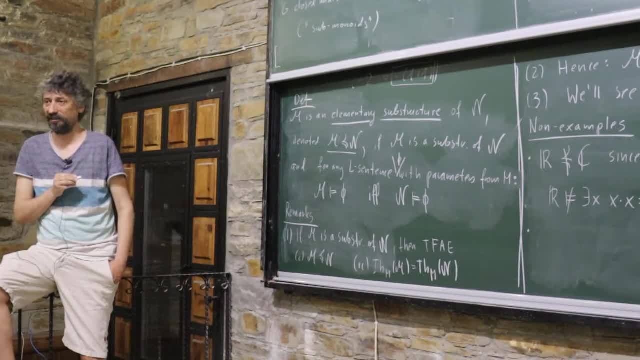 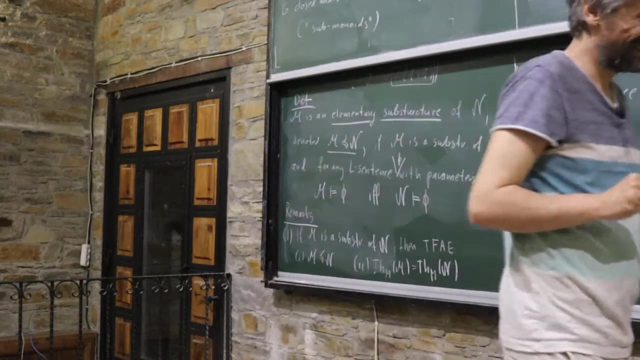 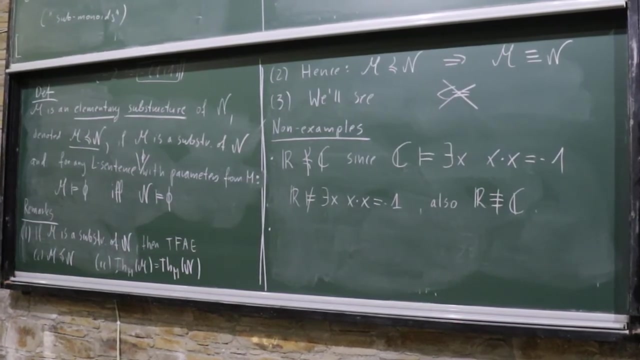 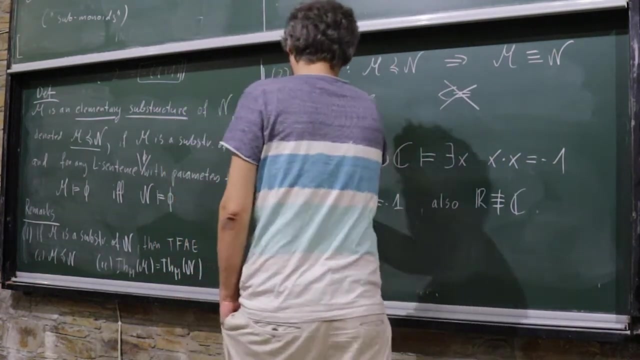 and this is very close to being a constant. there will be example, maybe. third example will use a parameter like, which will be also one: ah wait, okay. but so I will do more precisely. third example that I plan, but still okay, okay. so here I should say: but we understand I'm talking about. 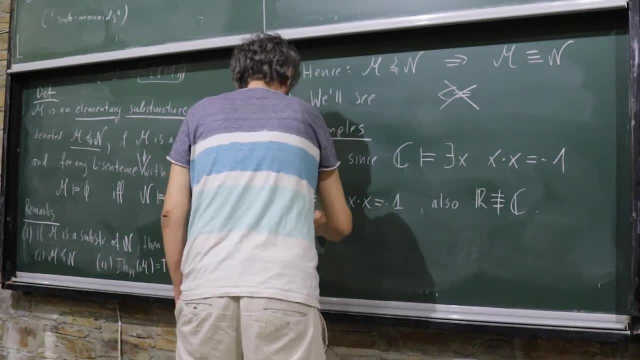 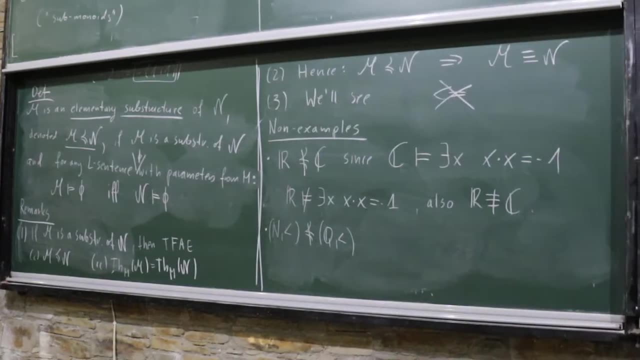 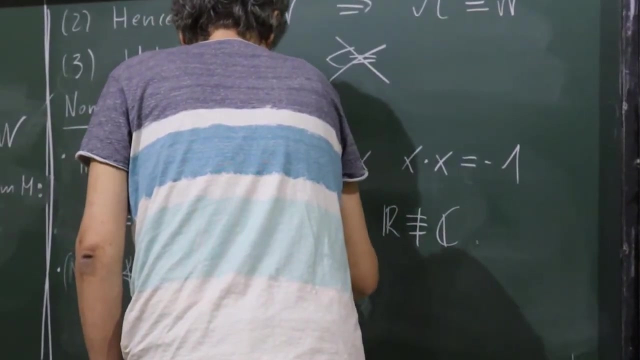 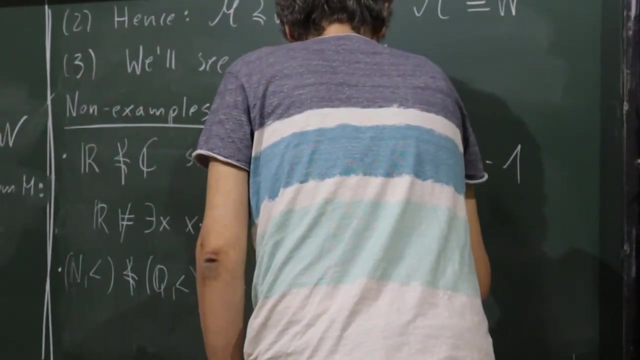 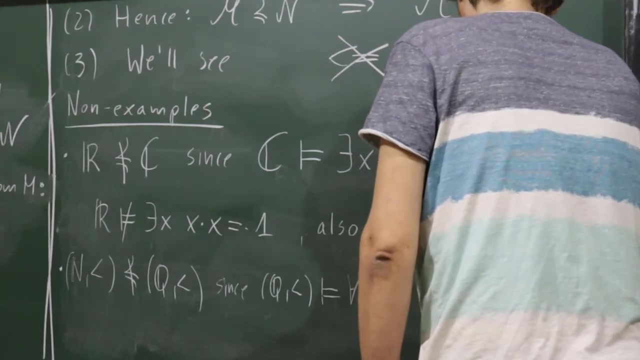 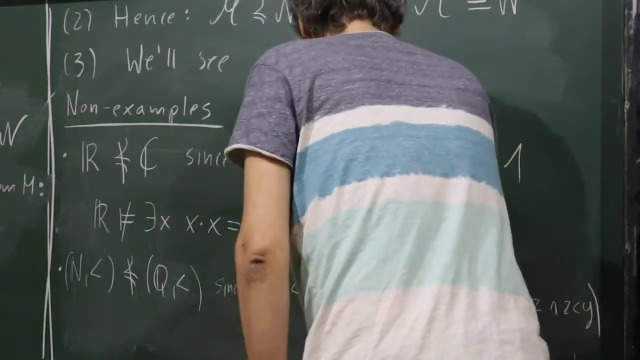 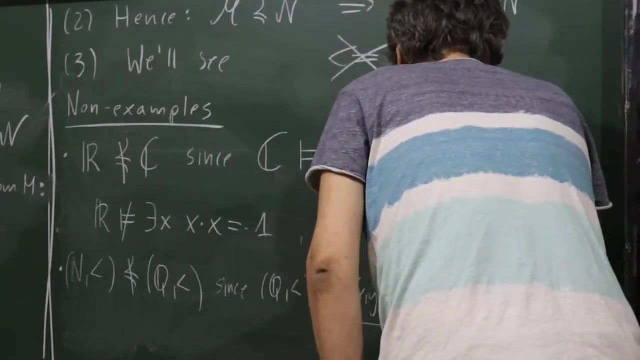 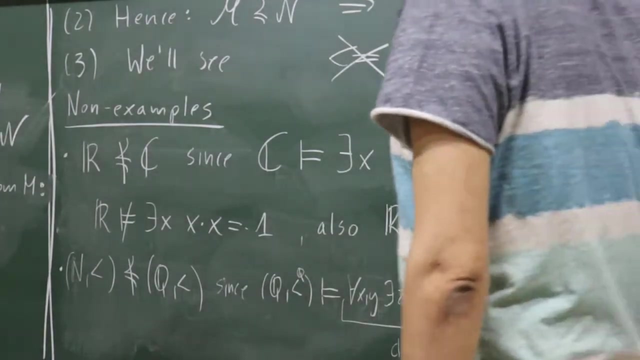 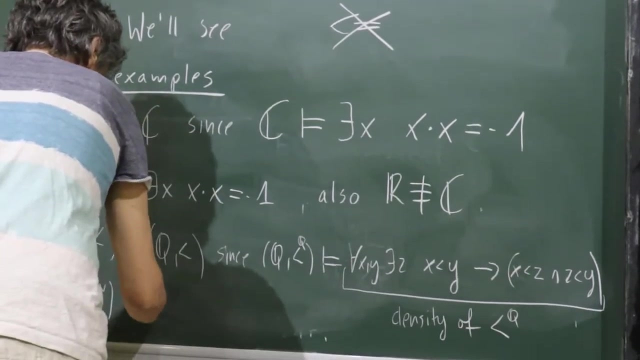 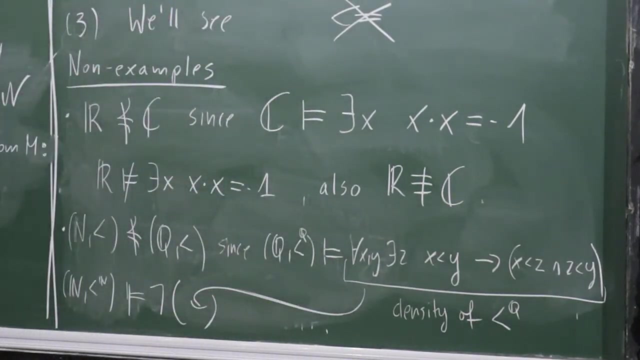 rings or fields, ahem, and again we have to give an example that when we compare the elements, as we cannot see, this is a not even elementary equivalent. but again, they are not even elementary equivalent. well, this is dense for each. so, for each Maybe, but it's not true. the ordering of natural numbers is not dense. 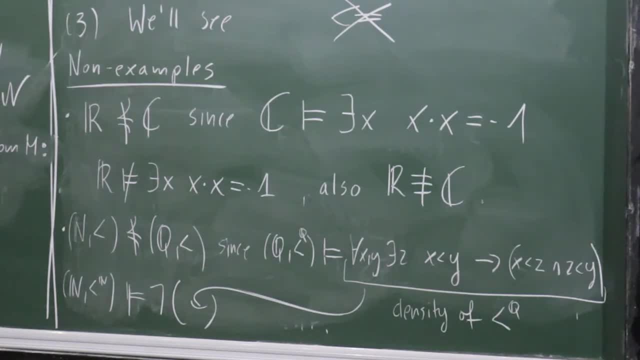 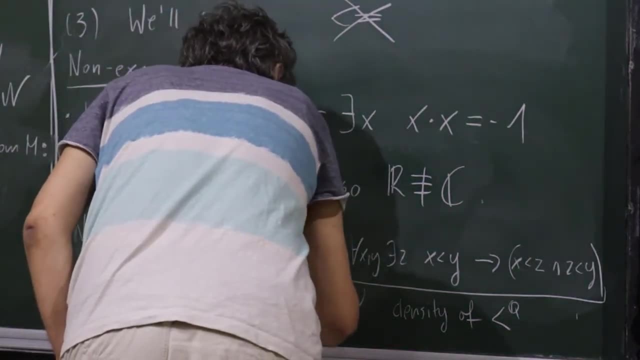 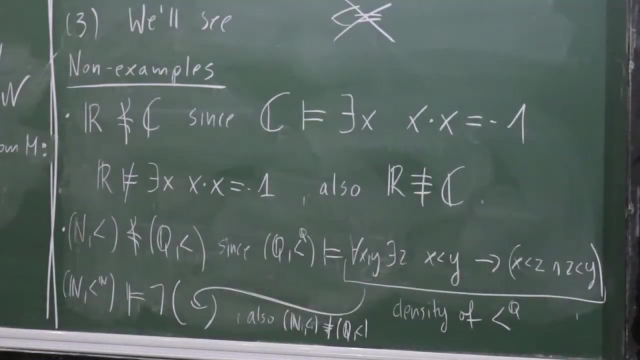 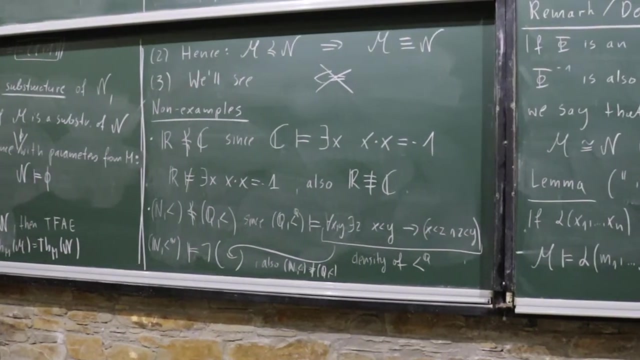 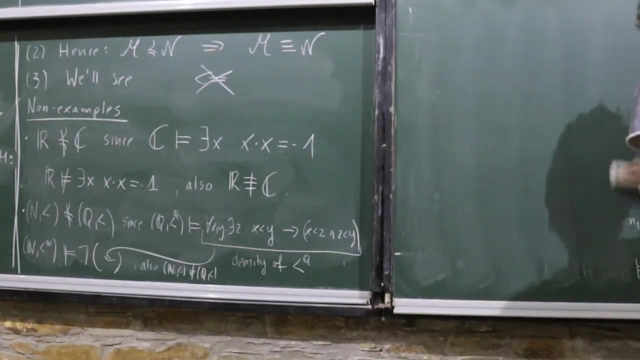 You cannot put anything inside 0 and 1,, but still there were no parameters, as here. So now, finally, example: when even the smaller structure is isomorphic to bigger, but it's still not elementary substructure. Okay, And now we will see this parameter. 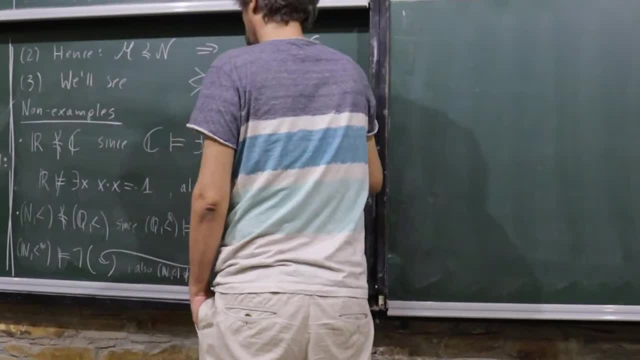 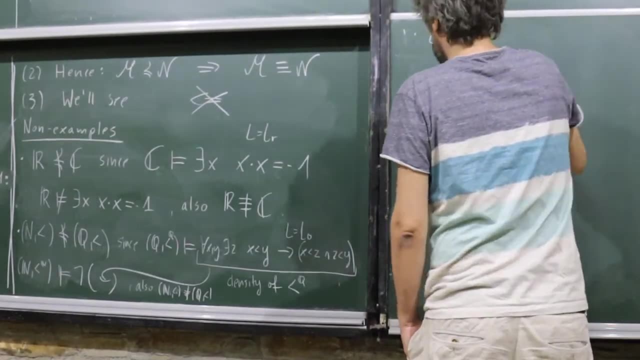 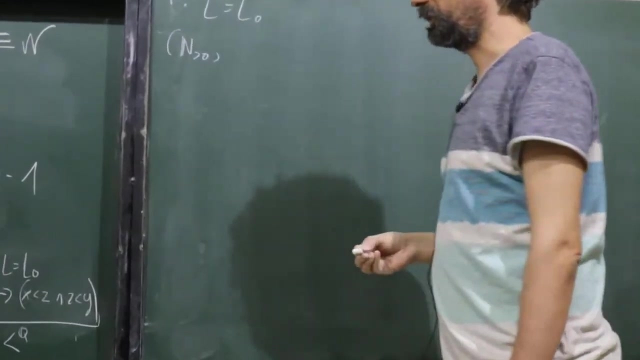 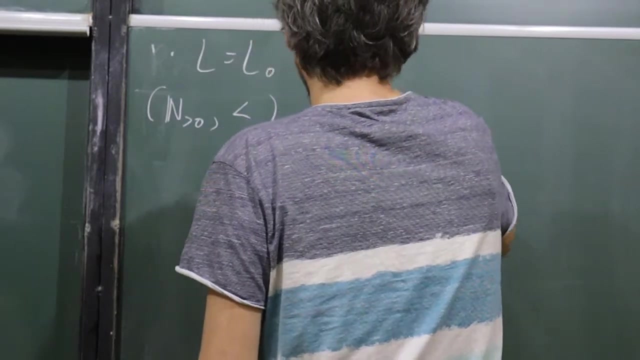 So in the same. so, of course, here L was language of rings, here L was language of orders. Okay, So I'm saying that natural numbers greater than 0, for me, natural numbers includes 0, is not. so what is the statement? 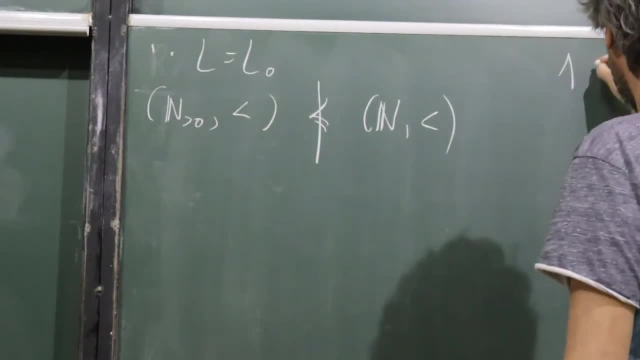 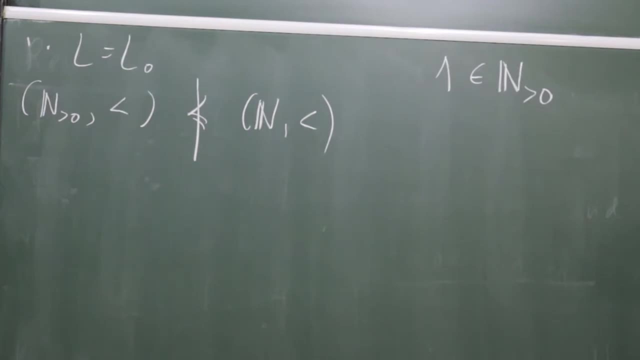 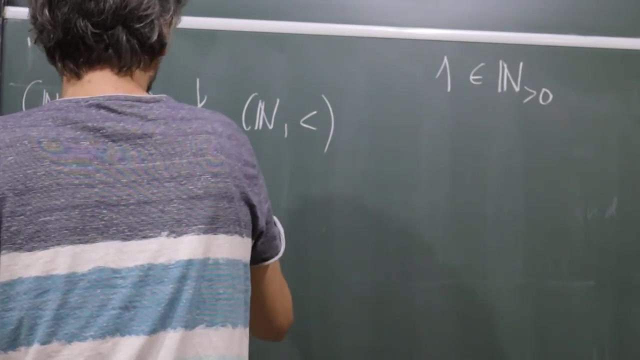 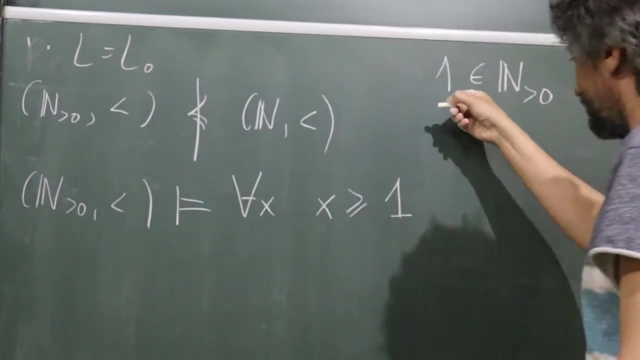 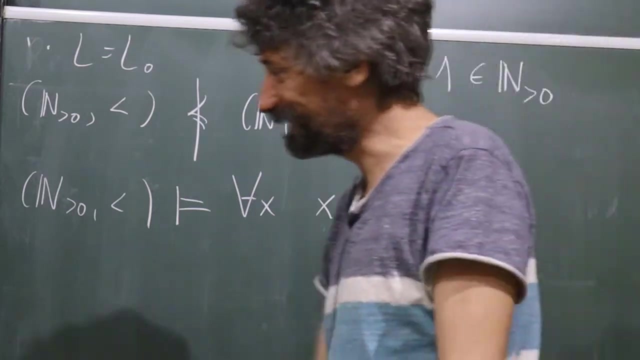 Now I will use parameter 1.. Okay, Okay, It's not in the language. there are no constants in the language and the statement is: for all x this: this particular one has an element here, not to be confused with this one, which. 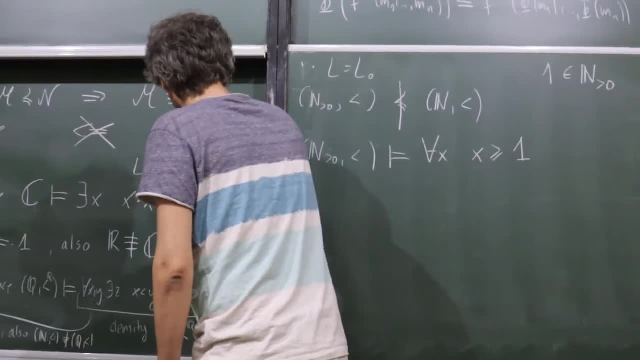 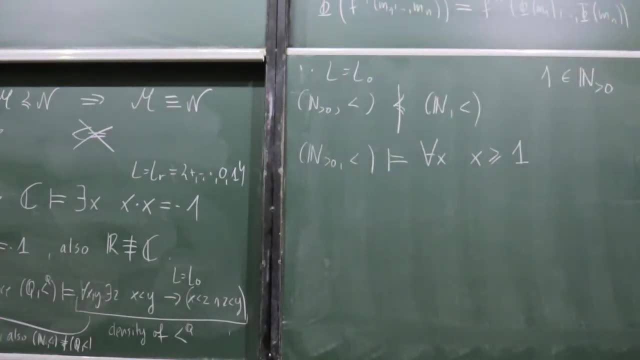 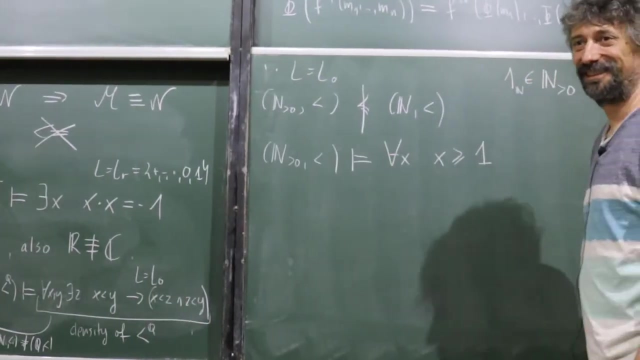 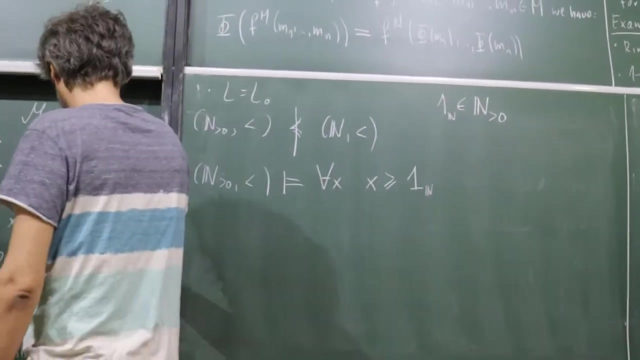 is: Okay, Okay, Okay, Yeah, that's that may give some headache, because we have: yeah, I guess here it should be written 1n. if you want, What? if you write 1c? I could write 1c, but the statement is like this. the sentence is like: no, I could, but 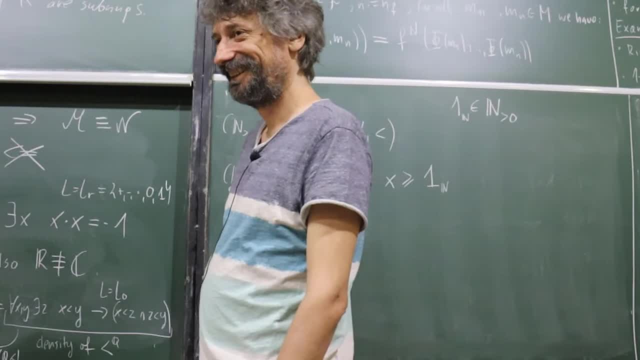 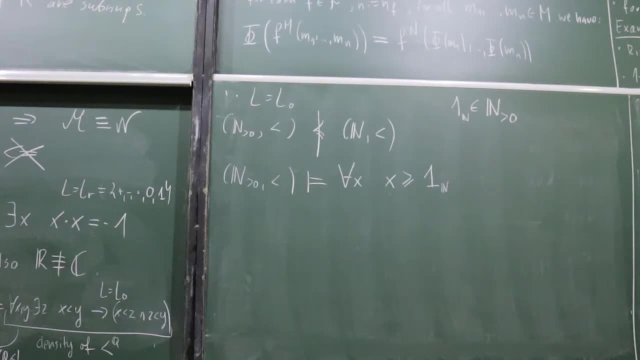 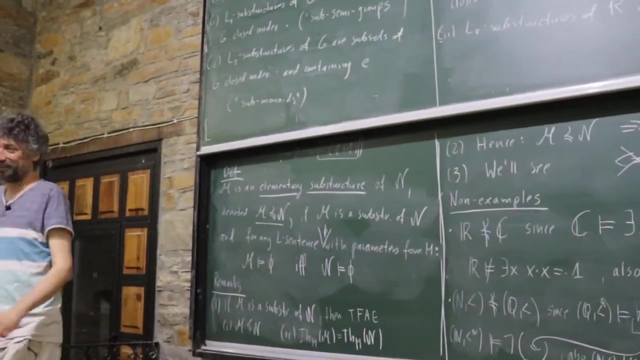 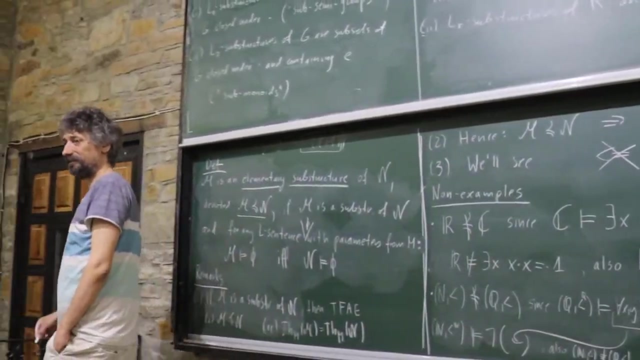 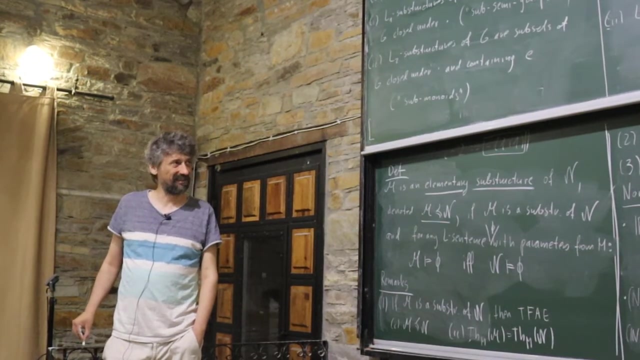 this is also okay. this is also okay, because then I interpret this element as this: then it becomes actually a sentence with parameters from c, which exactly the same meaning: but, yes, but, but here this one means really a constant symbol. ah, then there will be two possibilities. 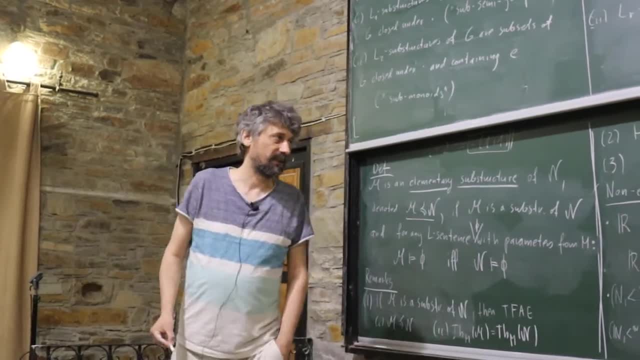 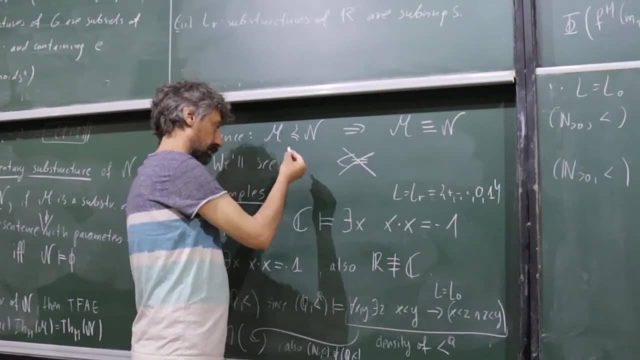 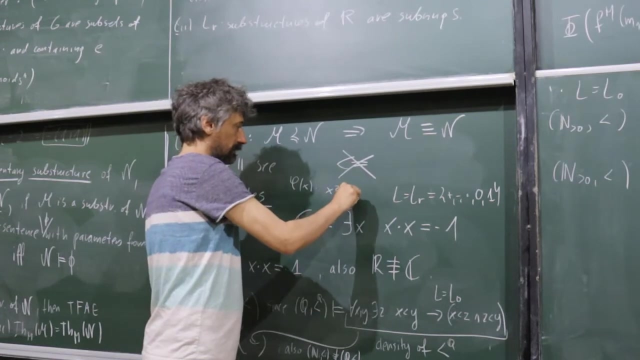 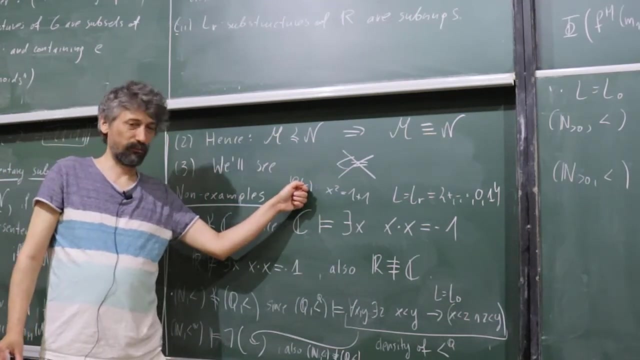 so then there will be just definable set which kind of there will be formula in your example. so I haven't finished that, but in your example it will be formula. okay, it really will be formula v of x. okay, okay, okay, okay, okay. and then the formulas, the elements which satisfy this formula. usually there are two. 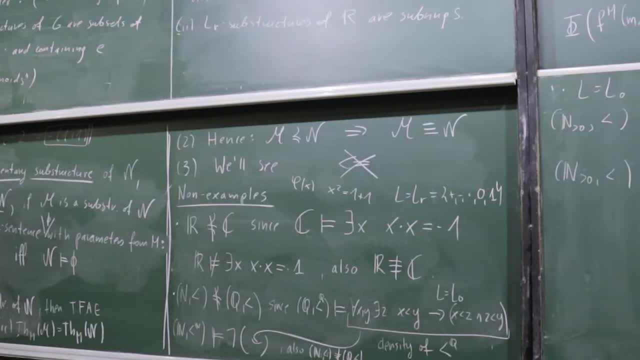 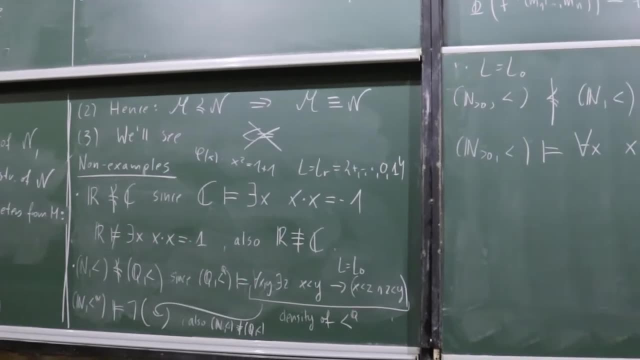 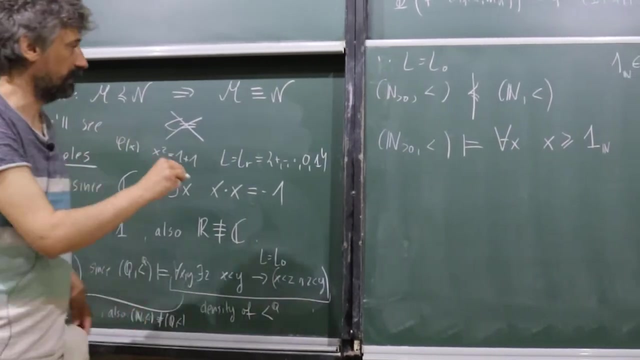 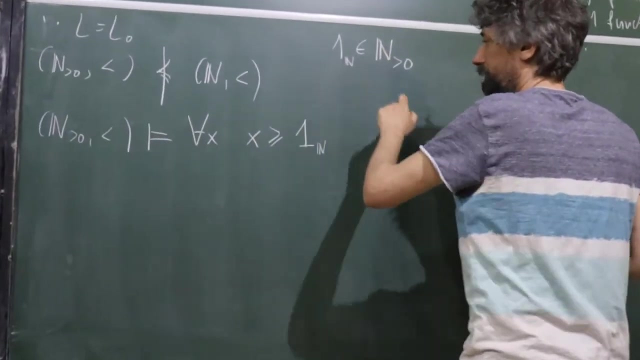 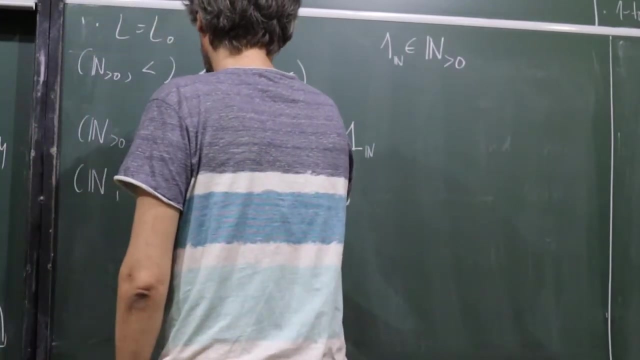 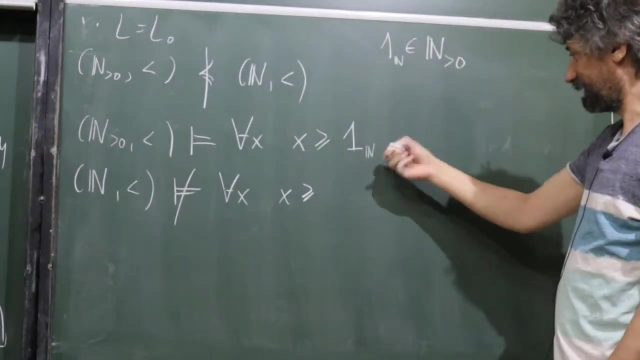 of them in every model. yeah, and that's it, and this is square root of two, I hope, yeah, okay, I could probably uh answer it a little bit smaller, okay, but this is true. so one is the smallest element in natural numbers greater than zero, but well, I could also put here greater, well. 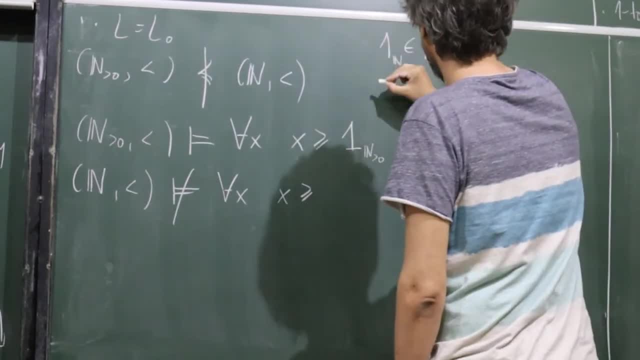 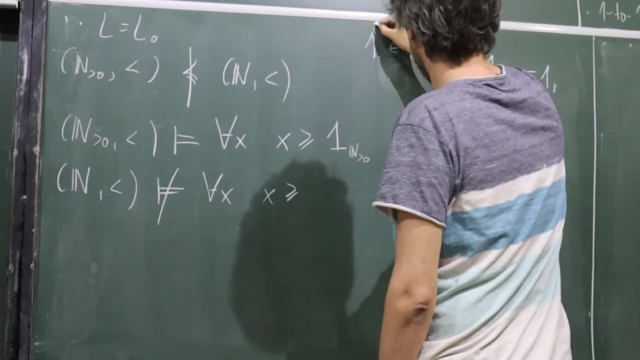 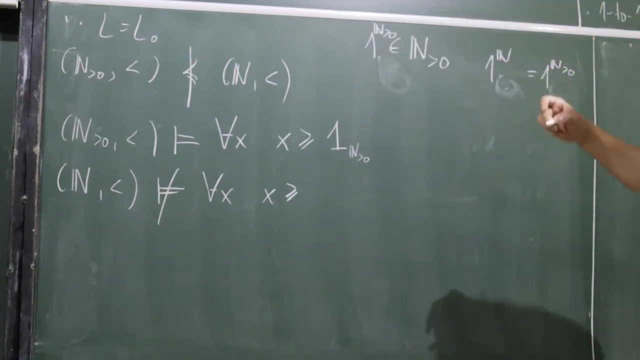 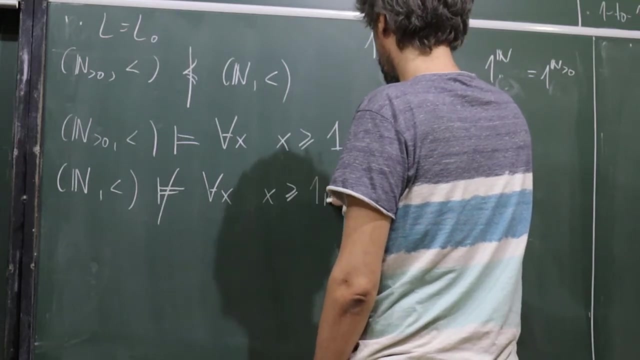 so you see what happens if I try to write a powerless word. I don't know the exact set. yes, of honor, and they should be up because it's a substructure. so one is the same. you take the parameters from substructure which are naturally interpreted. ok, I should not say that. 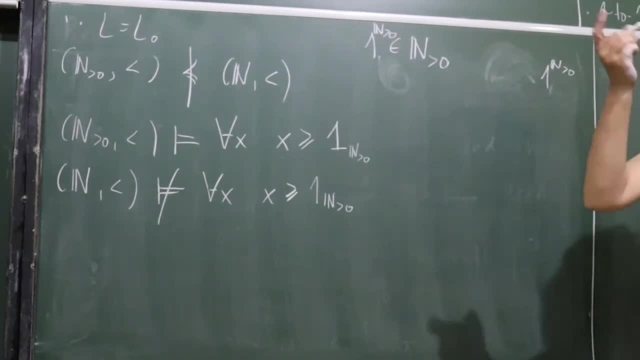 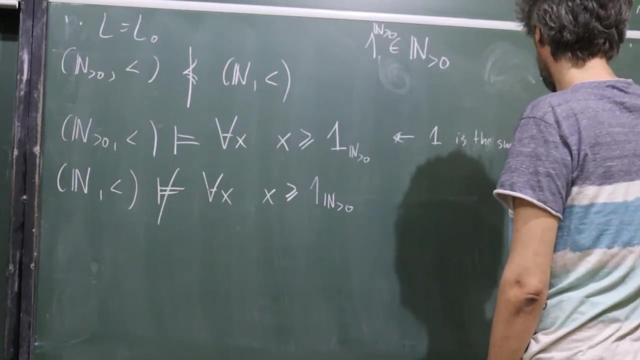 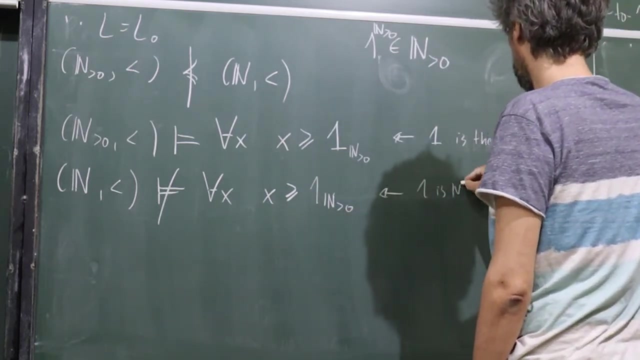 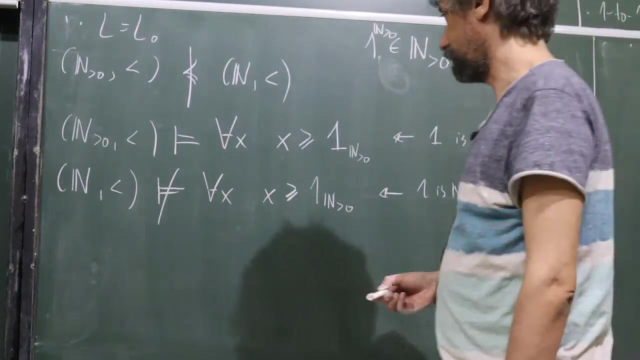 it's parameter from substructure is naturally interpreted in superstructure as the same element. but anyway, this is our real one. so here one is the smallest element, here one is not, because there is also zero, ok, so it's not elementary substructure exactly, but the function. 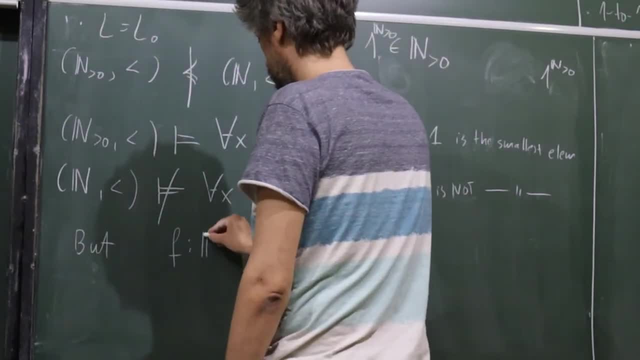 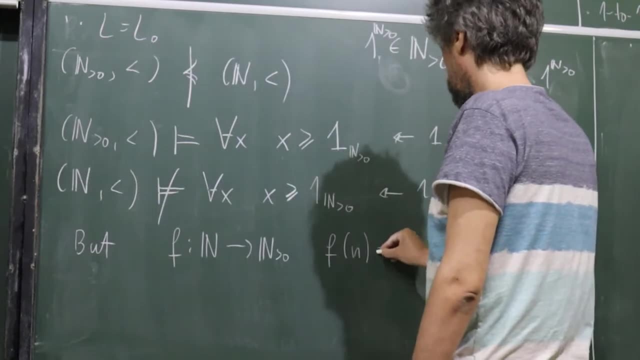 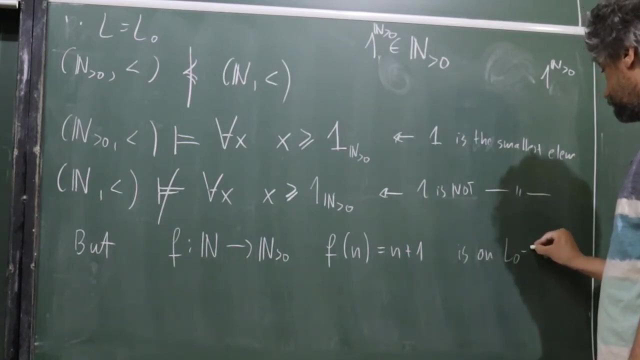 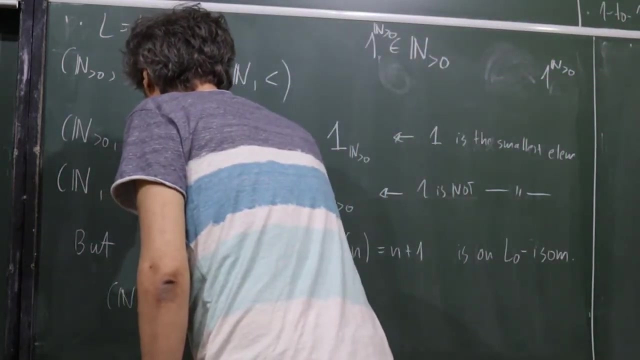 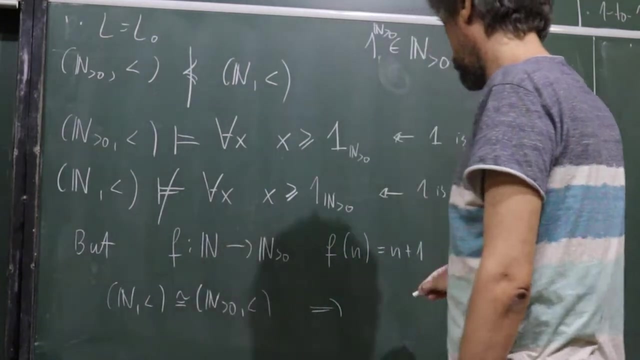 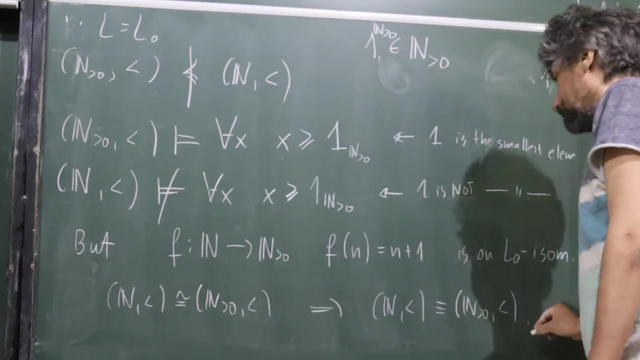 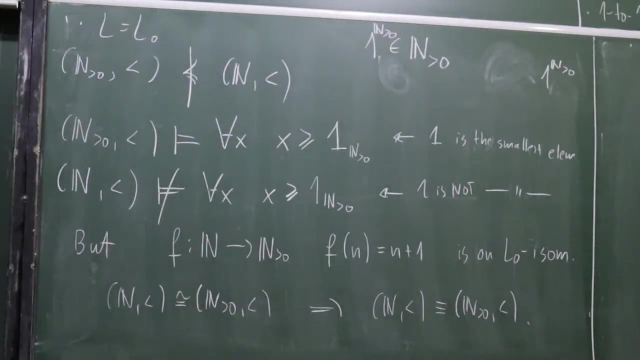 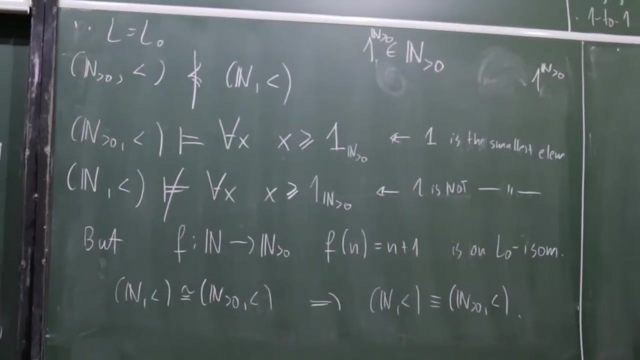 is, which you can guess, I guess, is an isomorphism. so in the particular, they are elementary equivalent. so they are even isomorphic, but not, it's not an elementary substructure. in particular, you have to use parameters to see it. ok, still, there is hope. so 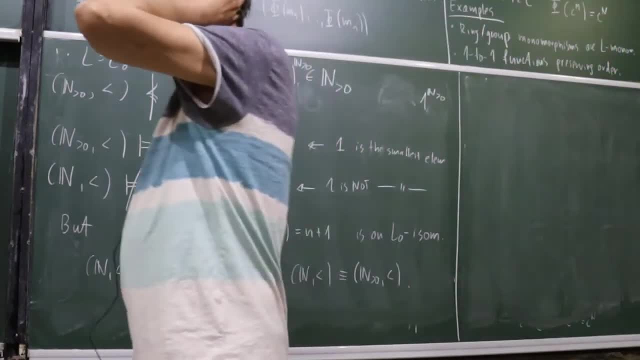 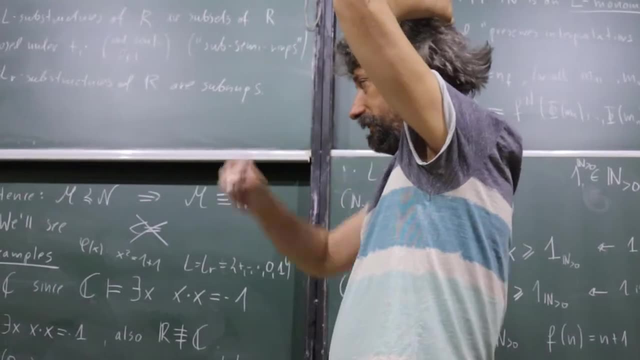 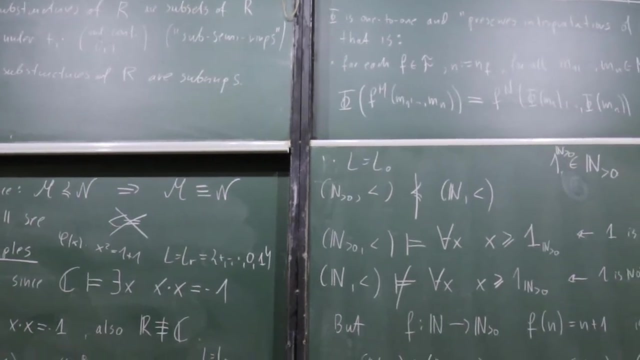 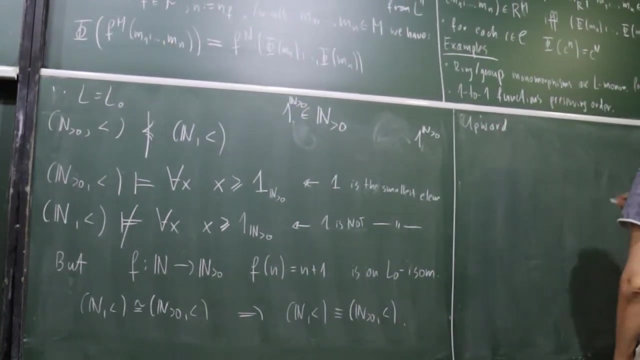 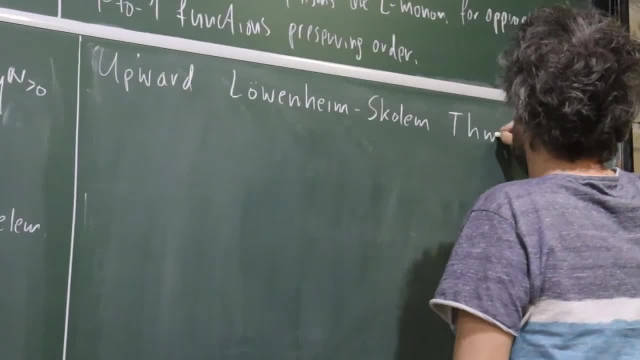 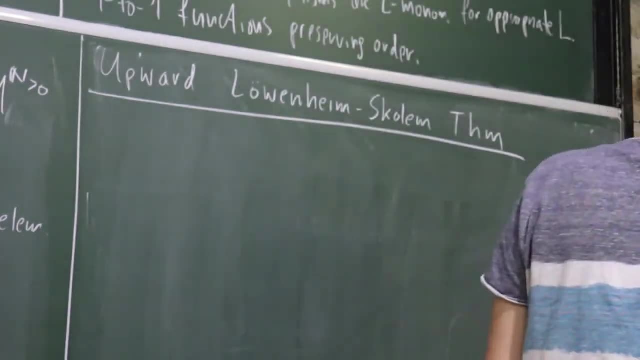 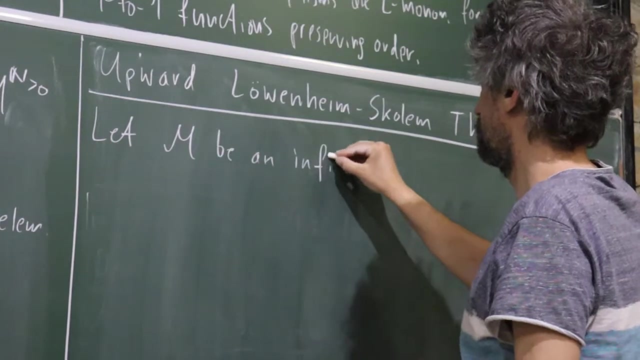 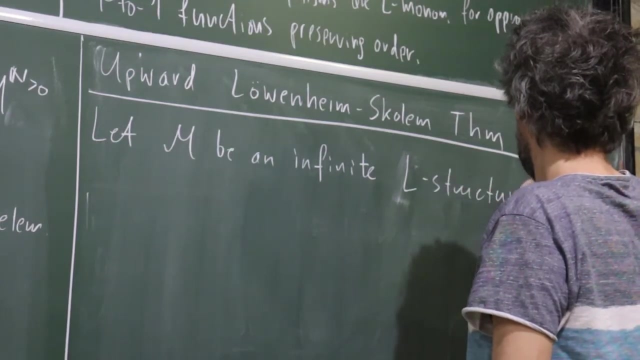 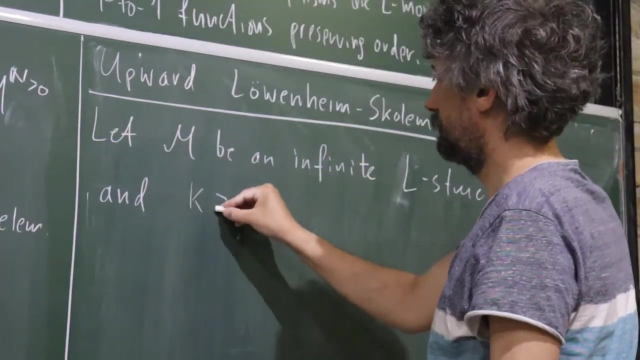 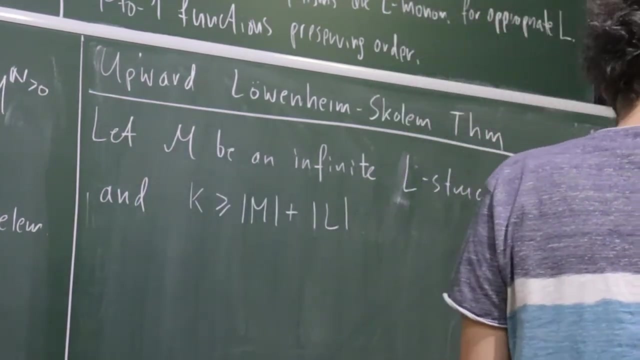 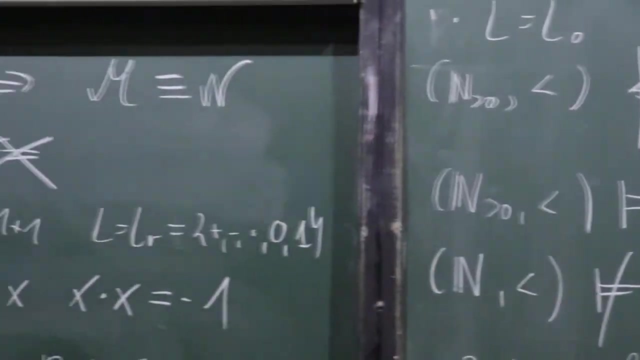 column theorem, column theorem, we will not need the downward one. what does it say? so that m is important, is infinite. and again, take any cardinal number, kappa, greater than cardinality plus cardinality of the language. so this is basically the cardinality of this language, l, extended by parameters from m, that's. 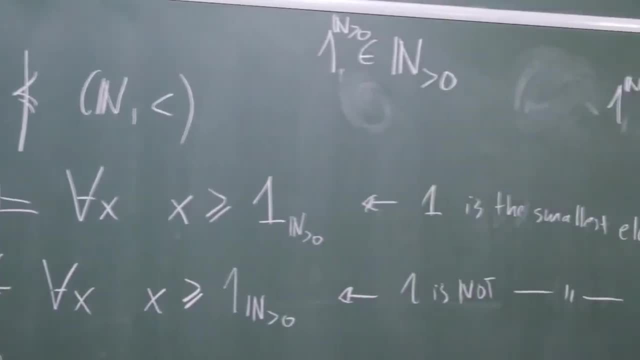 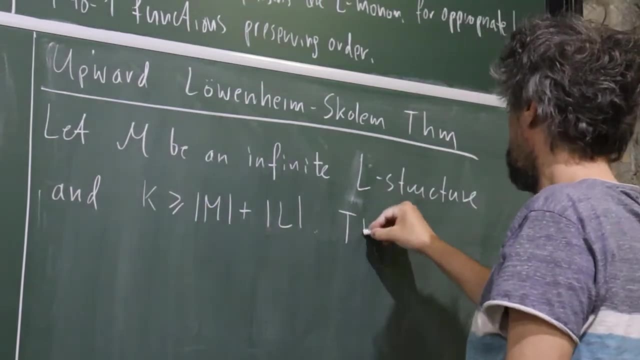 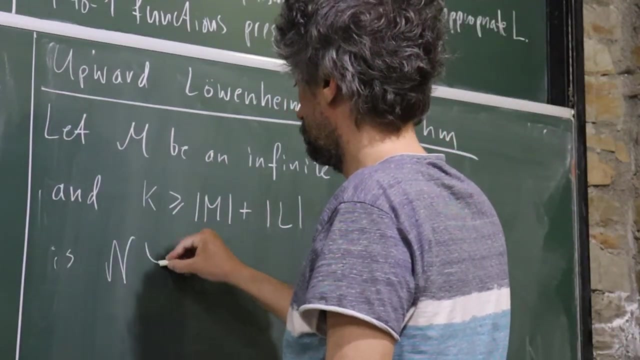 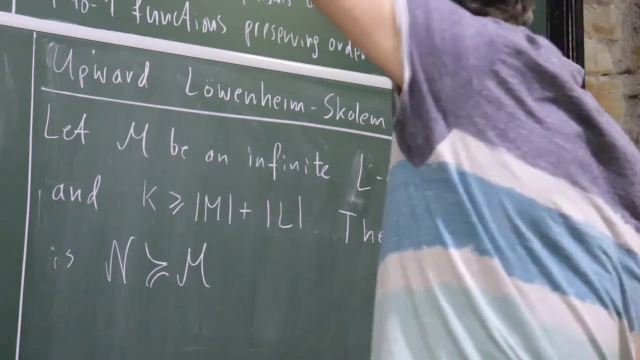 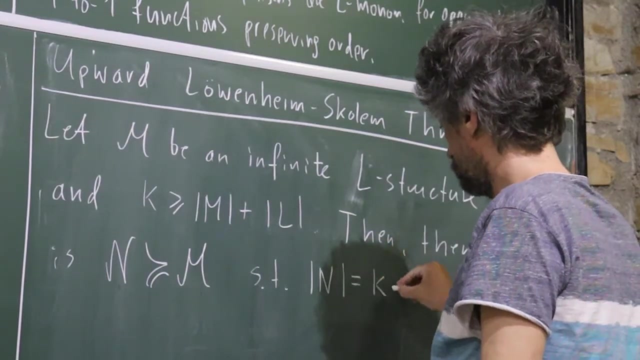 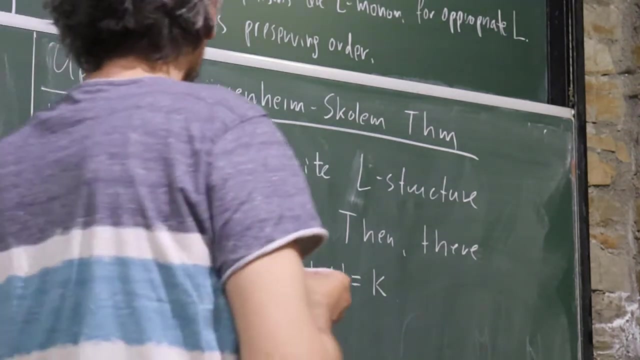 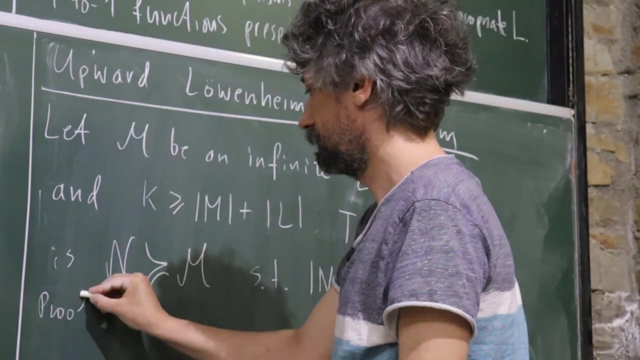 the meaning, then we always can find, like elementary superstructure of cardinality, kappa. so there is something bigger, something that m is elementary subtraction in n, such that, and using this we will show this model, theoretical theorem too, so so, and some properties of fields. so proof, arbitrary, just big enough. 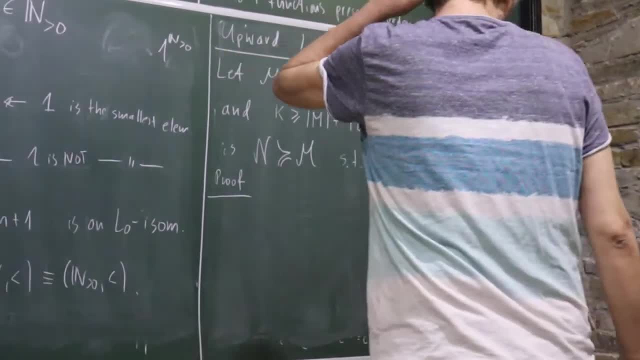 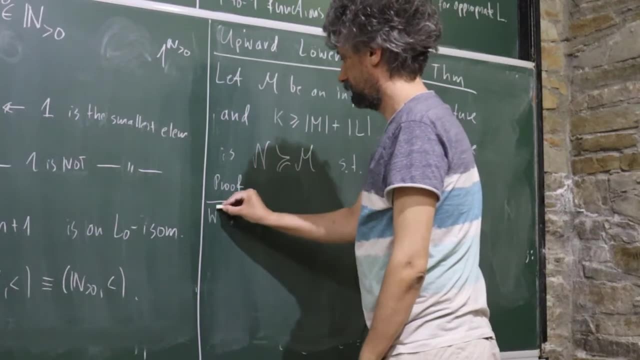 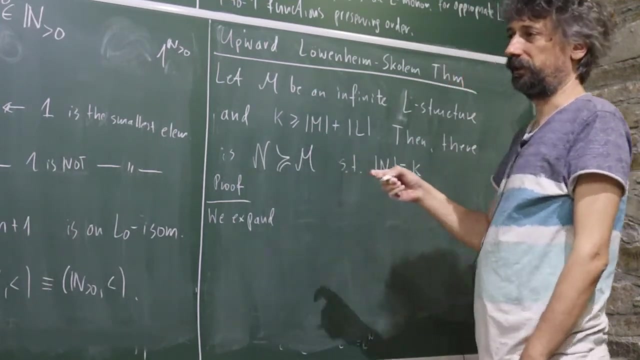 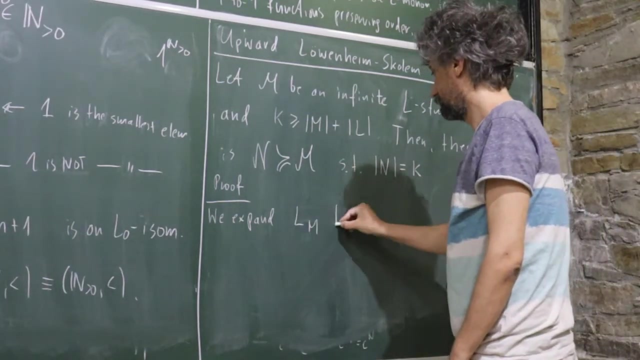 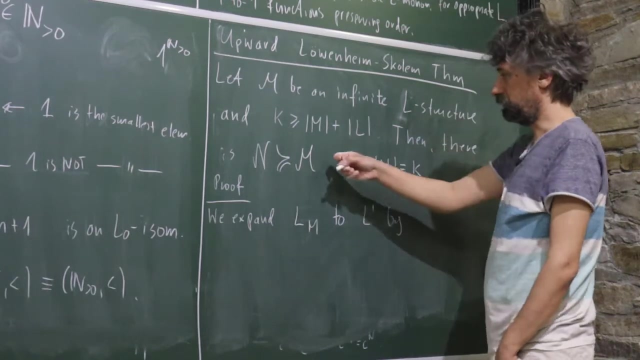 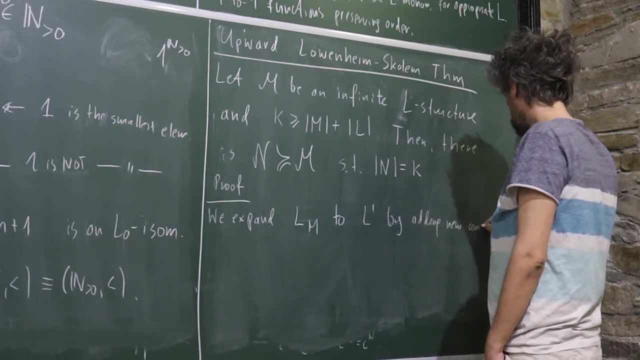 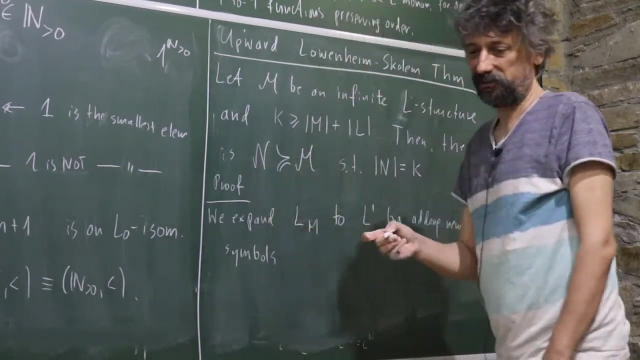 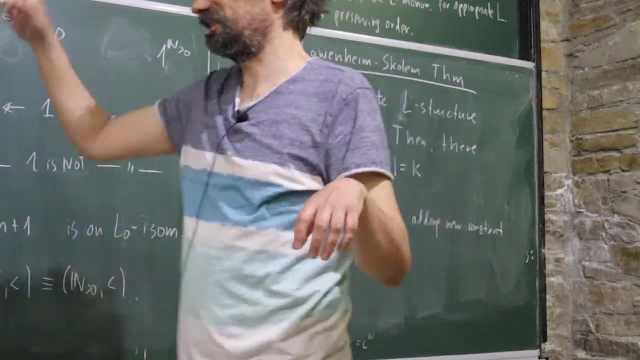 okay, so we work in some language even bigger, that language of l, l, expanded with constants from m to l prime by adding new kappa constant symbols. there's some constant symbols which were not already there, so l has its constant symbols are extra constant symbols for all elements of m and 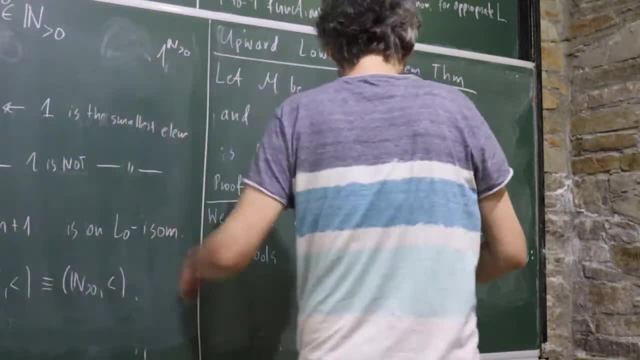 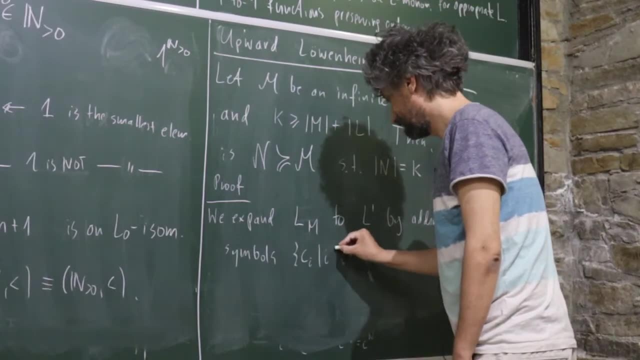 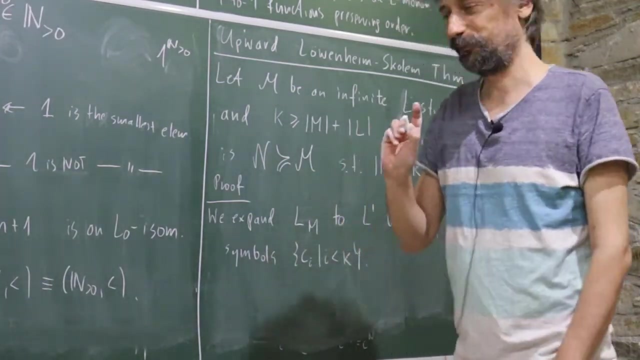 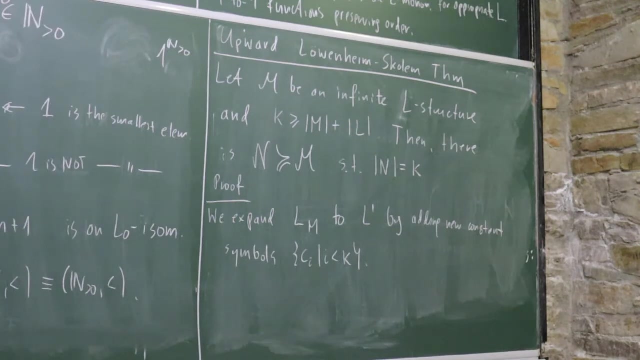 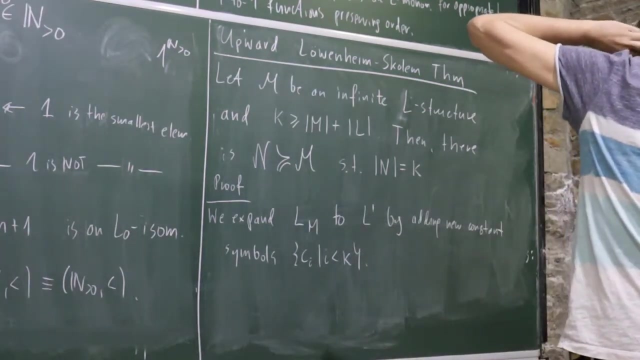 still, we are adding kappa new ones. we can do such things. so i think there are people who claim we cannot do such things, but there are not so many of them. why? why? why? because people believe only in finite sets and this is really, really infinite. 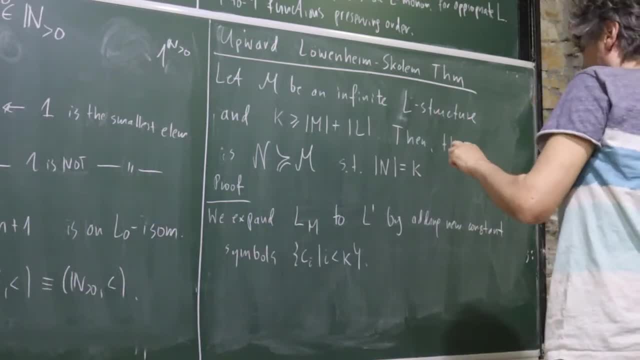 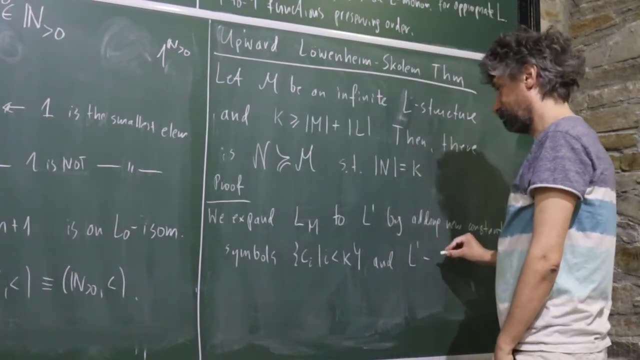 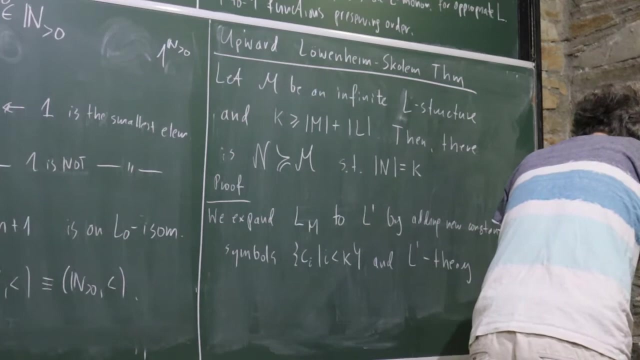 there's very finite number of such people. okay, so this is l prime and define. ok, and l prime, t t prime and to this theory will look like that. okay, let me check, let me take that back first. we will show this next time you go. this time move this, showing that this will hover. 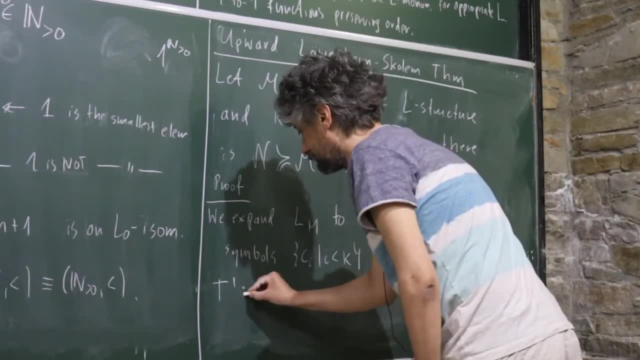 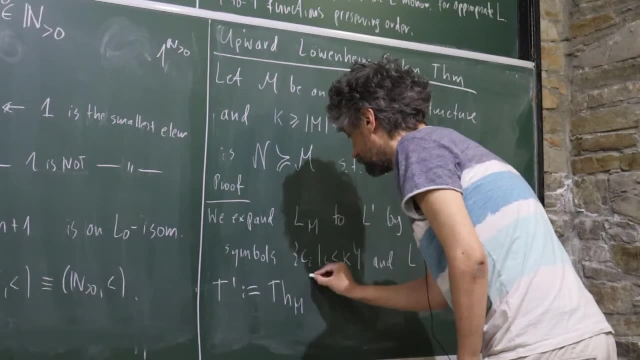 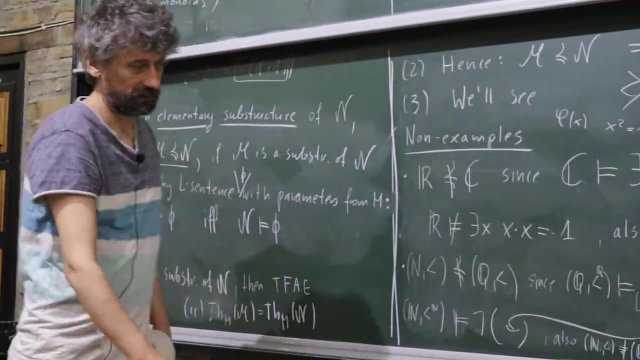 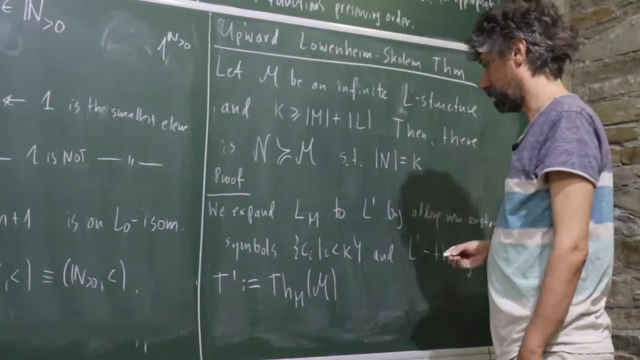 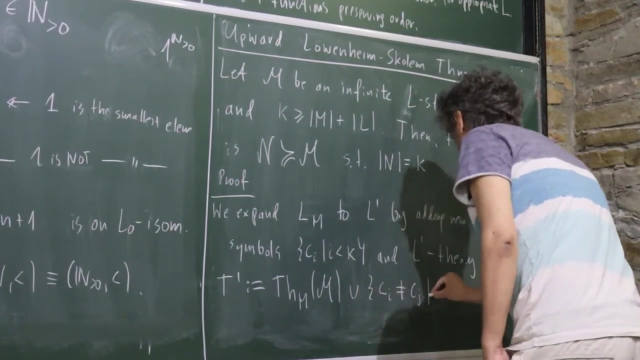 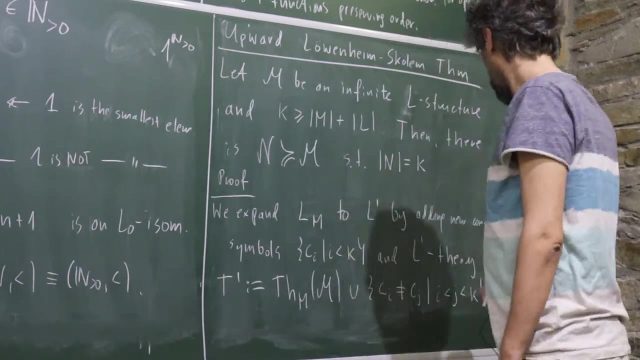 will apply compactness theorem and its model will be this: n. so this kind of full theory of m, even with constants from universe of m and saying all the constants are pairwise different. yes, so for all different pairs of indices smaller than kappa, this is still kappa theory, says interpretations of these. 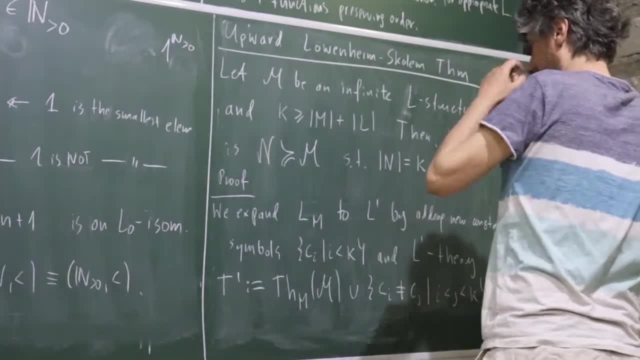 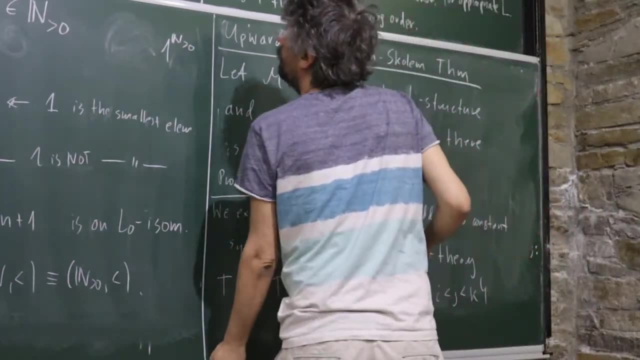 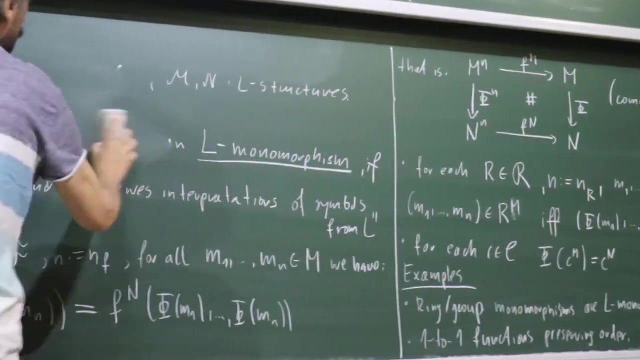 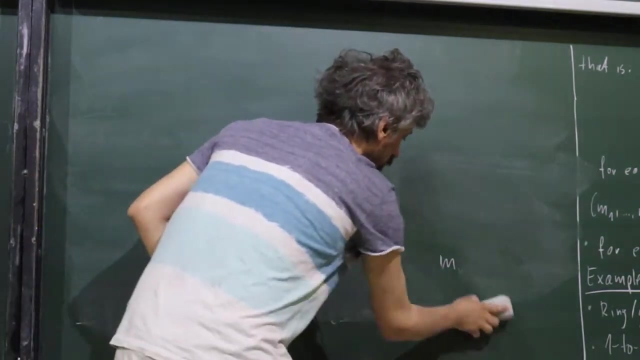 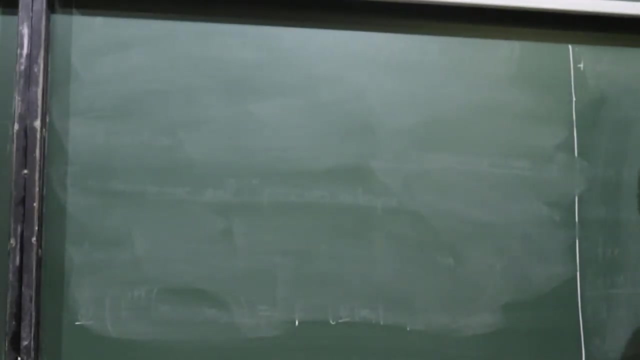 constants are different. okay, so now? okay, shall i? oh, it's not too hard, too technical, huh, i mean, if the proof is not too hard or too technical, maybe we can think the rest, the proof is not hard. yeah, i mean, we will just show that every finite. 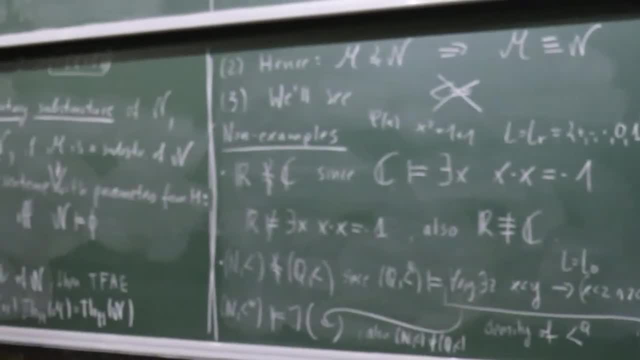 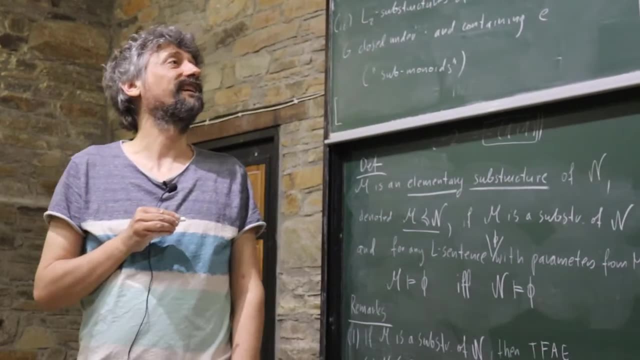 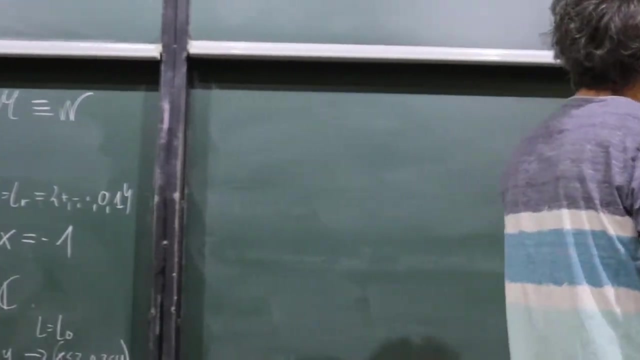 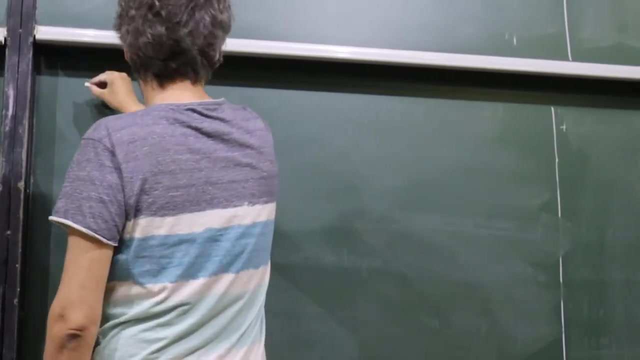 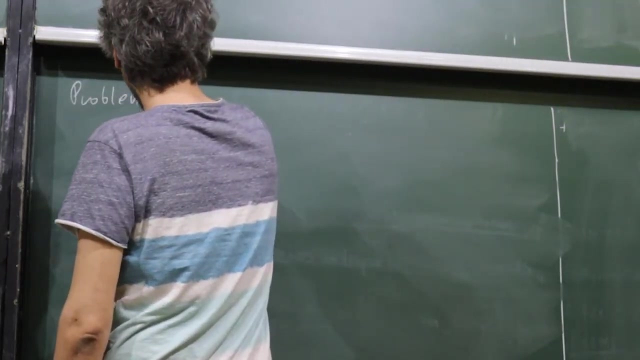 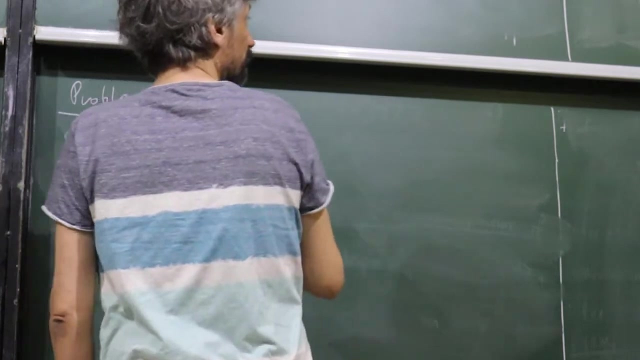 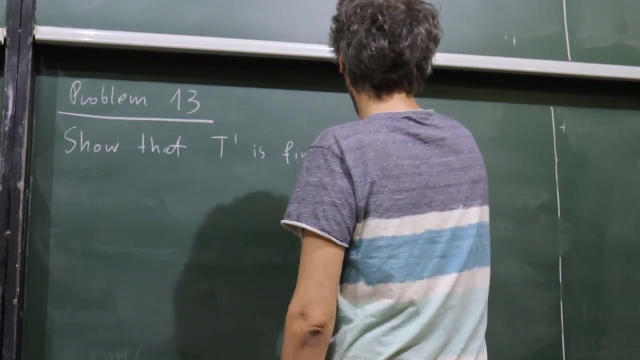 as a model, right, yes, yes, so. so you mean, without writing or what, maybe it might be a problem, i think the rest, ah, okay, there were enough. we could think: okay then, so, huh, okay, then, problem, okay, uh, thank you, how did a бог? the problem is finally. 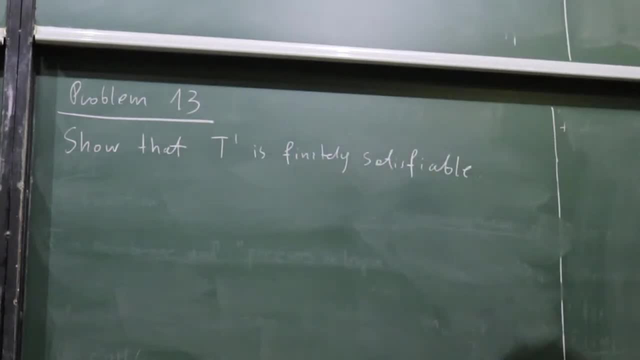 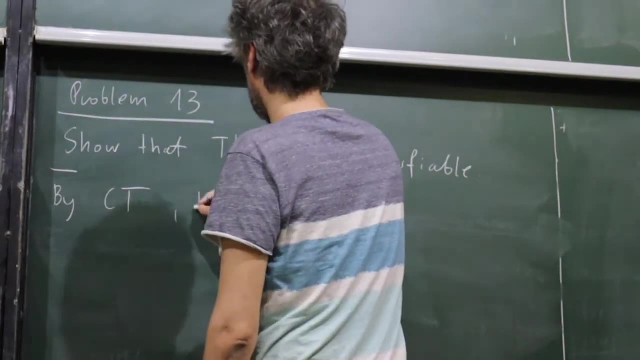 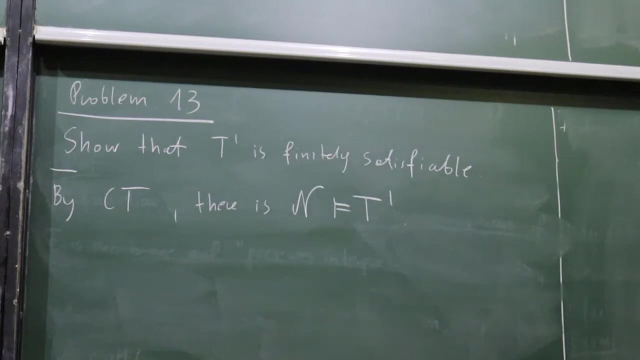 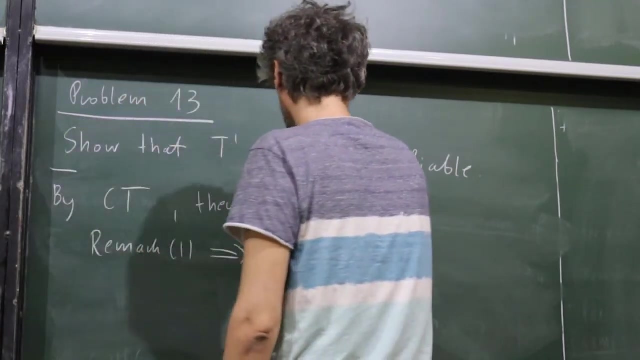 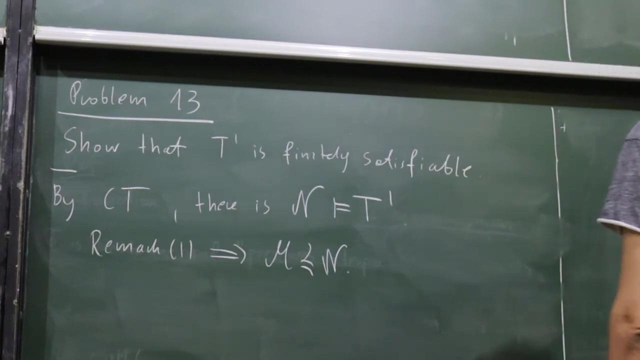 the problem is thin making it thinner, and thin and thin making it thinner. So now, by compactness theorem, there is a model of T prime and problem 13. So then, by this, by remark, not only that there is a model of T prime, but still this: 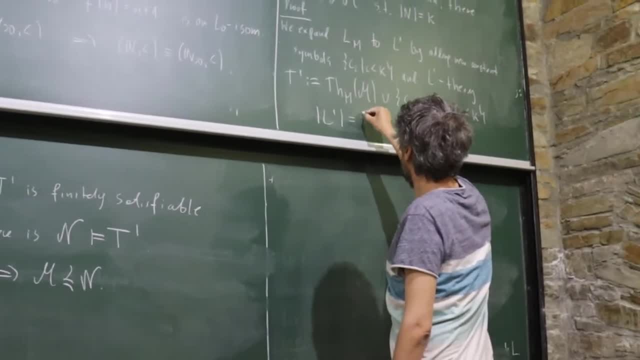 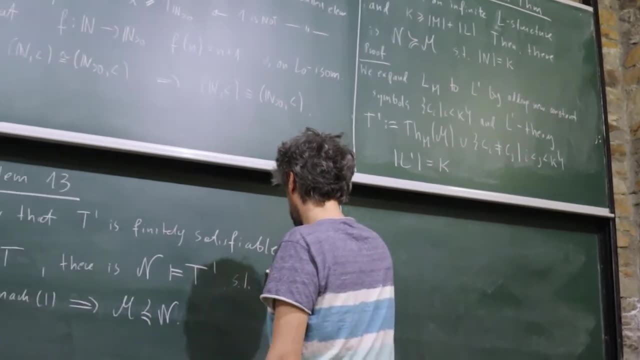 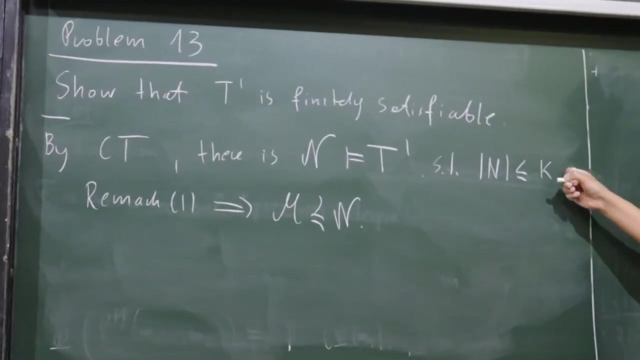 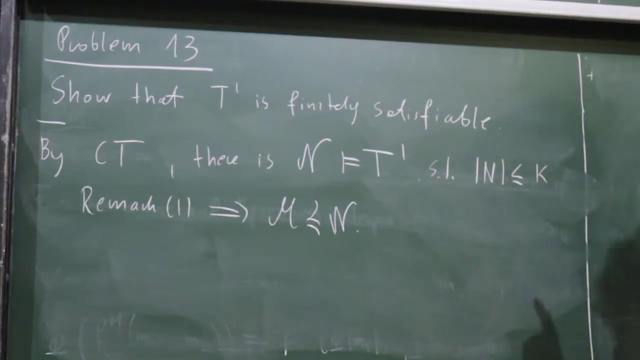 T prime, the L prime. now the cardinality is exactly kappa and by compactness theorem there is a model such that kappa. So this is the moment- actually this is a bit important. this is the moment when I need this bound from compactness theorem to get the model of exactly cardinality, kappa, okay. 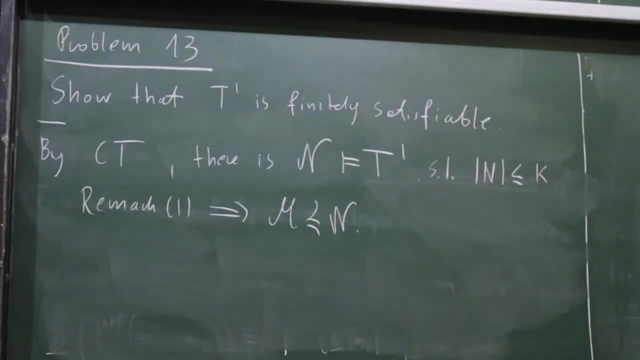 so this I don't want to skip. this was kind of because you could think: why did I care about it? so this is a moment. I cared about the bound, which will be important later. It's also smaller than the bound, It's also, yes, but now we see okay. 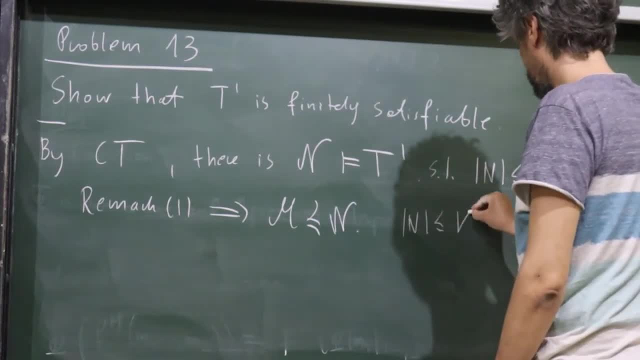 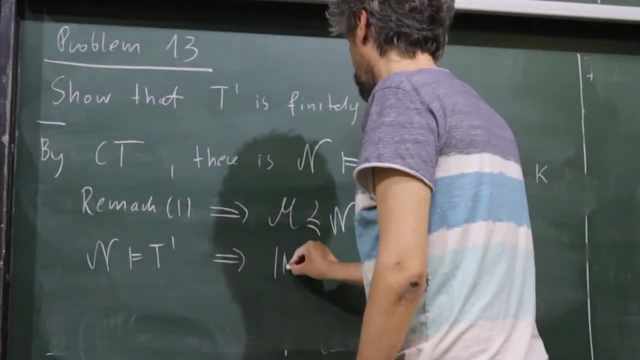 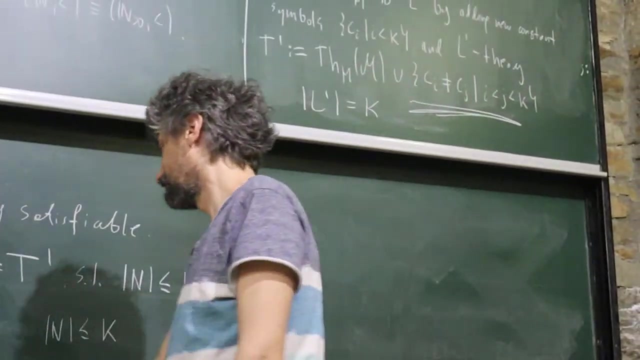 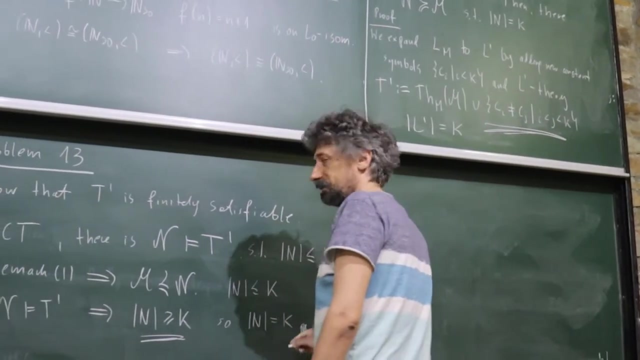 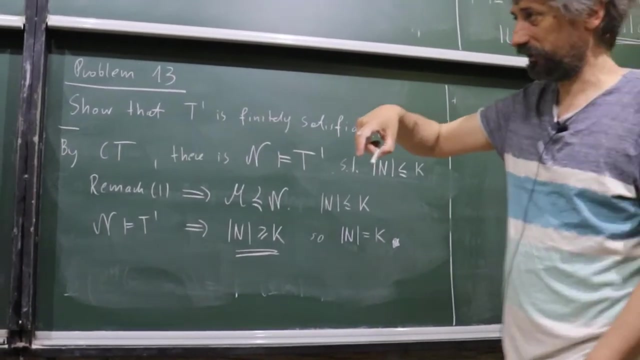 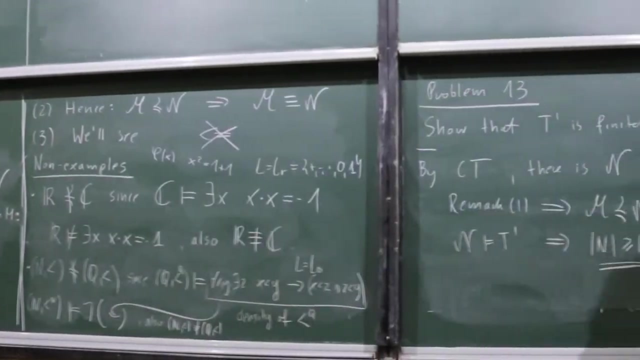 So here we have that this is smaller than kappa, but since n, then it's also at least kappa, of course, by this. so it's exactly kappa. That was the port, okay, So compactness theorem gives us many, many, maybe not sub structures yet, but like elementary extensions of arbitrary. and now 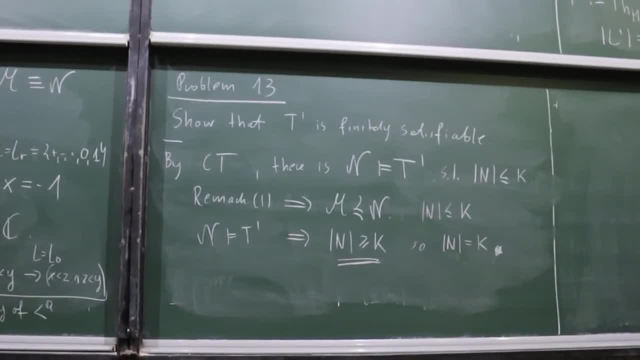 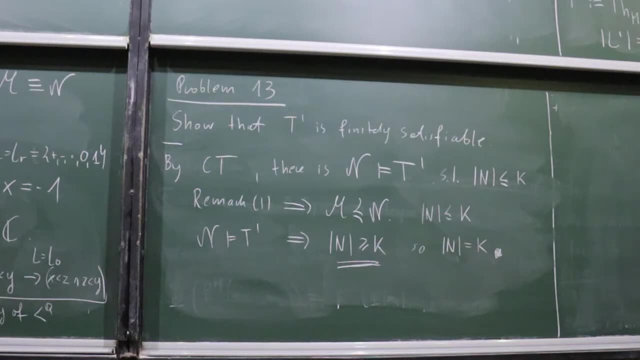 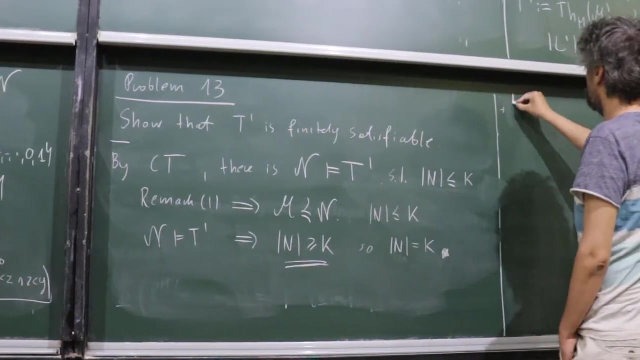 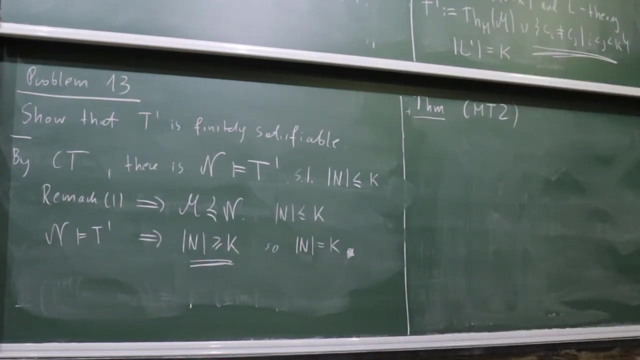 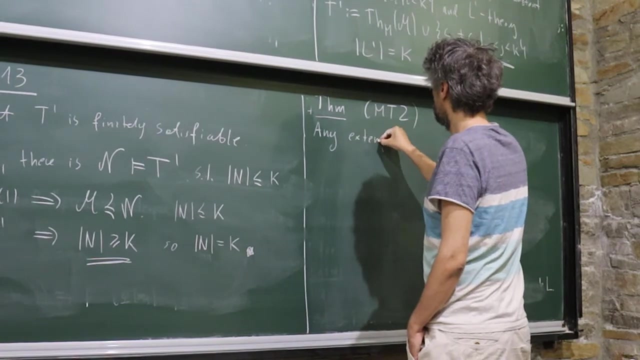 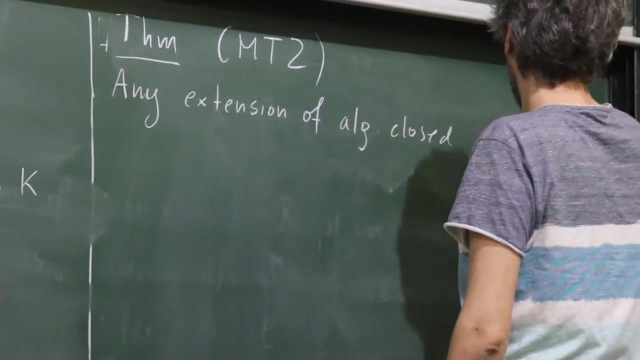 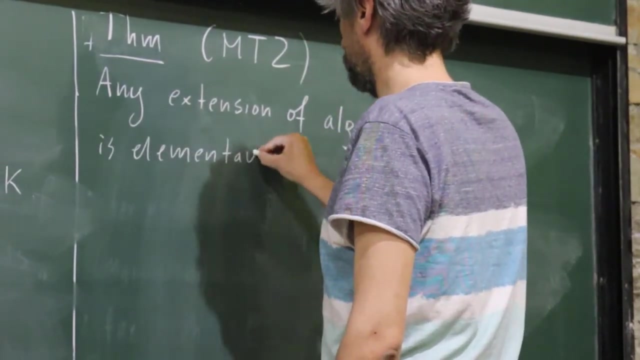 I may show- okay, the time I may start at least. so using this, I may show this theorem which was called mt2. this was crucial for Hilbert-Nolstein, that's. so any extension of algebraically closed fields is elementary, so this will be something concrete. 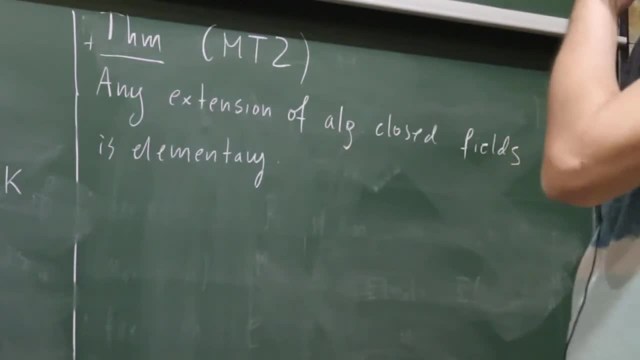 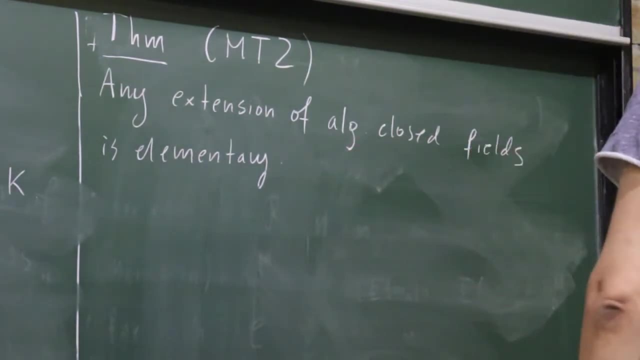 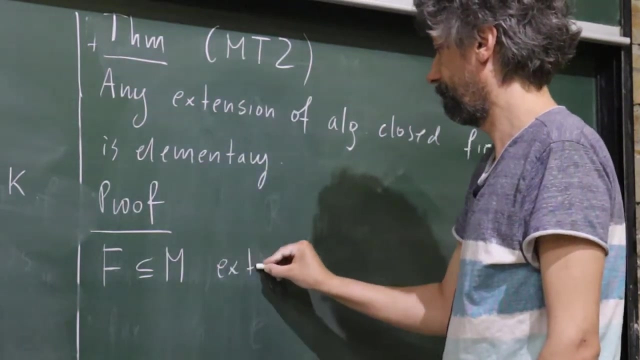 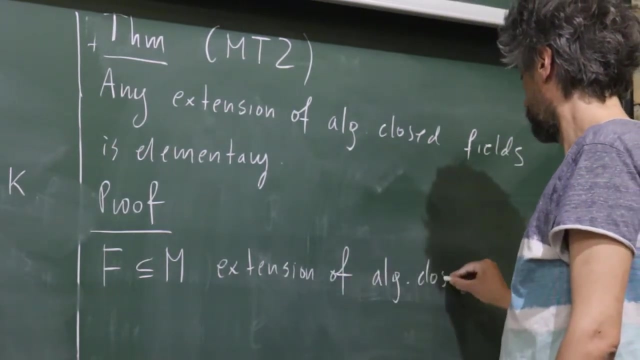 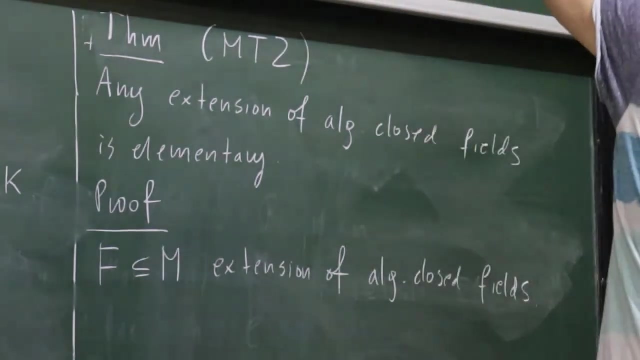 first real example that such things happen. okay, this was needed for Hilbert-Nolstein and that's, but it takes a bit more time that I have left, so let me start. so let fn: extension of algebraically closed fields. so what is the trick? now we take kappa. okay, now, of course, I don't distinguish. 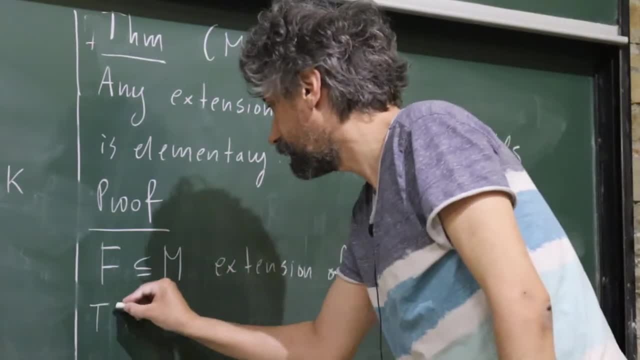 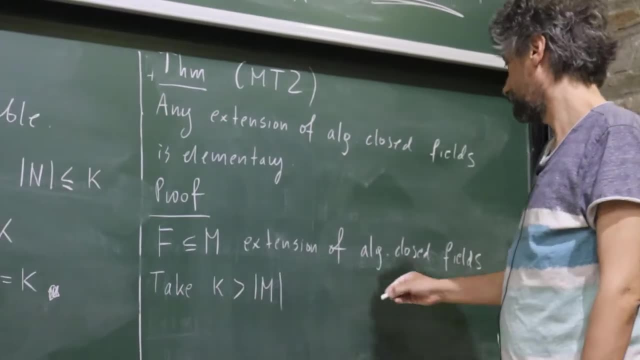 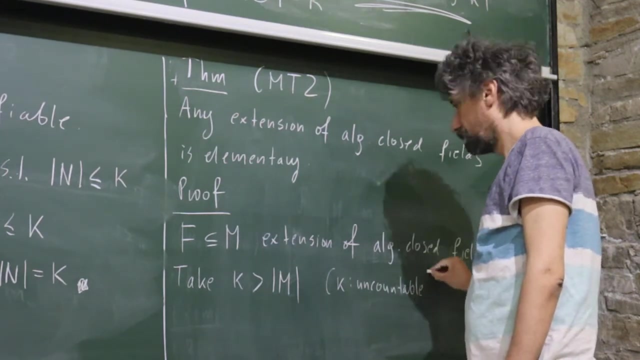 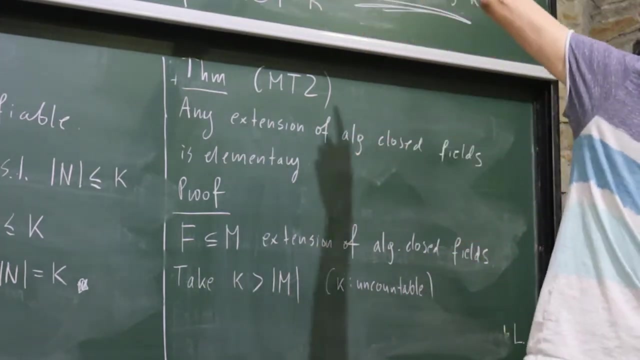 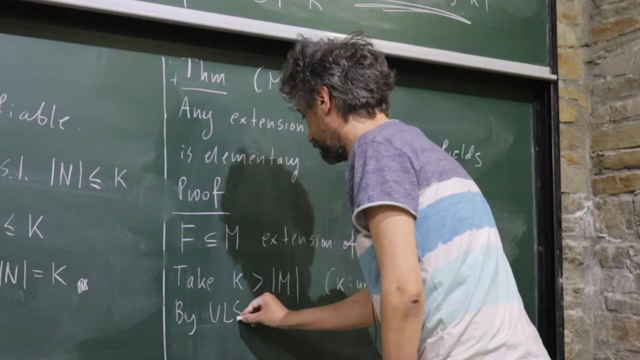 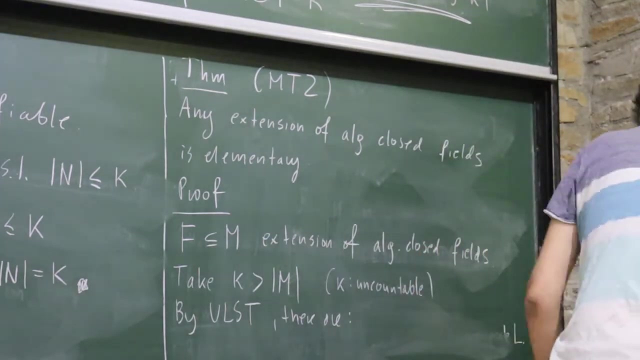 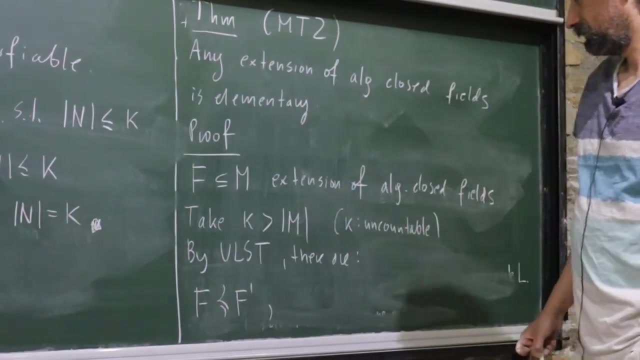 between universe and field. so take kappa, greater than this, in particular, kappa must be uncountable because algebraically closed fields are infinite and we apply upward lovenheim's color theorem. there are extensions here, elementary, so lmr, elementary extensions in language of rings of fields. 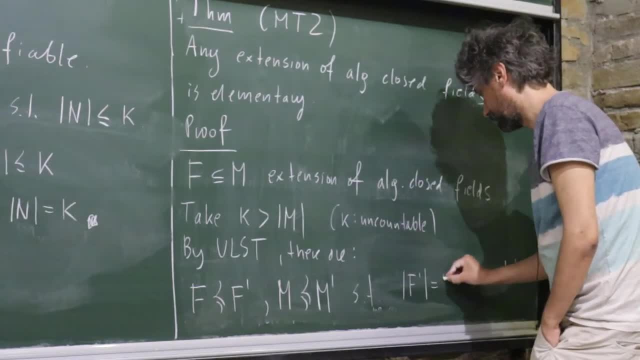 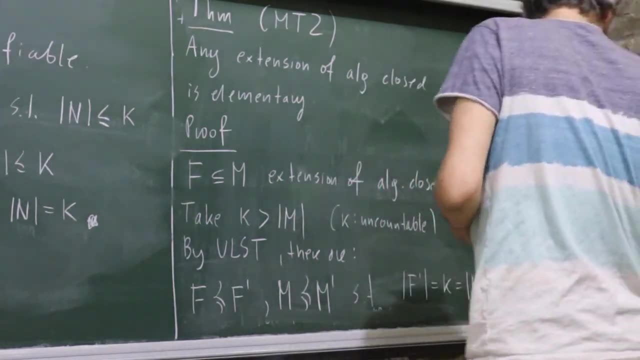 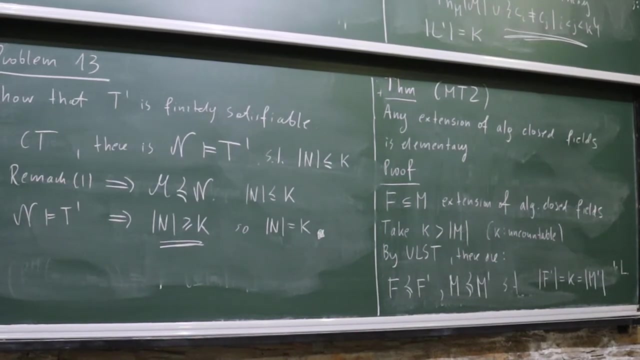 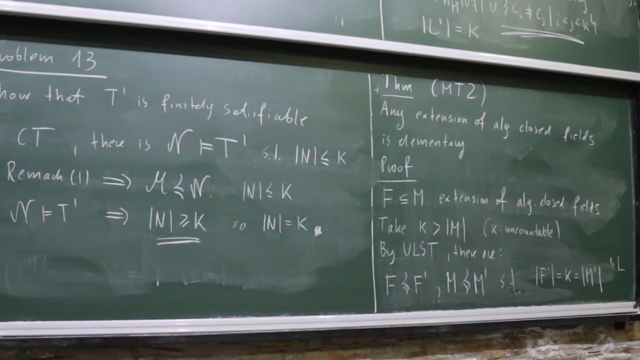 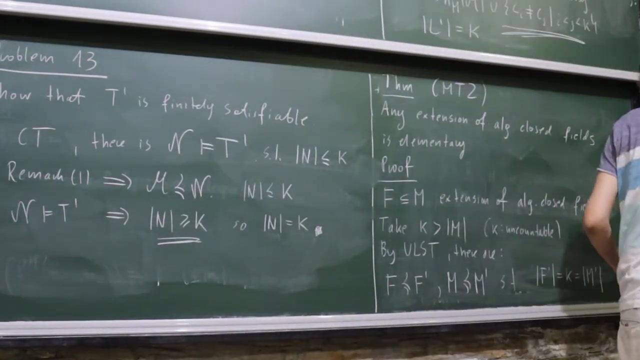 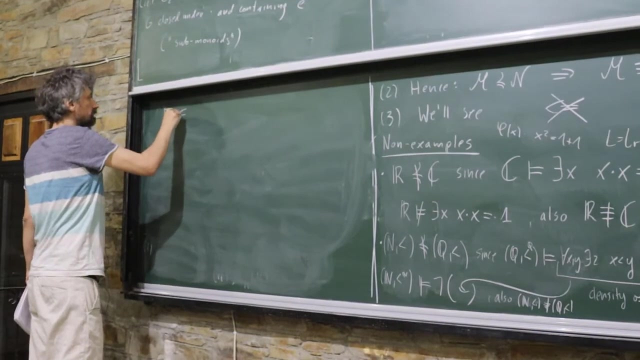 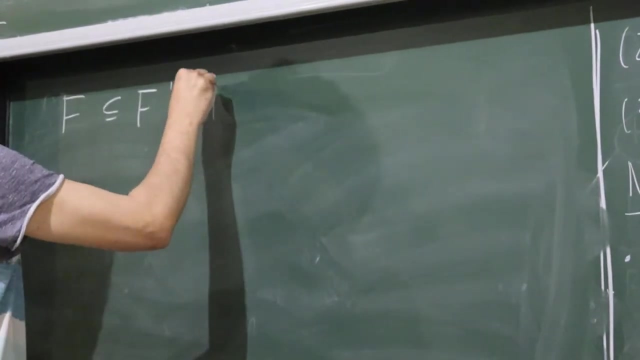 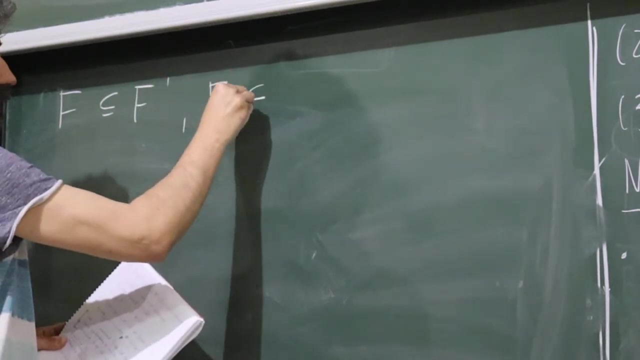 such that they are all of cardinality kappa, so so, so, so, so, so, so, okay, but now there is a moment, so so these are such extensions, okay, but now there is a moment. so these are such extensions, so these are such extensions. so in particular, we have such extensions. 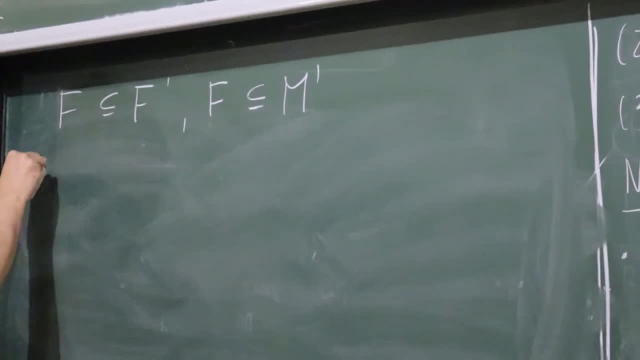 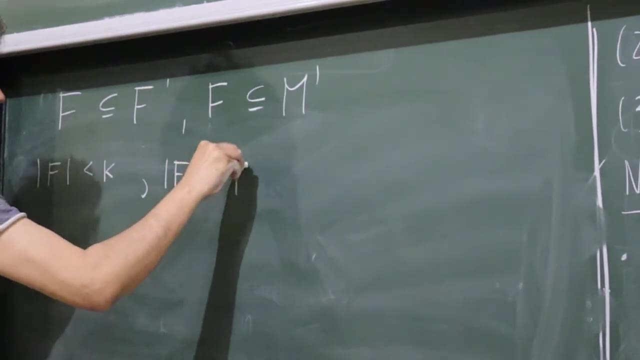 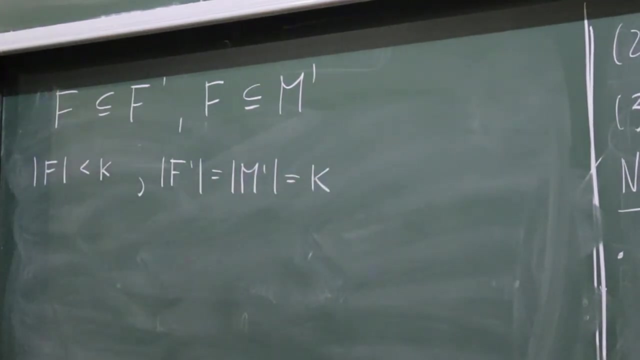 and cardinality of f is smaller than kappa. and now, okay, now it's a moment. how much do you know from fields? so we have such extensions? and now, okay, now it's a moment. how much do you know from fields? and now, okay, now it's a moment. how much do you know from fields? 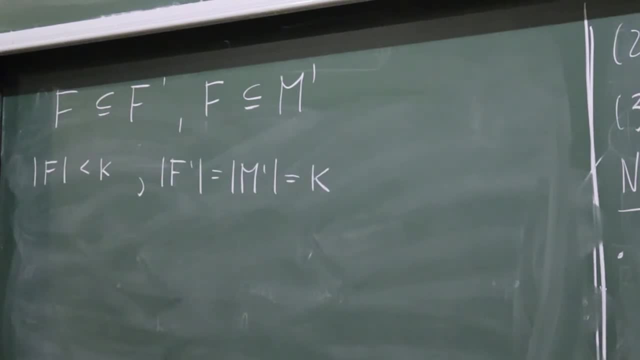 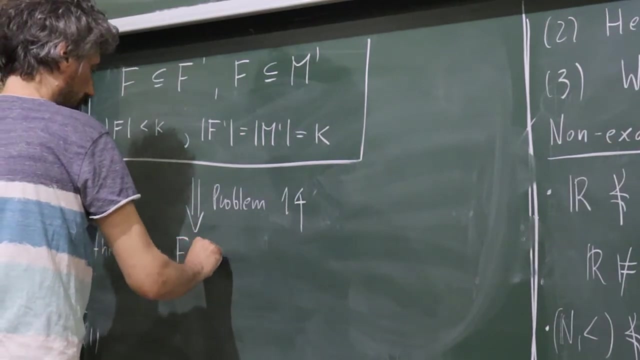 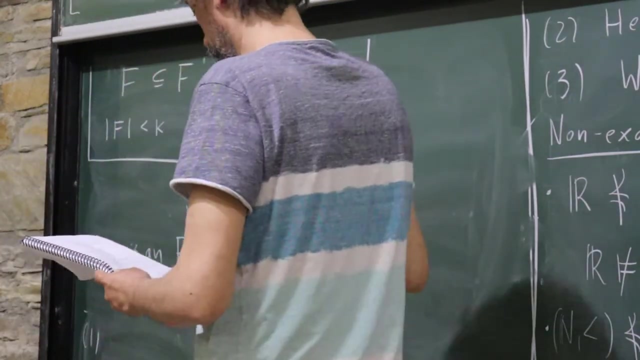 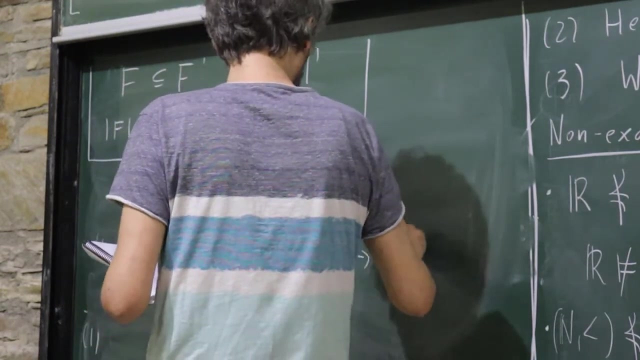 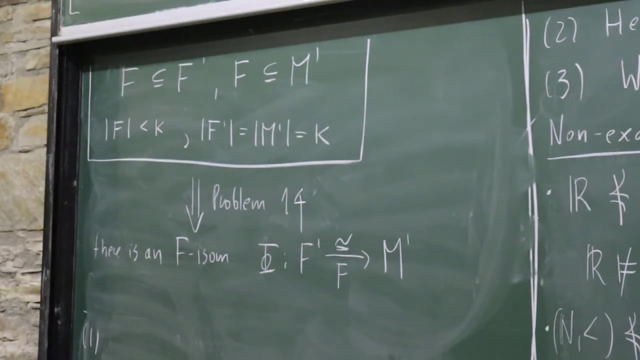 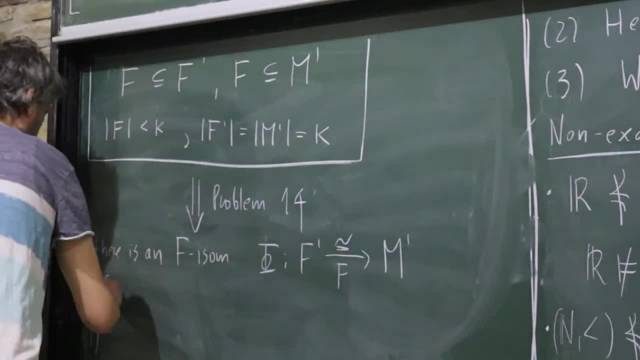 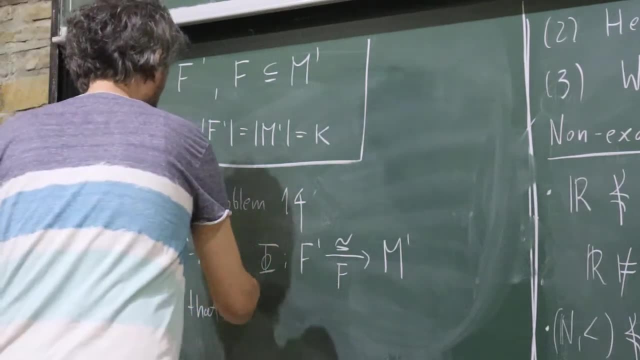 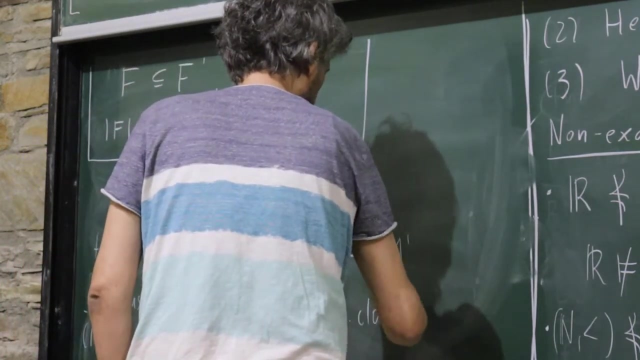 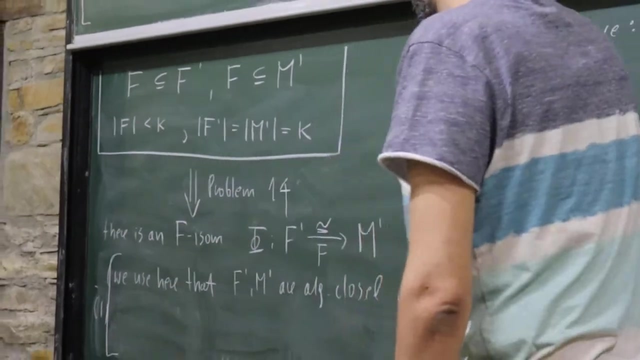 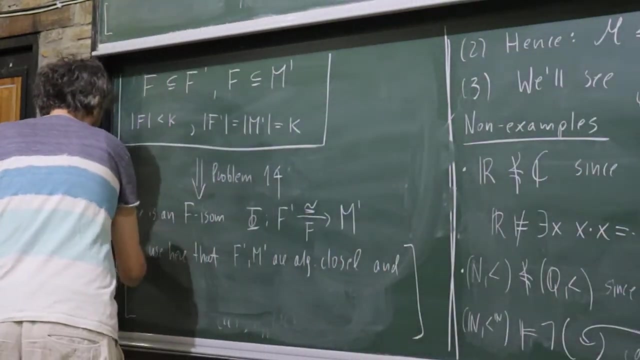 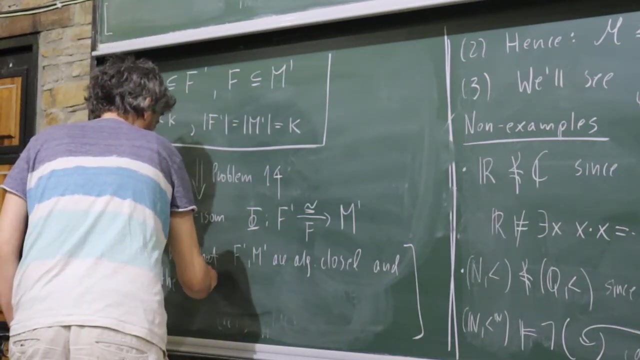 okay, so we use that f prime and prime are algebraically closed and okay, so i'm giving here a kind of hint plus what kind of things you have to know from field theory, from field theory, and that's the and that's the transcendence degree, transcendence degree. 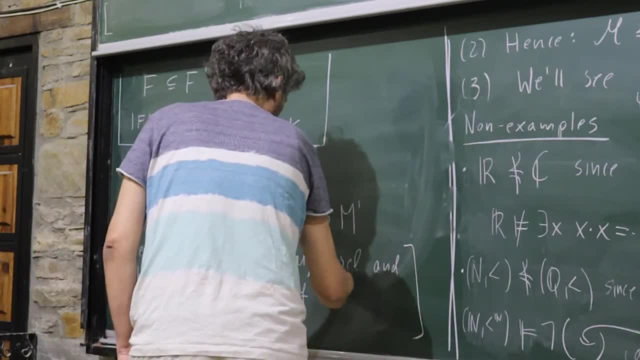 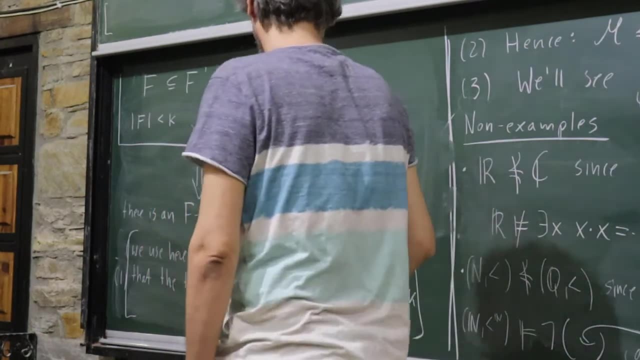 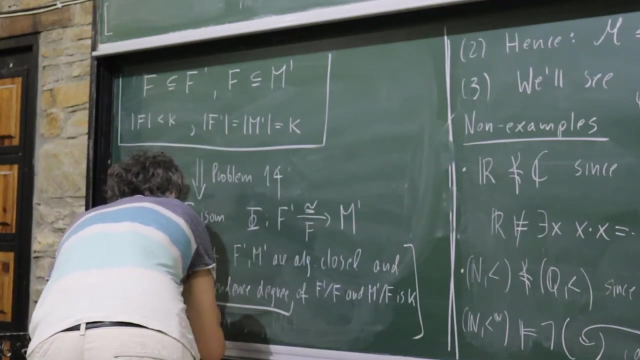 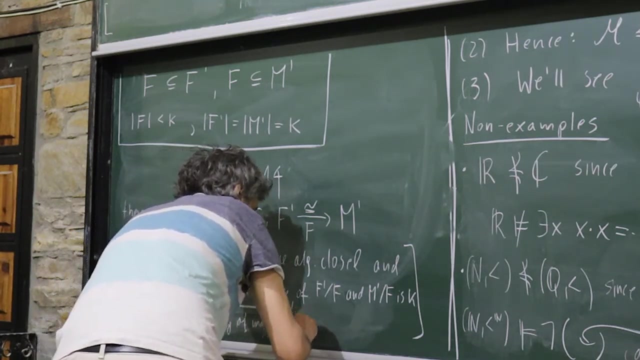 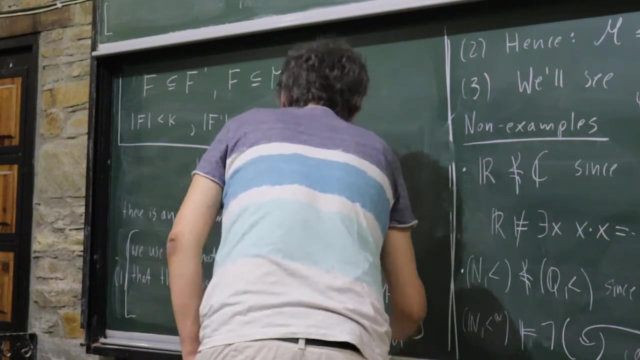 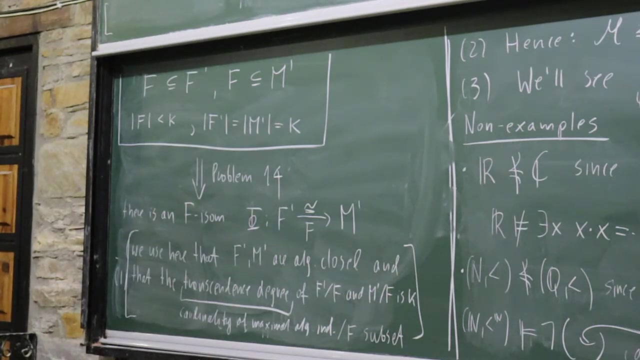 of must be kappa in this case, and transcendence degree, and transcendence degree of maximal and brightly independent over F subset. So did it appear in your life. We can discuss it in problem session, So that you should. So still, there is something, okay. 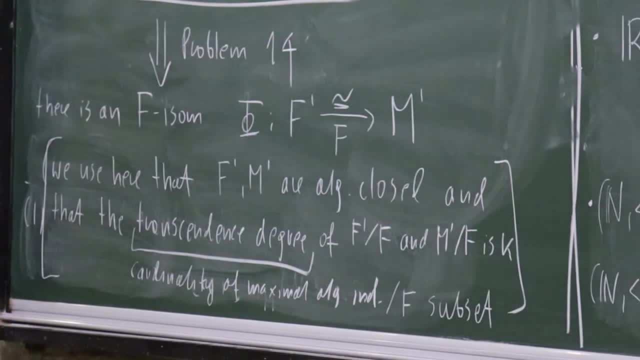 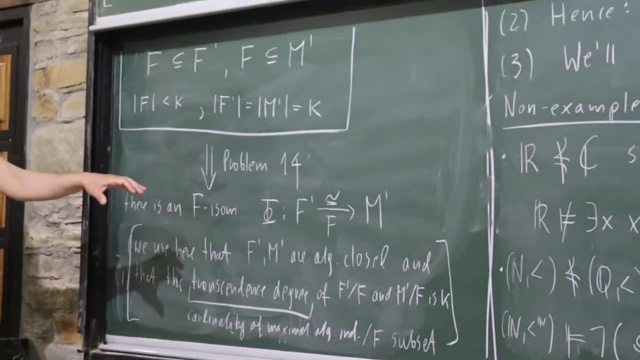 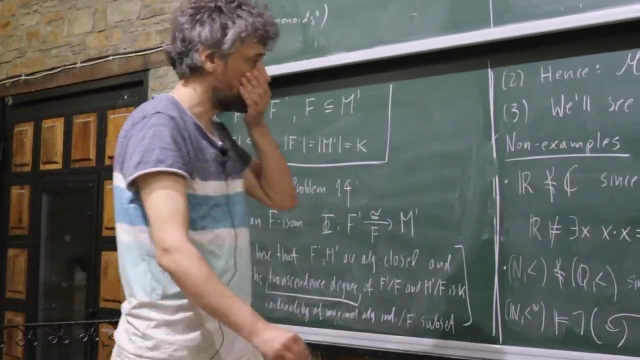 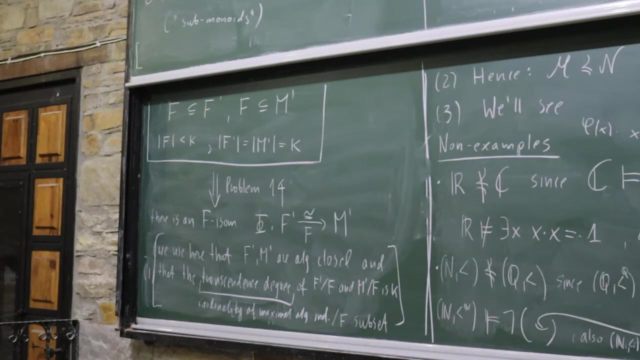 So I'm saying it's kind of obvious that by the assumptions, transcendence degree is the same kappa, and knowing that you should conclude that then there must be isomorphic over this field, F Okay, And then if we know that, Okay. 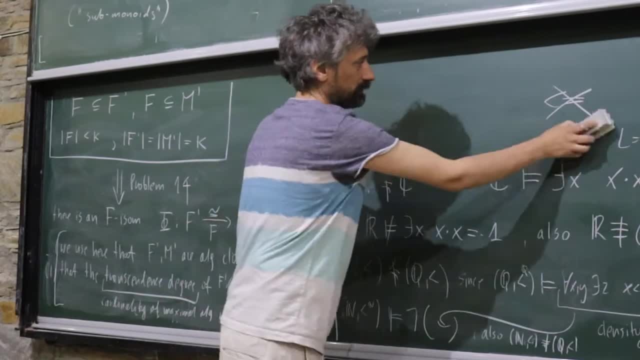 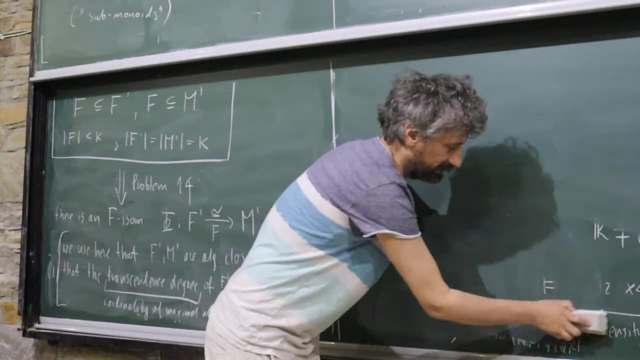 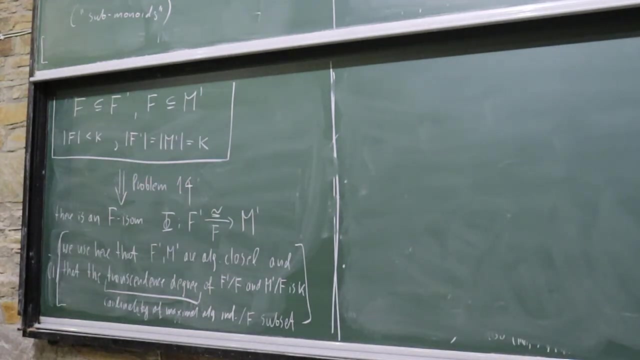 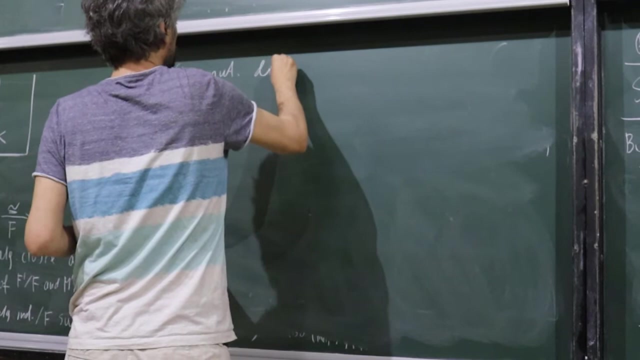 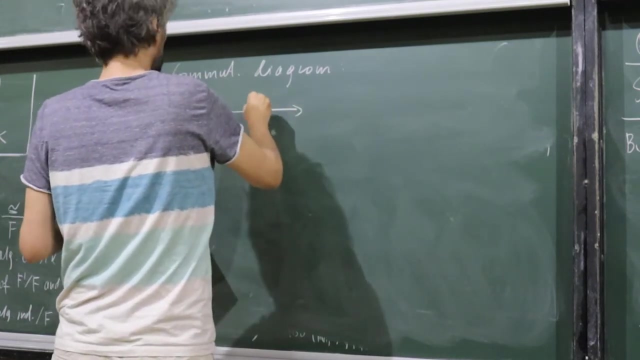 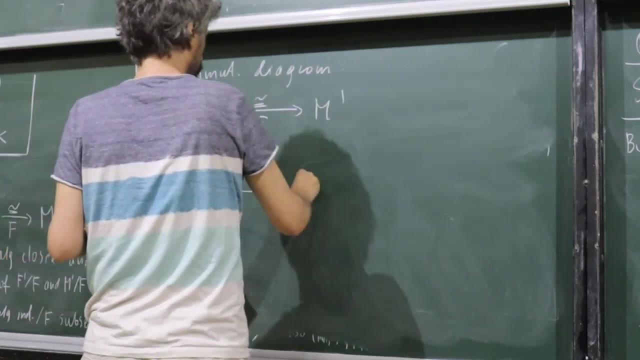 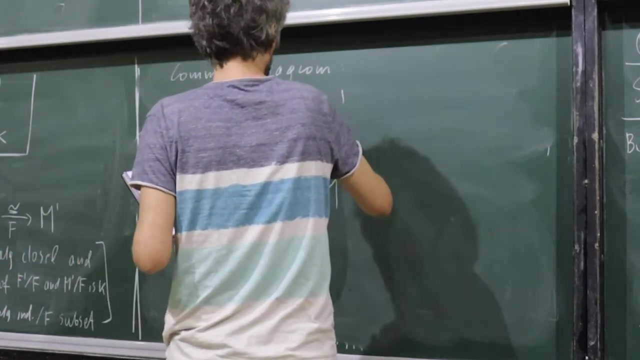 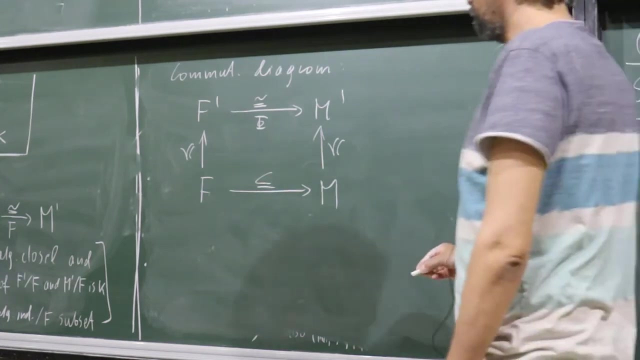 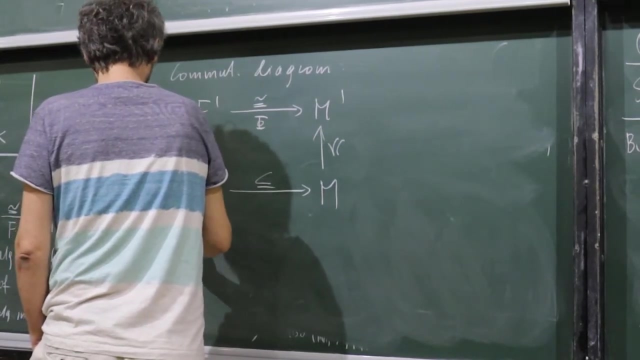 So I will just give a sketch and finish and come back to this next Thursday Because this is actually something quite interesting. What's going on here? So we have commutative diagram And, using this, if you have a VLR sentence, 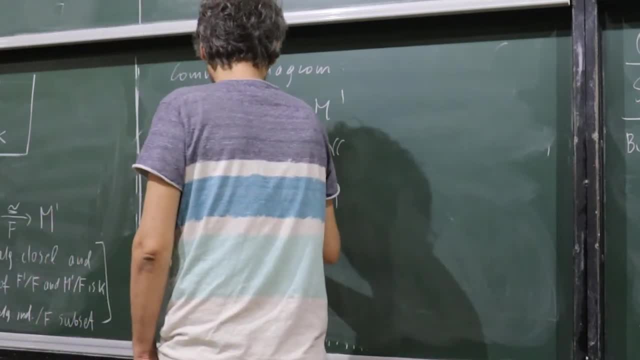 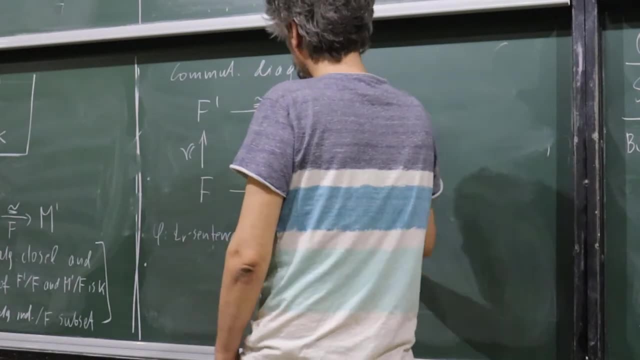 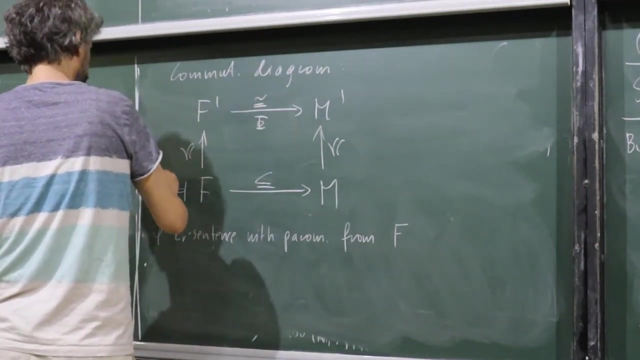 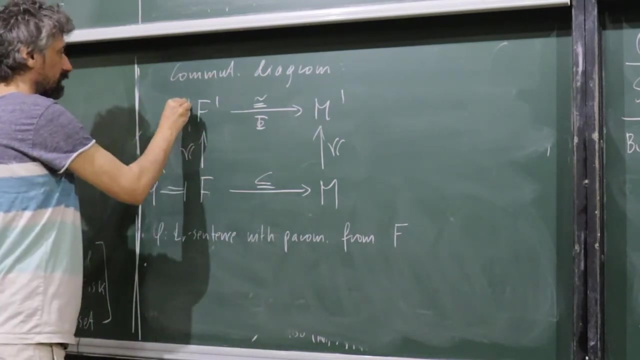 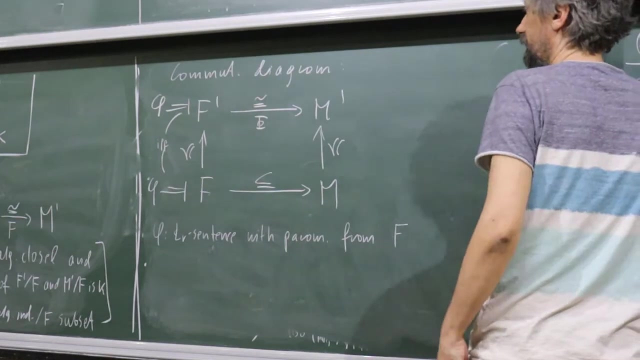 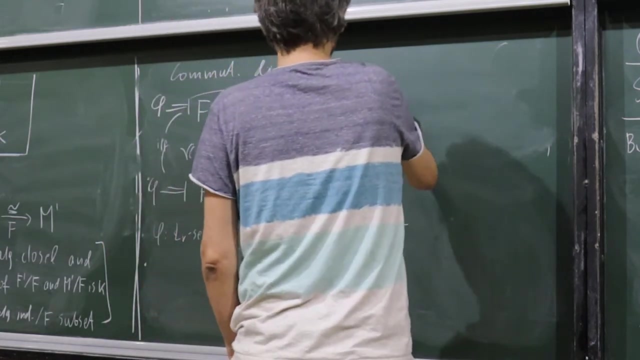 this of parameters from F, then you can just go around this diagram. So it is true here. If and only if. just by definition it is true here. But then, since also psi preserves parameter from F, it's if and only if. it is true here. 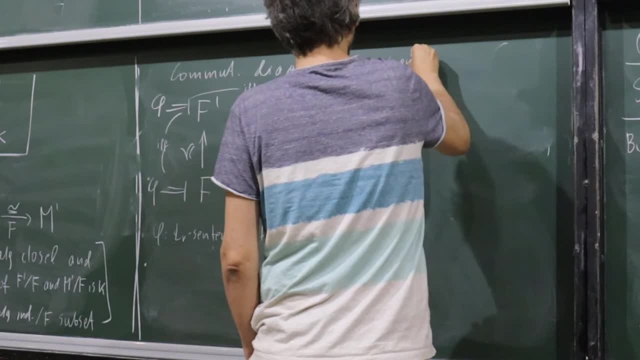 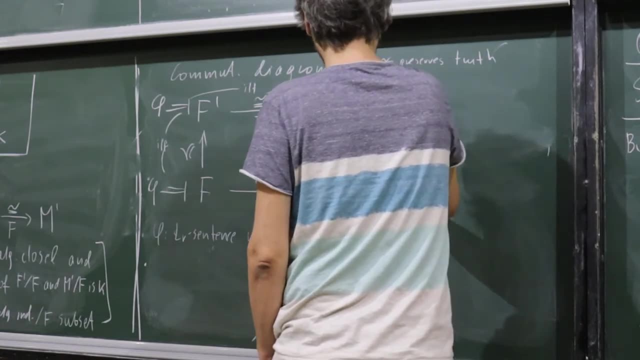 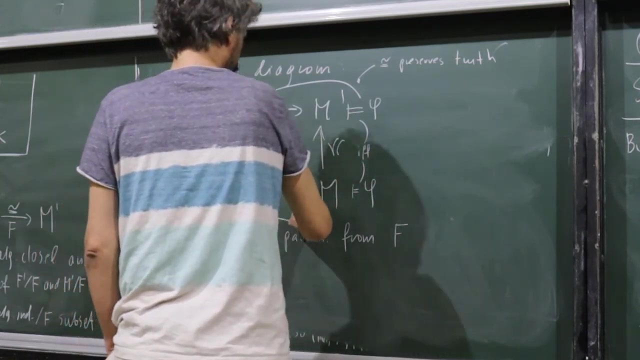 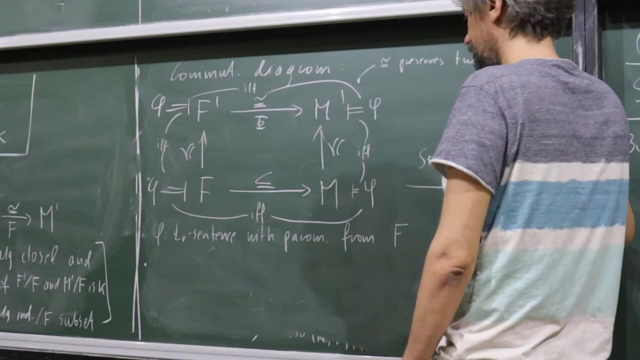 So this is, this isomorphism preserves the truth. And then again: So we get: this is true here, If, and only if, it is true here. So Okay, I will repeat it a bit next time, because it was too quick. 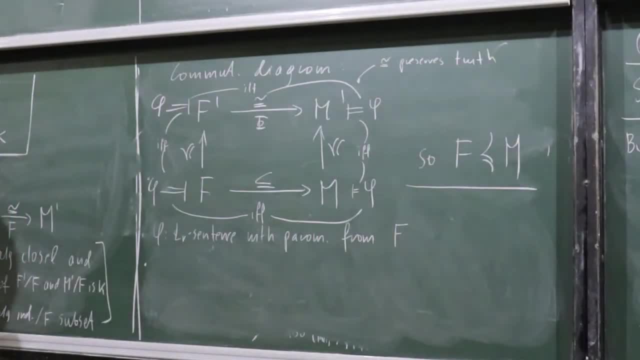 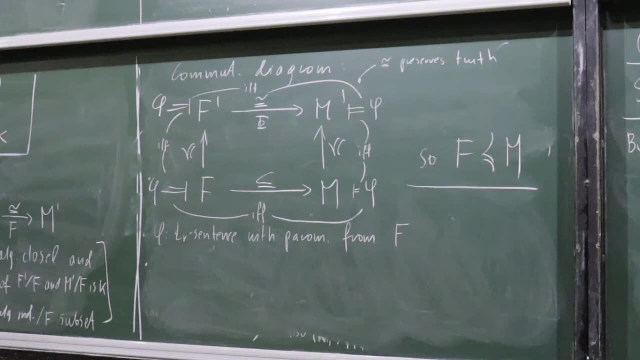 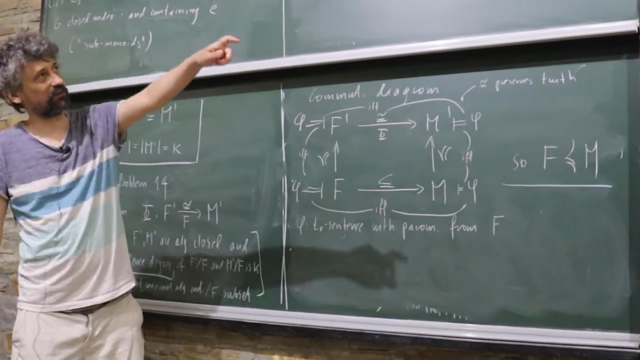 Okay, And then comment a bit more, But this is so, Okay, Okay, Sorry, But you can see that really the crucial thing was, Crucial thing in fact, was compactness theorem. Thanks to it, we get this Loewenheis column to find such things.